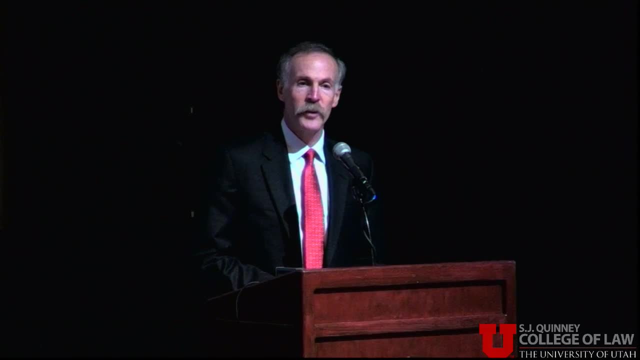 the time and effort and stewardship he's shown towards the Stegner Center these many years. Little need be said, really, about the appropriateness of the topic of this year's symposium: air quality, an issue that affects us all quite deeply, not just internationally. 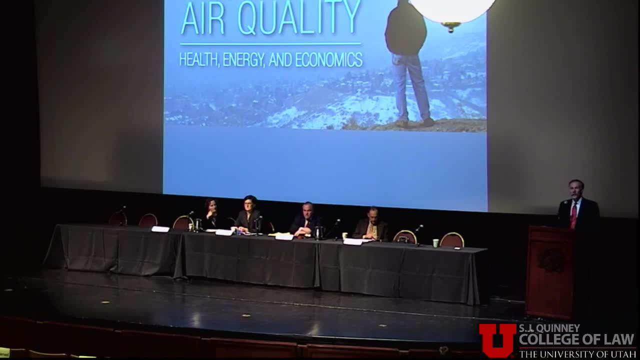 as we heard yesterday from Professor Percival, and nationally, but locally and regionally, as we have seen in the past, And I want to acknowledge the panel that has been here today for the process of organizing this forum. We've had a great discussion about air quality challenges on the 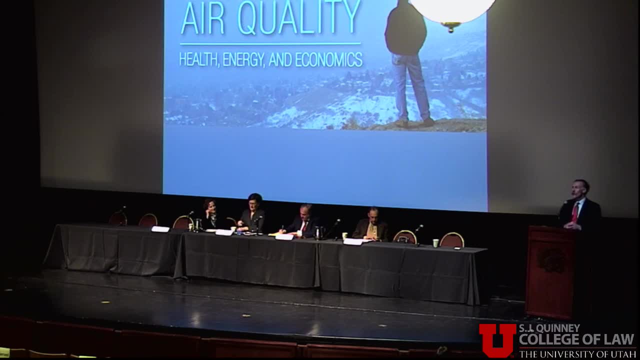 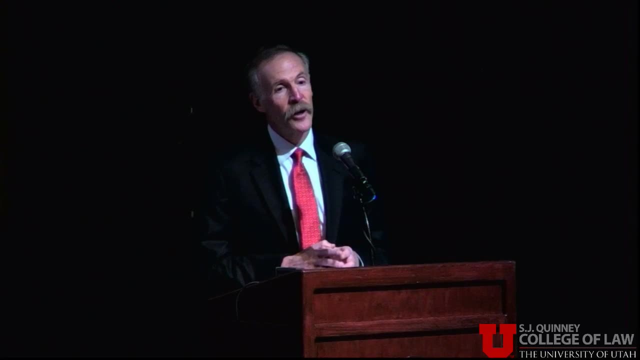 Wasatch Front, We've actually had a rather pleasant winter, ironically from an air quality perspective, And we all enjoyed that. But we know that our air quality problems are far from solved here. We know how much they affect our health, our economy, our general welfare. So this is indeed an extremely important topic And we're looking forward to a very illuminating discussion, as usual. 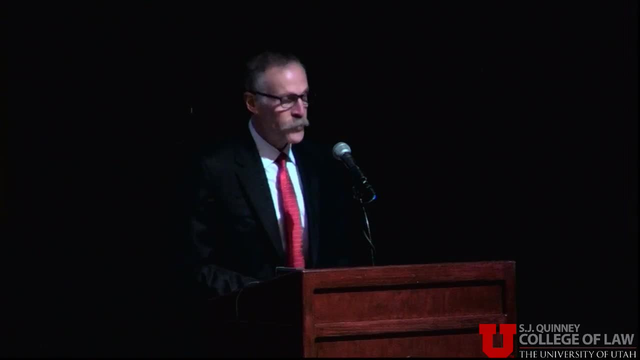 I want to give some thanks, to begin first to our principal funders and sponsors for the symposium and other programs of the Stegner Center. Principal funding for the symposium comes from the R Harold Burton Foundation, Our founding donor for the symposium, the principal funder since 1996.. 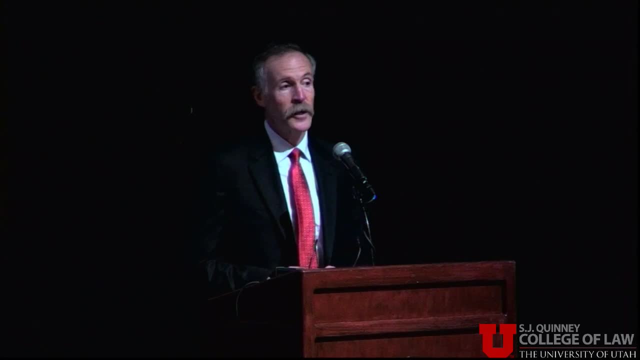 Also from the Cultural Vision Fund which, in addition to funding the symposium, also provides very generous funding for other Stegner Center events, our Young Lecture Series, our other speaker programs as well. Also our sponsors, the SJ and Jesse E Quinney Foundation. of course, the Quinney Foundation. 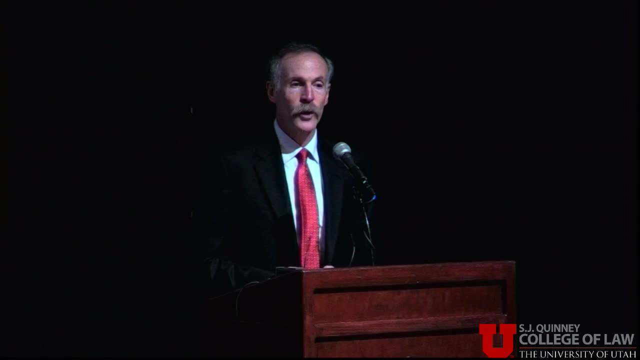 provided the naming gift for the College of Law, for which we are very deeply grateful: the Nature Conservancy in Utah, the American Bar Association's section of energy, environmental resources and the Natural Resources Law Forum, which is the student environmental law group at the College of Law. 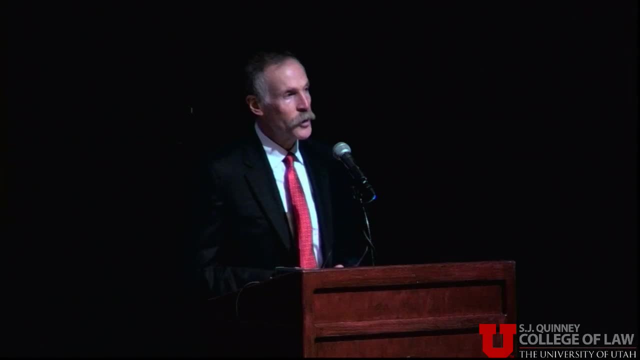 I also want to thank and acknowledge some of the people most responsible for this year's symposium. First, Professor Lincoln Davies. um special thanks to Lincoln for being the principal architect and organizer of the substance of the symposium. Mr Lincoln, who is here dressed as a principal, directs that sort of a Brownian building. that kind of involves people who areisy. 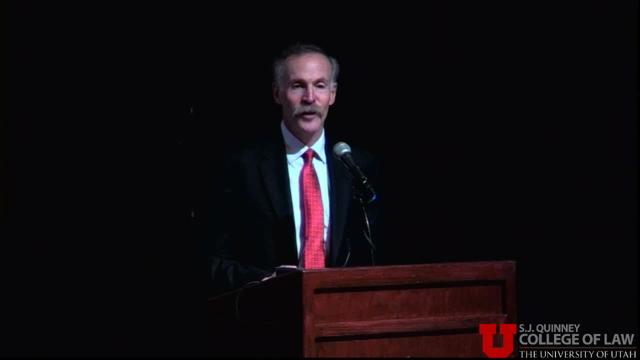 tran Hong to Lincoln for the zwischen jury andع first year as Associate Dean for Academic Affairs, which is quite a challenge, while coaching our National Environmental Law Moot Court team, which, for the second year in a row, won a Best Brief Award at the national competition. 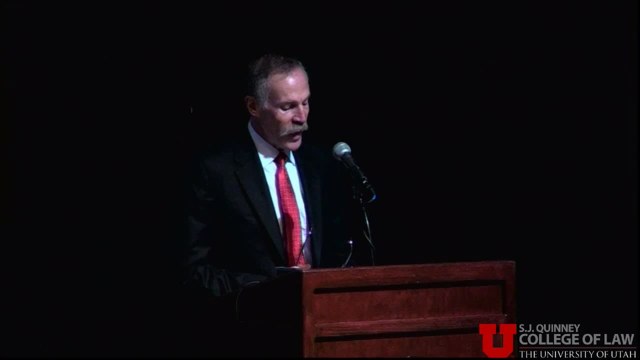 So a lot of work, but kudos and thanks to Lincoln for that. I also want to acknowledge Jan Nystrom, who's sitting in the back, our Associate Director of the Stegner Center, who's done her usual brilliant job of organizing and herding all. 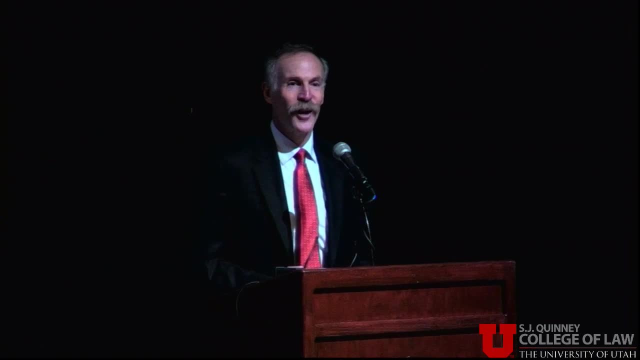 us faculty and administrative cats to make this event happen: Erin Reardon and others on the College of Law events team who have arranged for all the travel and meals and so forth, and a whole cadre of other folks that you'll meet out in the lobby from the College of Law staff and IT team helping with registration. 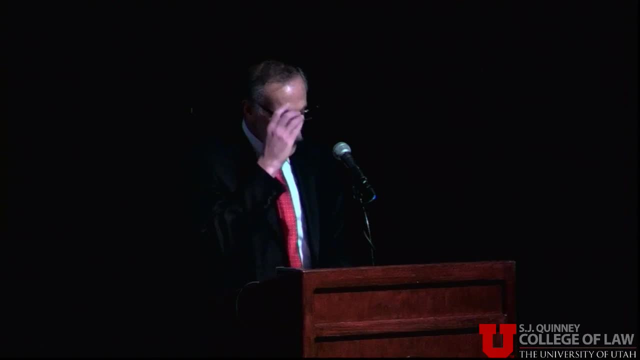 And IT support and so forth. So next, those boring but really important announcements about logistics. During the breaks there will be refreshments downstairs in the Rose Room, where breakfast was served this morning. You are allowed to bring beverages into the room, but not food. 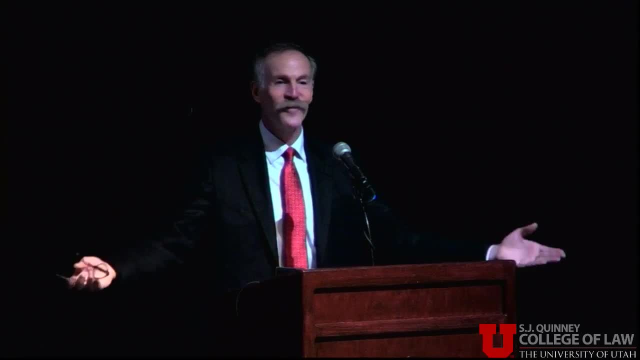 We will be enforcing that with civil penalties and other things that environmental lawyers know all about. We also love to have a break. We'd love to support our local bookstore, the King's English. They will be selling books by the authors and others on this topic, so we hope that. 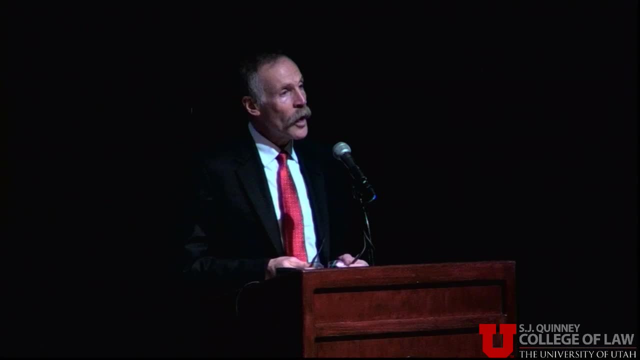 you will visit their table and patronize that enterprise. We're also joined by several local organizations focused on air quality and other environmental matters. They've got tables downstairs. We hope you will take the time to visit them, chat with them, Take a look at their literature. 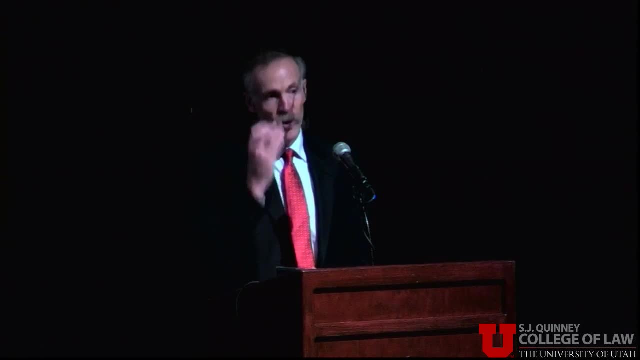 There are evaluation forms in your packets. These are really, really helpful to us in evaluating the symposium, in looking at new topics for next year and to reporting- for reporting to our funders. So I hope you'll take a few minutes to fill out those forms and return them. 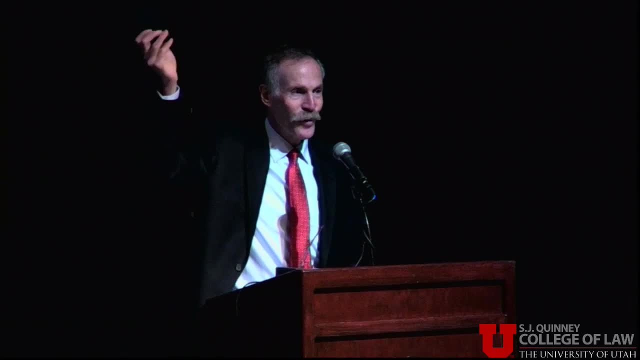 And finally, please silence or turn off your cell phones. David and I were just talking about duck. I'm sorry. We have a lot of duck sounds on his cell phone, so he is turning it off right now. Okay, So with that we are going to move right into our opening panel. 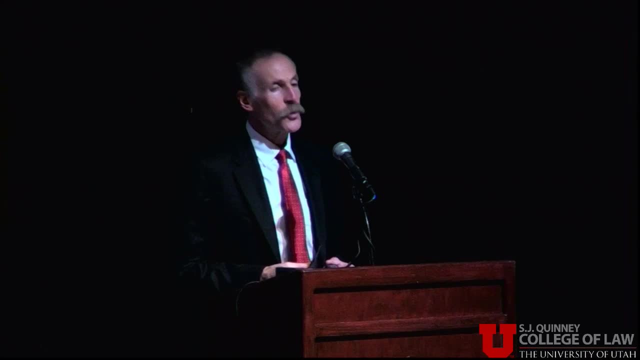 I will introduce the speakers very briefly, as we will do throughout the symposium. All of our speakers have very long, very impressive resumes, but we prefer to devote our time to the substance and to question and answer, So we will simply be identifying each of the speakers. 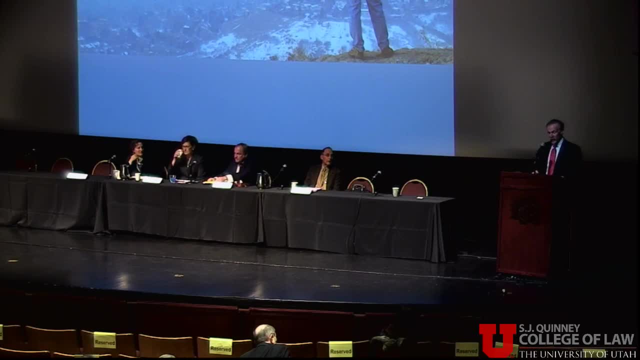 you can read more about them in your packets. So our first panel, the Clean Air Act: Origins and Directions. we're going to hear from the speakers in the order in which they are seated. I'm going to introduce them all. They'll come up in sequence and then we will take question and answer as a panel. 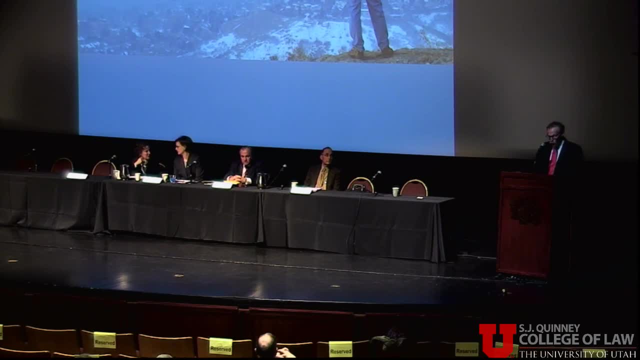 So the first speaker will be Professor David Schoenbrode, who is the trustee professor of law at New York Law School and a visiting scholar at the American Enterprise Institute. Next we'll hear from Professor Robert Percival, from whom we also heard yesterday as our Stegner. 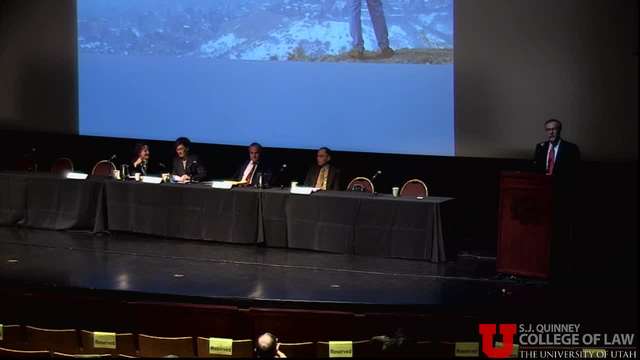 lecturer. He is the Robert F Stanton Professor of Law and Director of the Environmental Law Program at the University of Maryland's Francis King Carey School of Law. Third, we'll hear from Anne Weeks, who is Senior Counsel and Legal Director of the Clean Air. 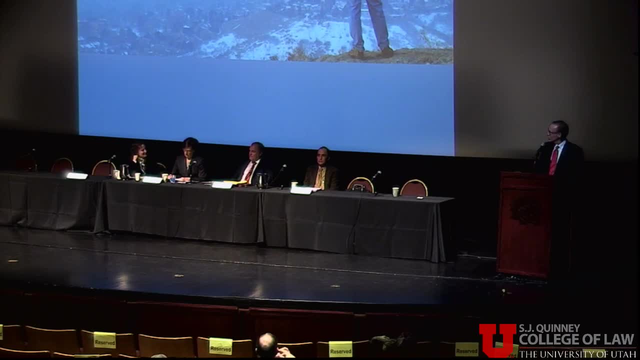 Task Force And finally, from last but not least, from Professor Alice Kazwan, who is a professor at the University of San Francisco School of Law This semester. she is a visiting professor at the University of California, Berkeley. Please help me to welcome our first speaker, David Schoenbrode. 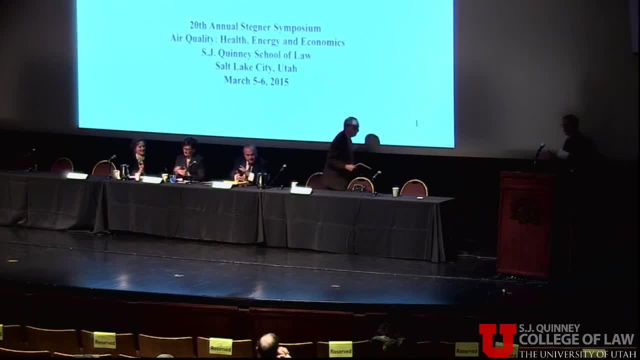 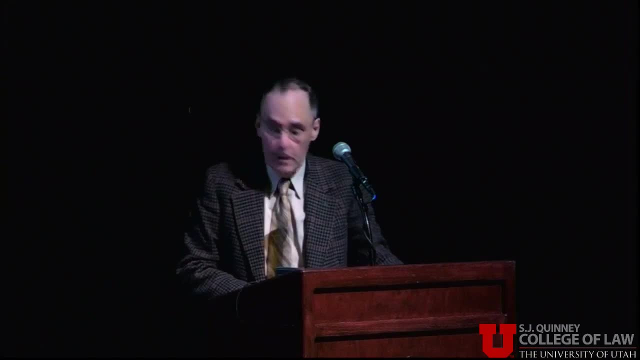 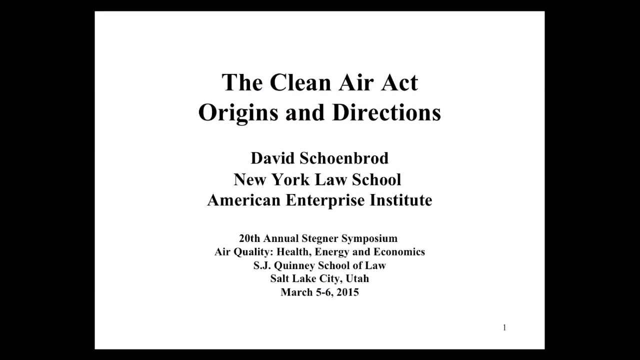 DAVID SCHOENBRODE JR. Well, thank you for bringing me here. Thank you for bringing us all together. Is this microphone working properly? Okay, When I first read the Clean Air Act soon after it passed in 1970, it delighted me because 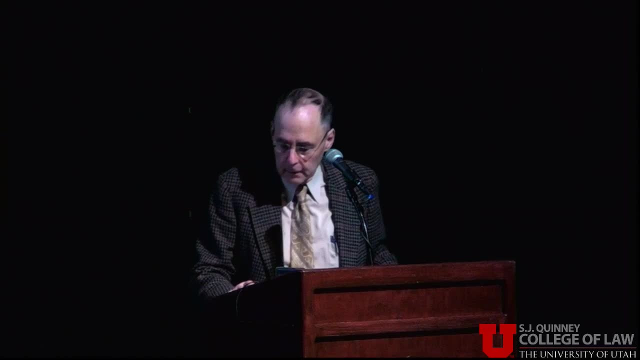 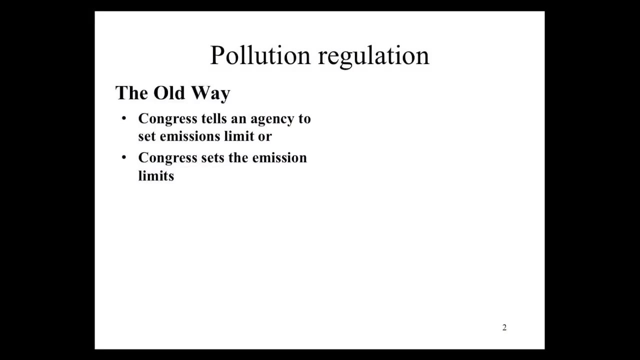 it promised to protect health in a new way. In the old way, Congress tells an agency to set emission limits or Congress sets those emission limits itself. The old way seemed problematic because the regulated industries would capture the agency that set the emission limits and therefore be captured. 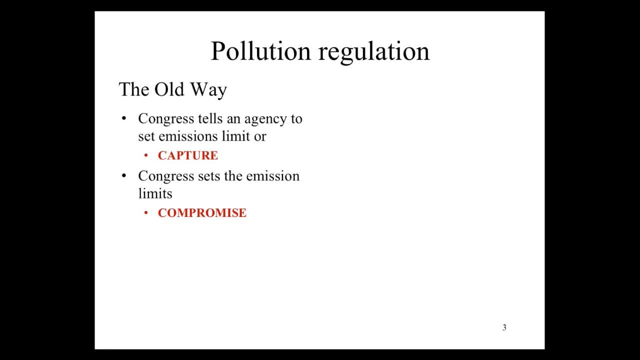 Or if Congress set the emission limits itself, it would have to compromise. That's the nature of Congress, of course. In the new way, Congress tells an agency to make emission limits sufficient to protect health by a deadline. Perfection. Where is this? 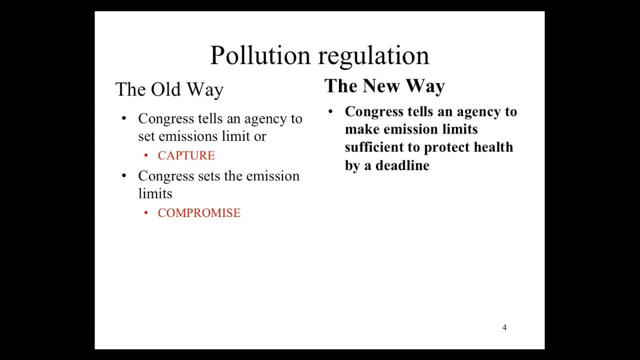 Okay, Okay, It's not advancing. Hmm, Ah, you need a dean. That's why we have deans. That's my role, DAVID SCHOENBRODE JR. Okay, Thank you very much. So here's how Congress seemed to produce perfection. 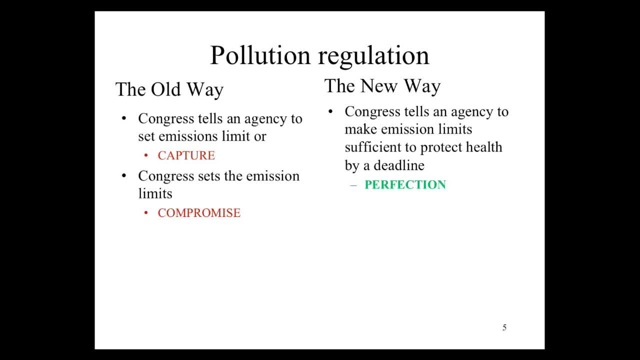 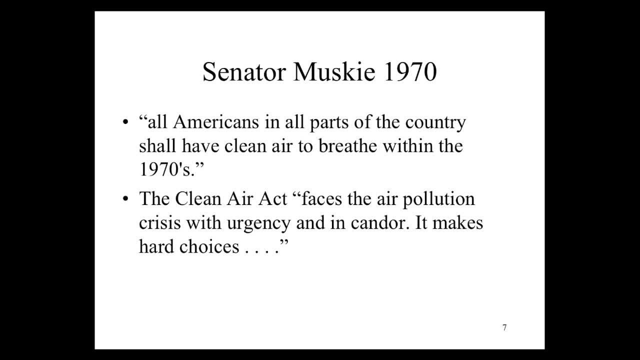 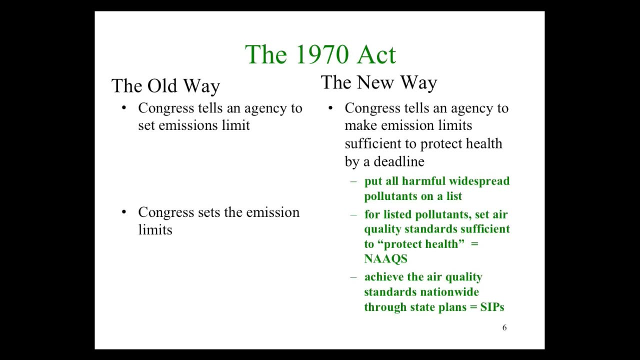 Congress told the EPA- What am I not knowing? Sorry about that. It told EPA to put all the harmful widespread pollutants on a list and then for each one of these pollutants to set air quality standards. they're called National Ambient Air Quality Standards. 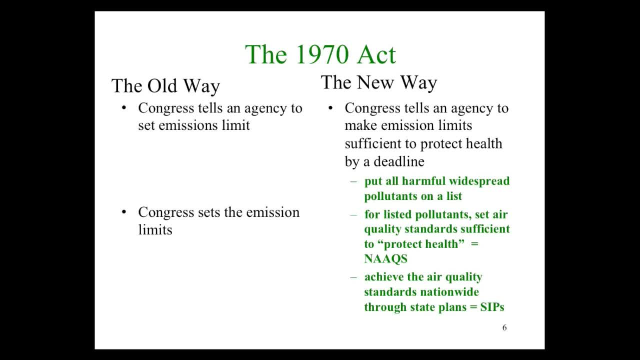 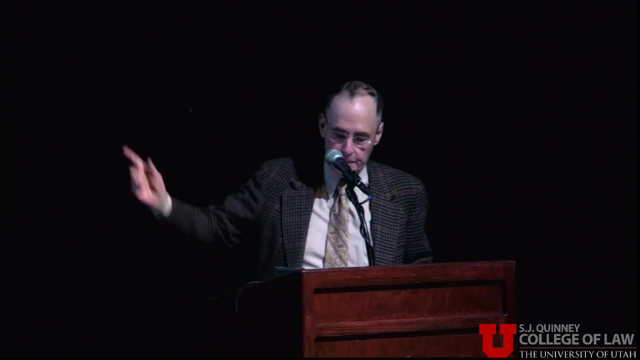 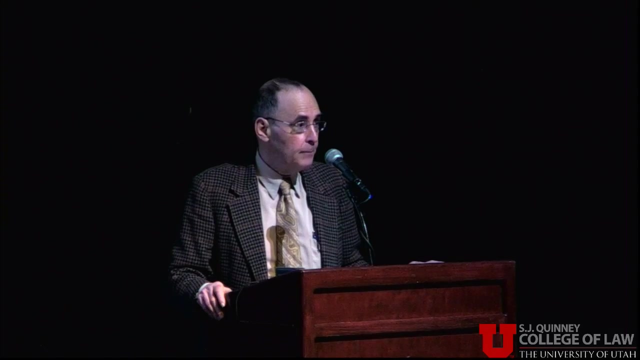 They're supposed to protect health, and environmental lawyers know them as NACs by their acronym- And then to achieve the standards everywhere, EPA is supposed to rely upon state implementation plans, which environmental lawyers know as SIPs. Now, the statute also imposed deadlines by which EPA must do these duties, impose the 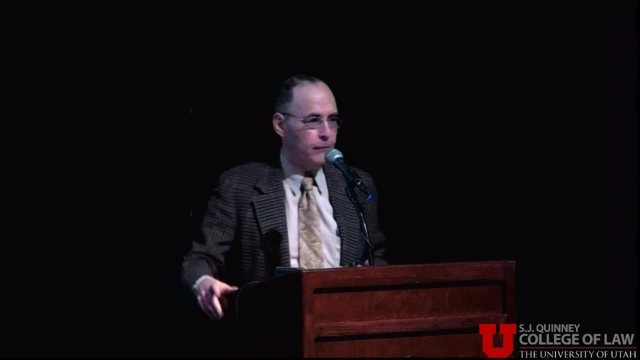 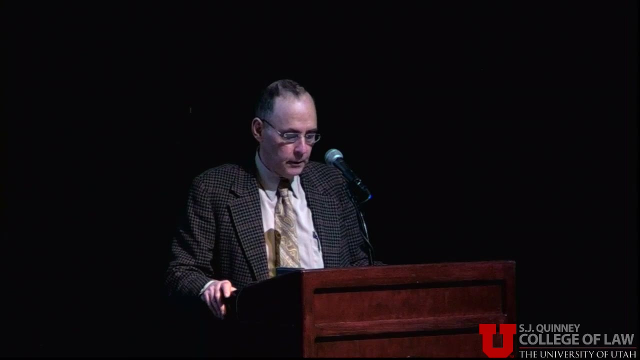 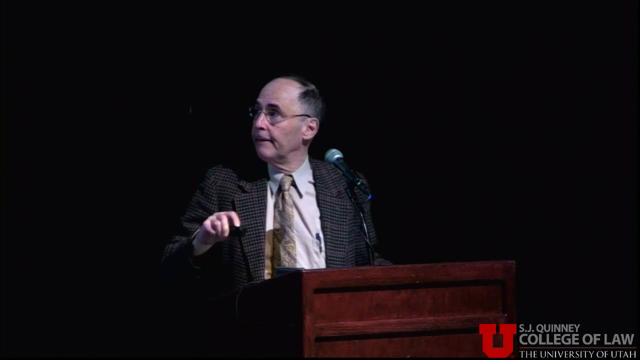 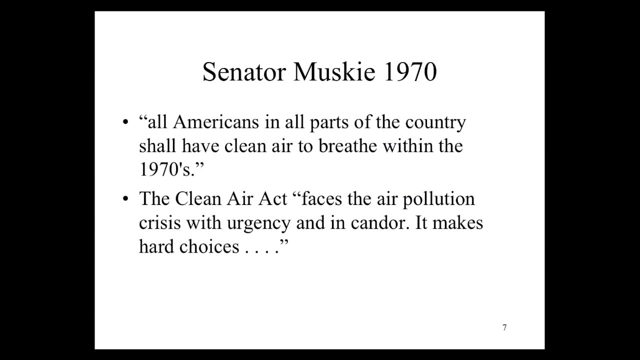 analogous duties for those harmful pollutants that are not widespread and therefore not on the list, And authorize citizens to enforce these deadlines in court. On this basis, the bill's chief author, Senator Edmund Muskie, stated all Americans and all parts of the country shall have clean air to breathe within the 1970s, and he also went. 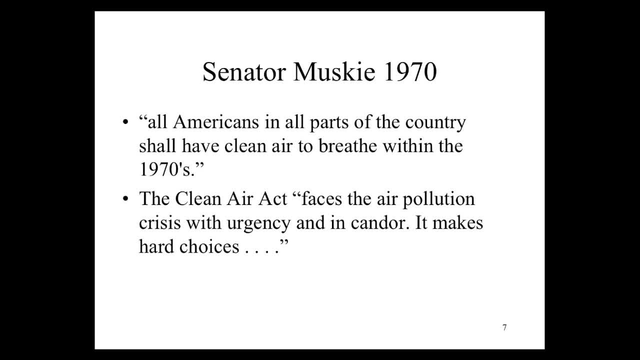 on to say that Congress had made the hard choices with candor. so you could see why I thought this was important. I thought this was just a great statute. Now, the statute also contains some bits of the old way in it as well. Dean, I'd like you to help me. 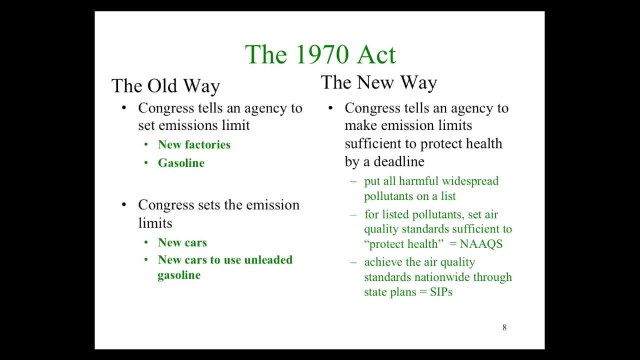 Next, please? Okay, first of all, Congress gave the EPA broad discretion to regulate power plants and other factories, And it also gave EPA broad discretion in terms of regulating gasoline, at least the gasoline used by the cars that were already on the road. 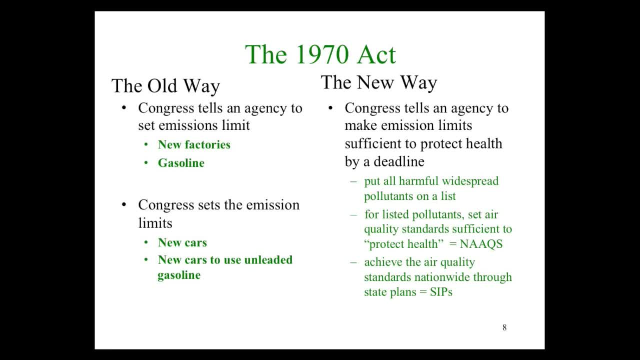 Congress itself took responsibility for deciding that auto manufacturers must cut emissions from new cars by 90 percent, That's on the lower left there. And also it took responsibility for these new cars having to use unleaded gasoline. The reason for that was that the emission costs were going to be reduced in the federal 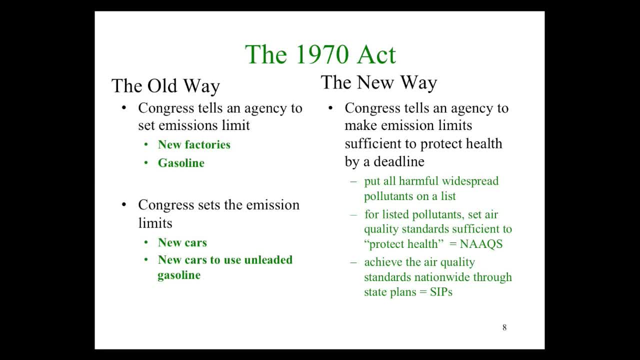 control systems in new cars would not work if the cars used leaded gasoline. Congress would look stupid if it required us to pay for those emission control systems and they didn't function. These two bits of the old way were insufficient to produce the goal of protecting health. 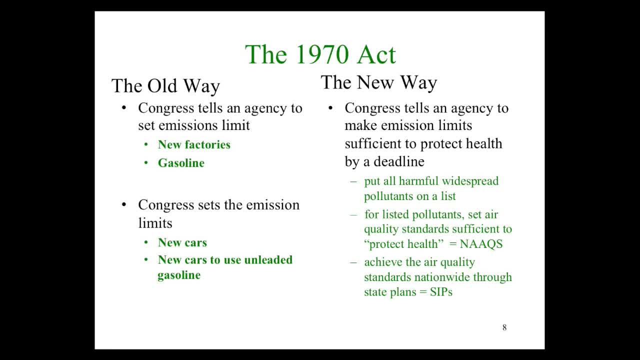 And here's an example: When the new cars would begin to come on the road, the 90% cleaner new cars would begin to come on the road in 1975, there would be 100 million old cars still using leaded gasoline, and that would not be good for health. 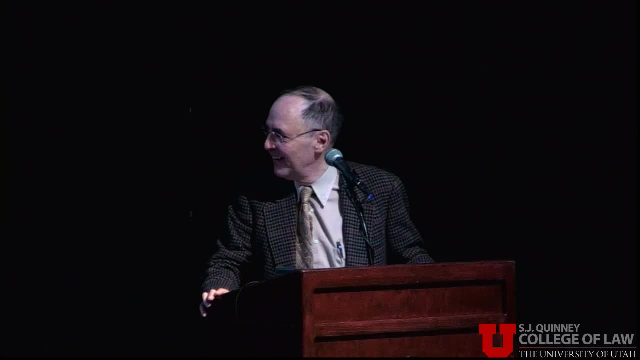 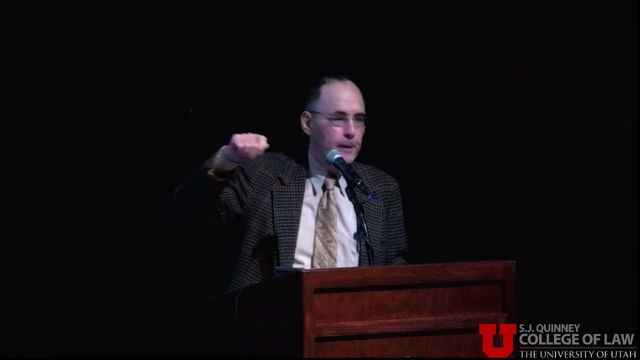 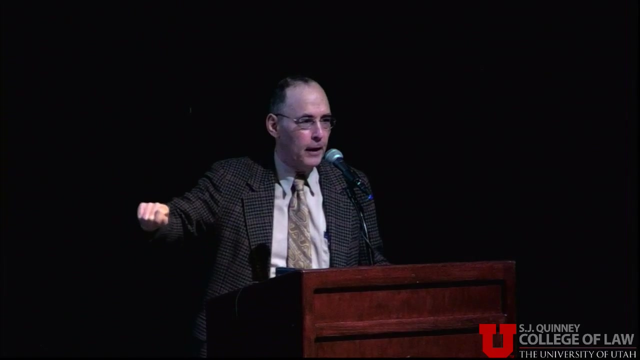 But not to worry. Congress subjected things like lead to the requirement that they be put on the list, that there be ambient air quality standards. there be deadlines, and if you took all the deadlines in the Clean Air Act and put them together for lead, health would be protected. 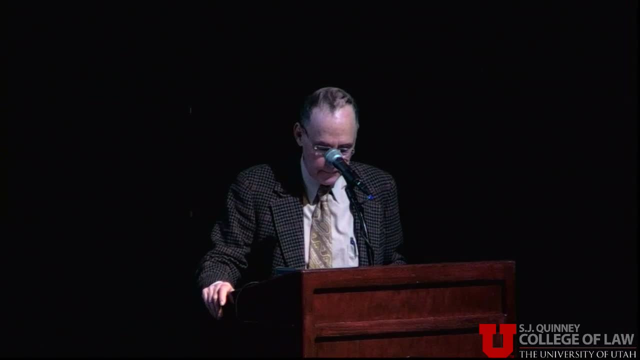 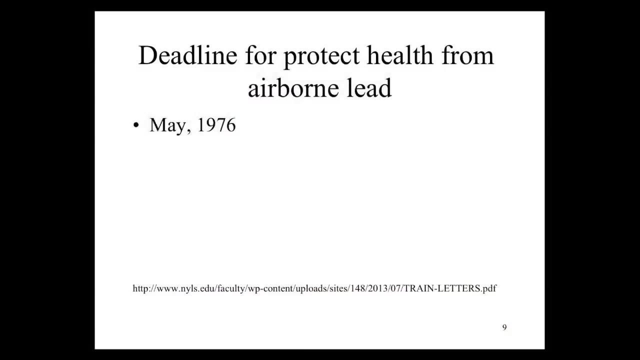 by By 1976, May 1976.. That was the good news, it seemed. Yet within a year of the statute's enactment, EPA decided not to postpone any decision on whether to regulate the gas, the lead in the gas of these 100 million old cars and it. 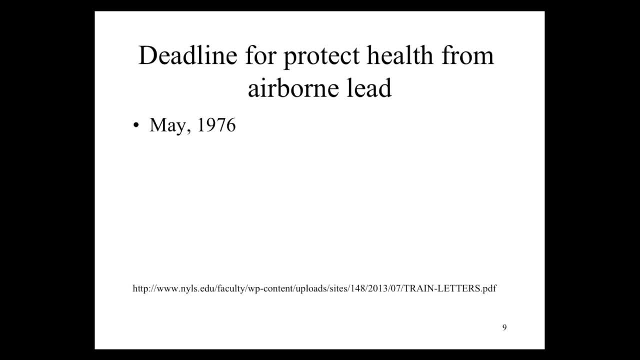 decided not to set an air quality standard for lead, thus freeing itself from the deadline to protect health by 1976.. Now we at NRDC, we are one of the most important creditors in this country in the history of the National Highway Patrol, as you probably know. 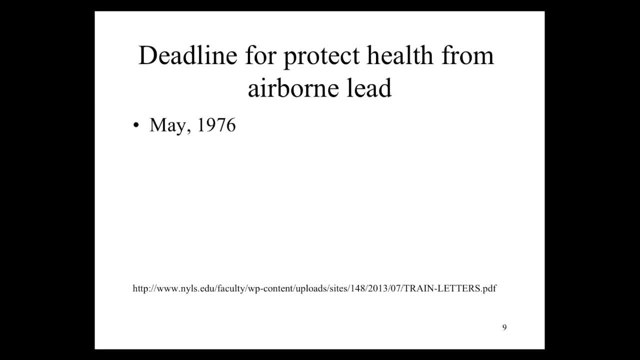 We have been collecting the legal evidence of the court. in the minds of many of you- And I'm certain many of you would suggest me that I'm only referring to the DC Circuit. I am not, And you have a good chance of knowing what happened in the first decade. The DC Circuit in 1972, gave the EPA 30 days to rule on the proposed limit on lead and gasoline used by the old cars. EPA did promulgate the reduction and was later upheld in the Ethel case. The Second Circuit required EPA to set an air quality standard for lead, which was later upheld in the 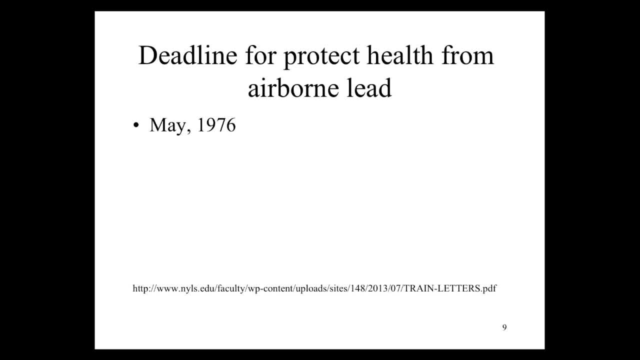 2nd Circuit. The Second Circuit required EPA to set an air quality standard for lead, which was later upheld in the 3rd Circuit, EPA to set an air quality standard for lead, which was later upheld in the Lead Industries Association case. 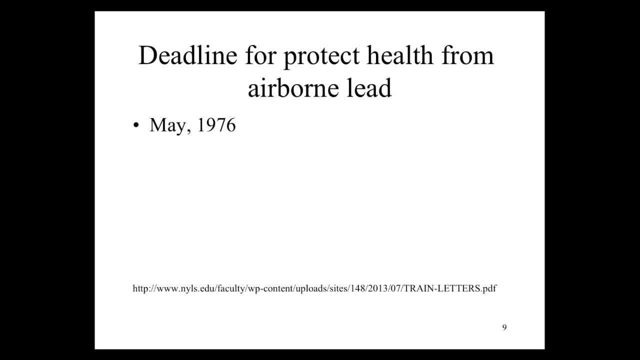 Now, the reason we wanted an ambient air quality standard was not that we wanted state implementation plans to regulate lead and gasoline. we wanted to put pressure on EPA to take its weak regulation of lead on gasoline and make it stronger. Now, by the way, for those of you who teach the case or want to know more about this, 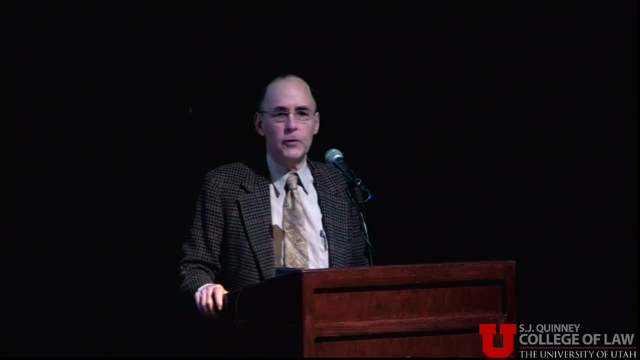 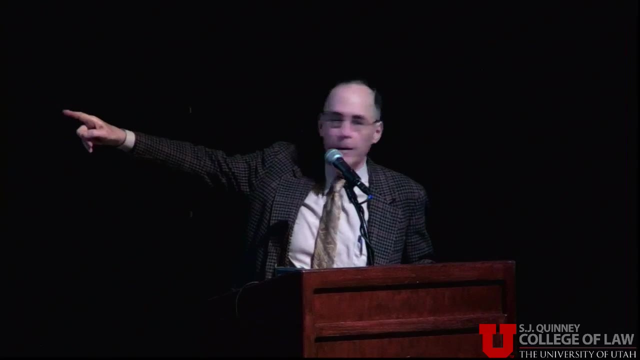 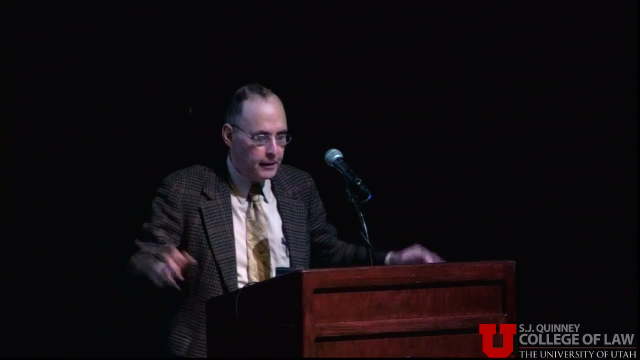 I had a very lengthy exchange of letters- 19 pages of letters- between me and EPA Administrator Russell Train back then. it was like 40 years ago And if you're interested, the link at the bottom there is the letters. Very unusual thing to have some environmental advocate and the EPA Administrator anyway. 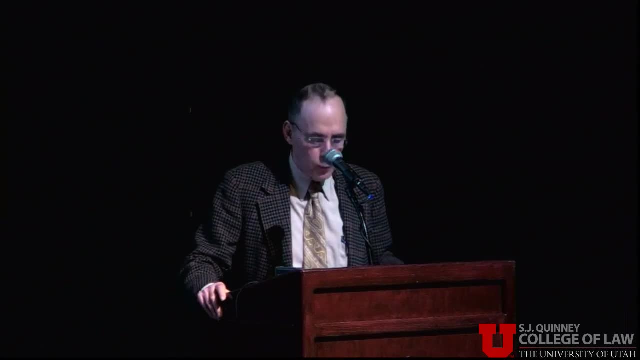 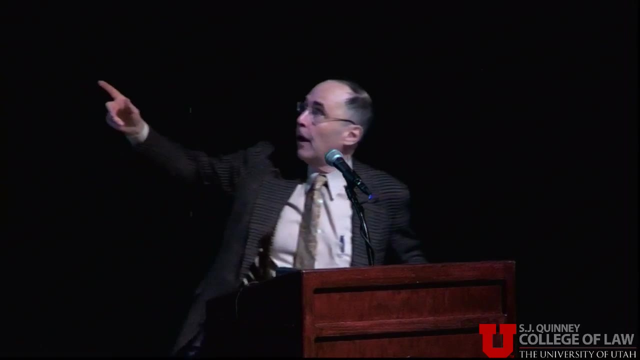 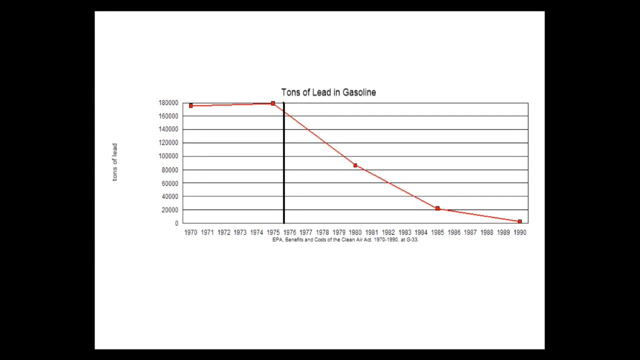 they're kind of interesting in retrospect. So here's what results. Here was the lead rem— The Lead Industries Association Lead emissions that resulted And if you look up there at the graph you'll see that lead emissions from gasoline actually went up slightly by 1975 and only went down just a tiny bit by 1976.. 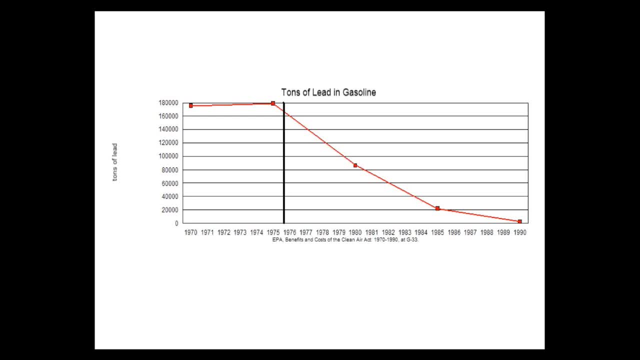 That's how far they got in protecting health right. The vertical line, of course, is the deadline. So there was a little reduction by 1976, and most of the subsequent reduction came not from the new way but the old way. 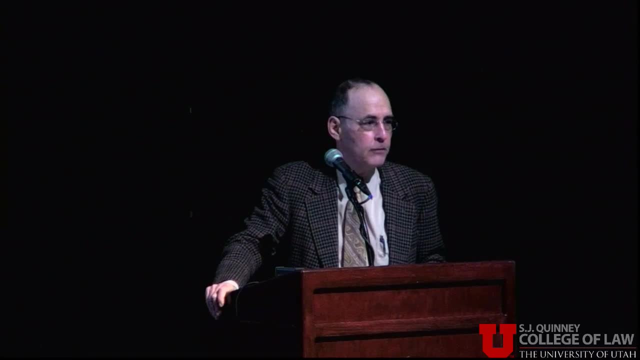 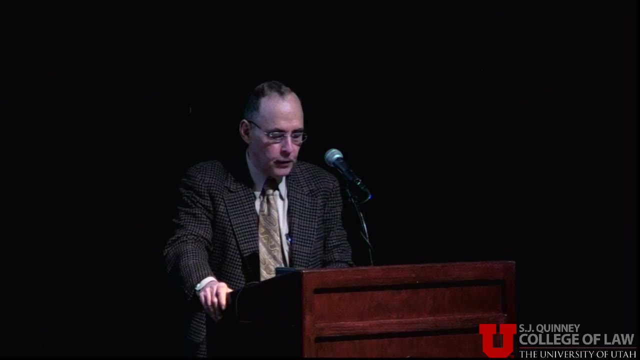 Because Congress had taken responsibility for saying that the new cars have to use unleaded gasoline. And it was not just conservative Republicans who frustrated the faithful implementation of the new way. In the 1970s, liberal Democrats in Congress lobbied the EPA not to regulate lead and gasoline. 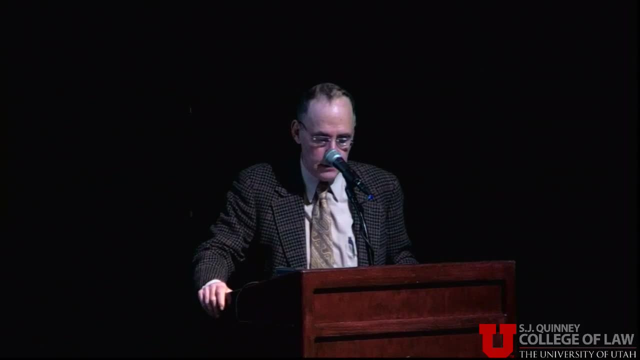 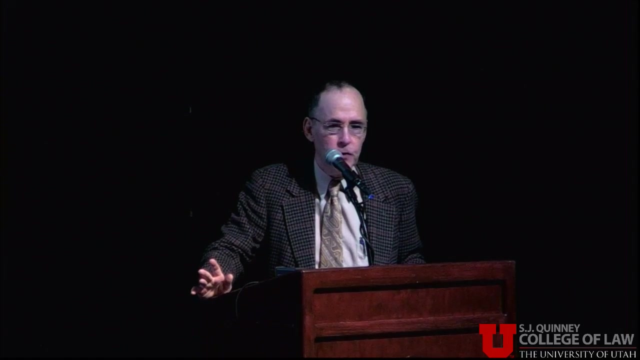 used by the old cars and not to set a tough ambient air quality standard. In addition, President Jimmy Carter, who campaigned for office as an ardent environmentalist, weakened the phase-down regulations. Then along comes President Ronald Reagan. In the early days of his administration, his people were gunning to actually weaken the 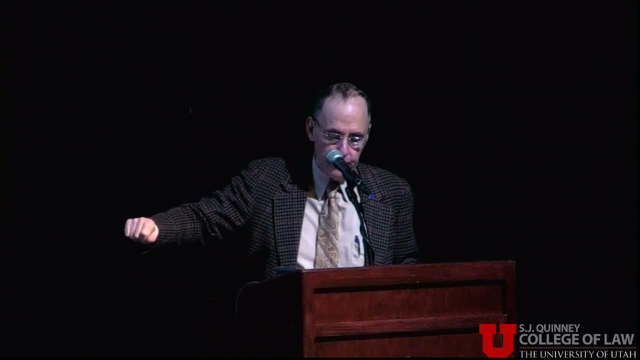 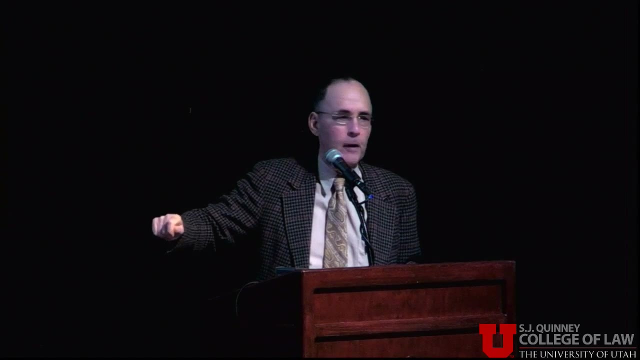 regulations on lead used by the old cars even more than Carter had. But actually they turned around and they didn't do that And the reason was really the chief payoff of our getting EPA to do an ambient air quality standard for lead is it had to confront the health case. when they confronted the health, 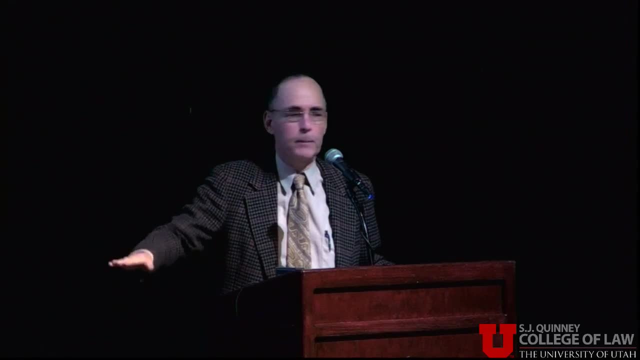 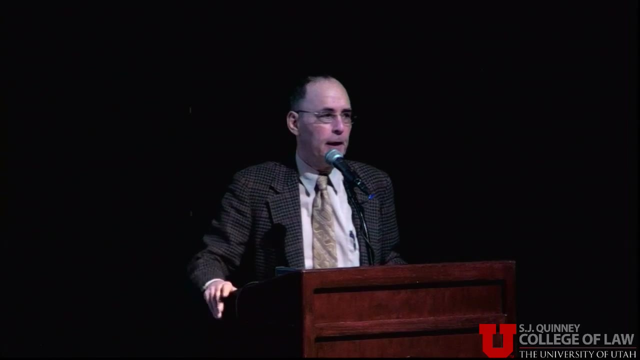 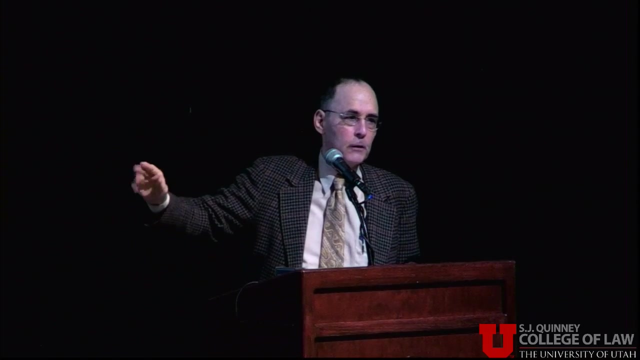 case solid, and the Reagan people, to their credit, decided: you know, there's enough health stuff going on here, we're not going to do it. Then something else interesting happened, As more and more of those new cars started replacing the old cars, and the new cars could. 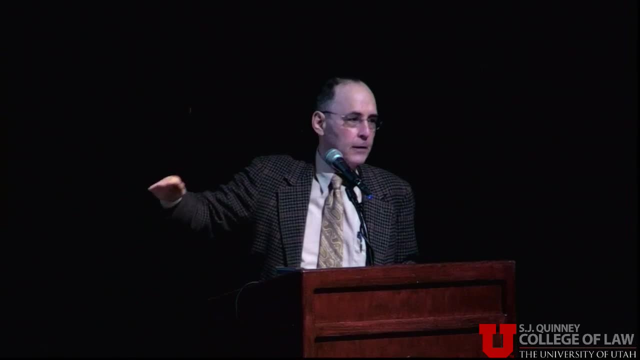 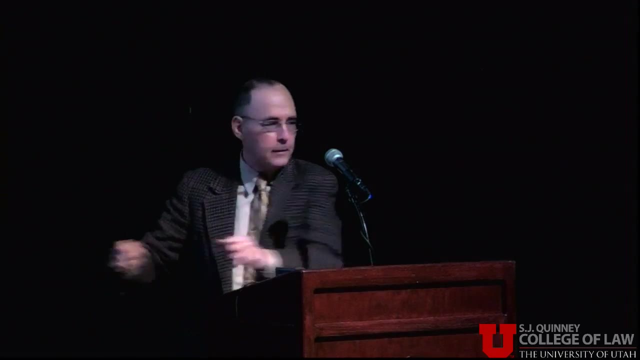 only use leaded gasoline. the market for leaded gasoline was getting smaller and smaller. So you think about ExxonMobil Texaco. now they've got two sets of trucks out there, one carrying leaded gasoline, one carrying unleaded gasoline- and that's an expense and they don't like the expense. But on the other hand they didn't want to just stop selling leaded gasoline, because then these little niche refiners would soak up that market. They didn't want to lose market share. The solution: Get EPA to ban leaded gasoline. So what happened was the big part of the refining. 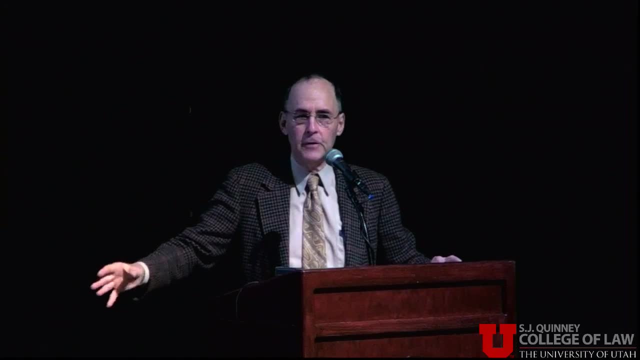 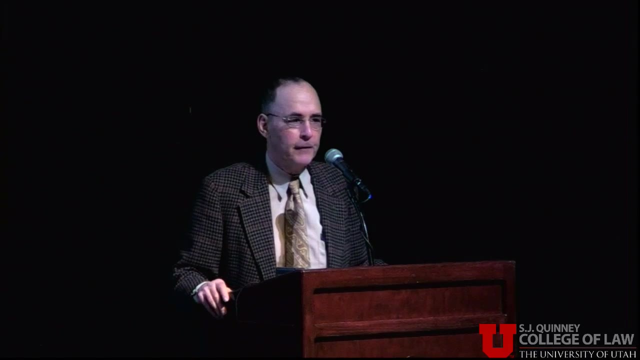 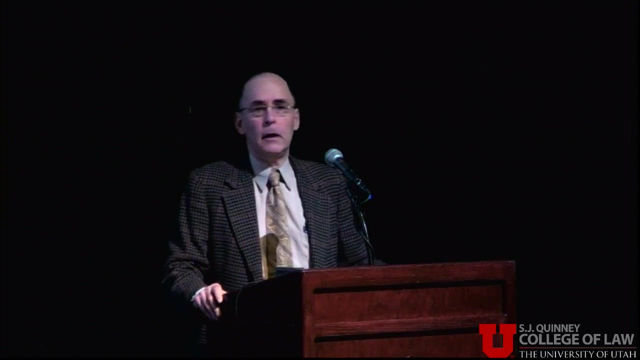 industry, at least some segments of it, began to change sides. So today, EPA will tell you what a great thing they did. We got tough on gasoline, lead on gasoline. They didn't get tough until big oil changed. Now, years later, I happened to be talking to an administrator. 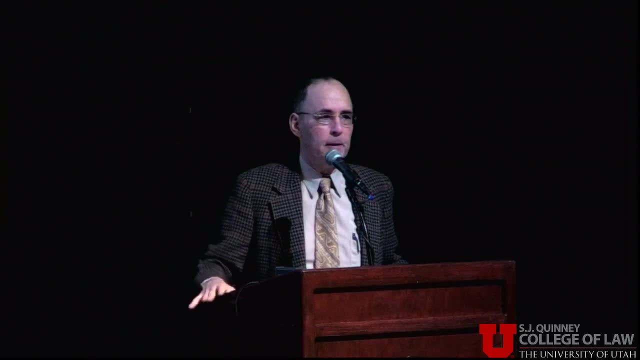 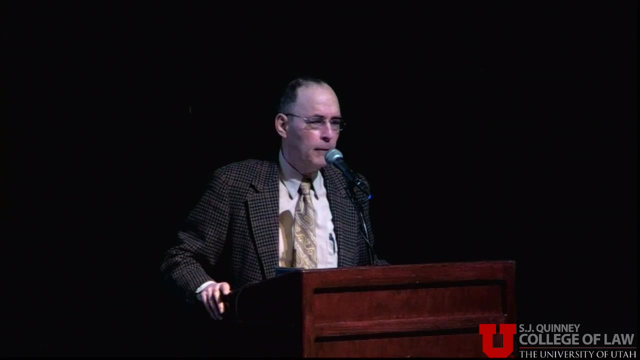 of the train. this was years after he left government in his office about something totally different. And as I was leaving the room he said: how did you know lead was so bad? And what I told him was: I talked to the physicians on the phone and they said: well, 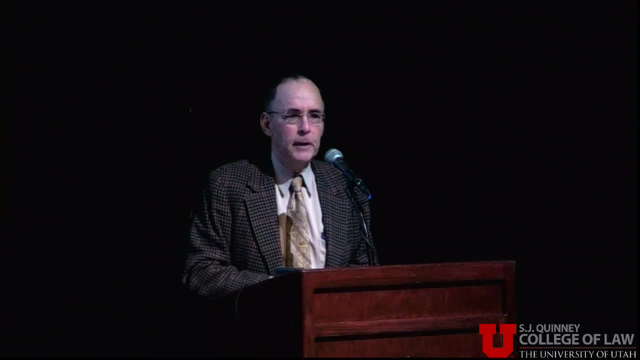 I'm the staff of EPA, And what that told me was that he wasn't getting the news. He was a totally honorable man. He would not have asked me that question otherwise, And what I deduced from that was that the political pressures on EPA from Republicans and Democrats was keeping the health. 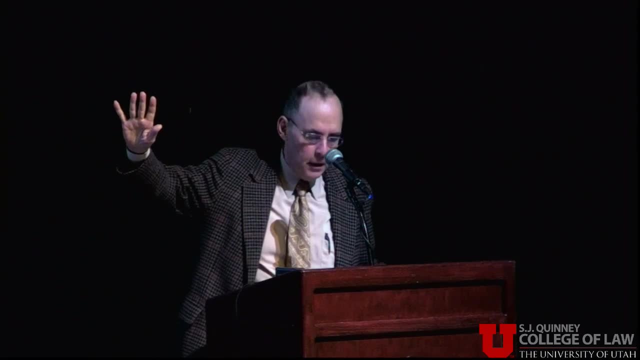 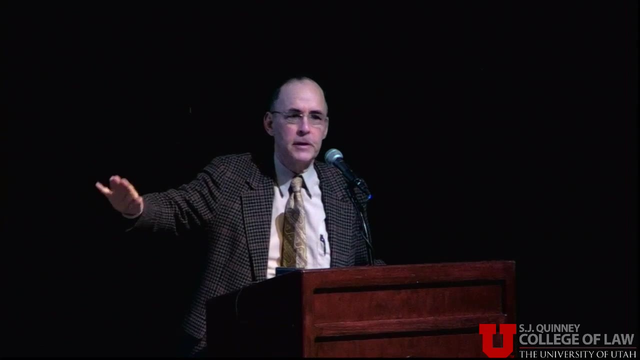 case away from the people making the ultimate decisions. So you know, when Congress says to an agency: protect health, that doesn't mean health isn't going to be protected. That means the people in Congress avoid the blame for health not being protected. That's what's going. 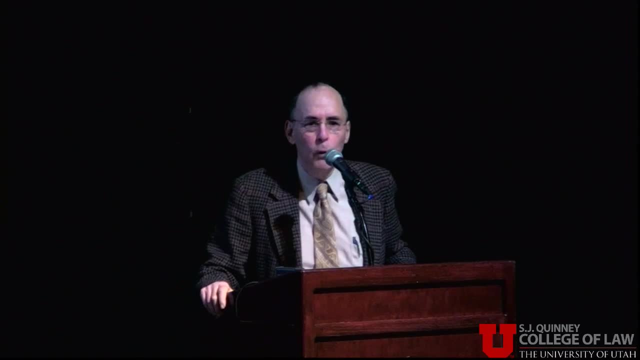 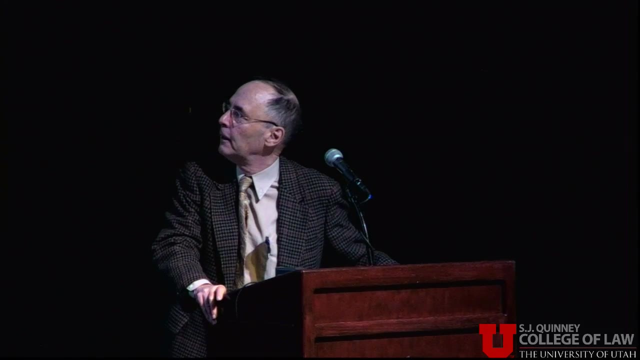 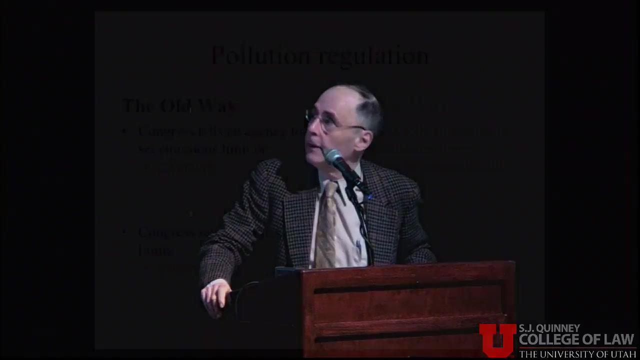 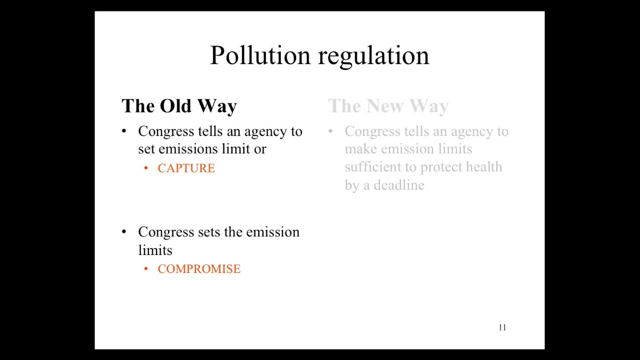 on. So let's think about what would have happened if the new way was not possible. Okay, so we wiped out the new way. Now the old way, the one on the upper left there, telling the agency to do it. that just wouldn't do right, Because you know we're going to have to do it. 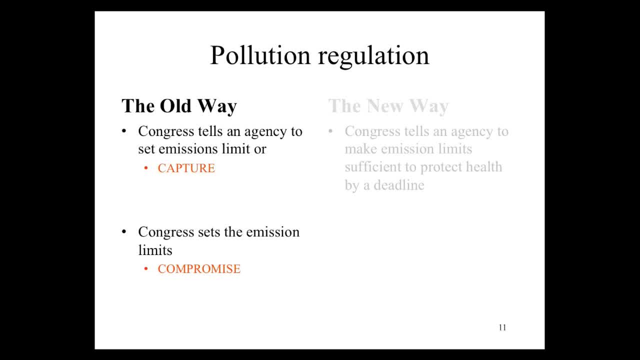 differently. The public had gotten sick of just passing the buck to the agency. That's what had happened under the old Clean Air Act- and it had gotten nowhere, and there was a real revolt against that. Besides that, back in 1970, the pollution issue that most bugged up the public was lead in. 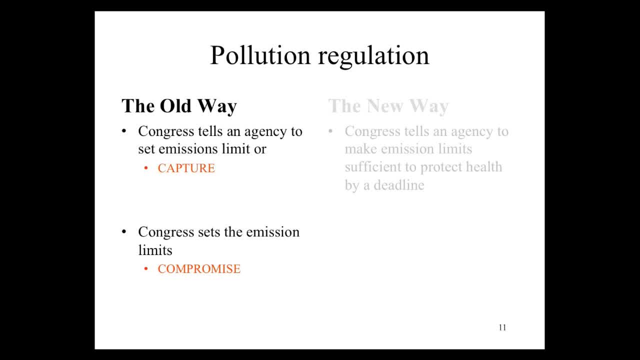 gasoline. So Congress would have had to do something. okay, It would have had to regulate not just the lead in gasoline used by the new cars but the old cars. So the question is how much There would have had to be a compromise right Now as to the new cars. Congress had said. 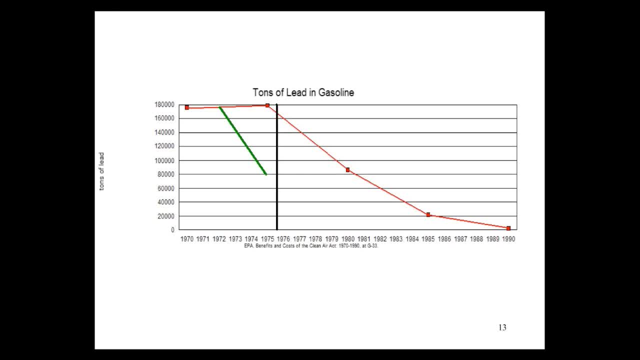 they got to reduce 90%. How much would Congress have caused the refiners to reduce lead in gasoline? Well, the chief interest group there actually is the lead additive makers, and they're not nearly as powerful as the automakers. I'm guessing maybe a fifth of a percent. 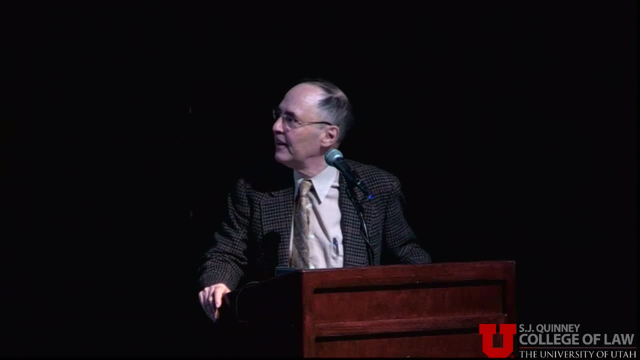 50% reduction over the same time period. These deans are great. Okay, There we go. No, that's right, Go back to where you were. There we go, Perfect, Okay. So that's, I think, what Congress. 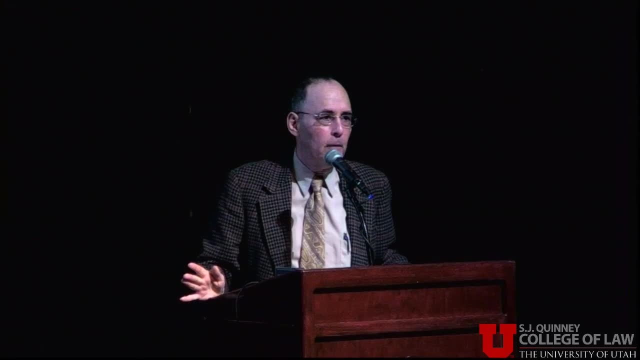 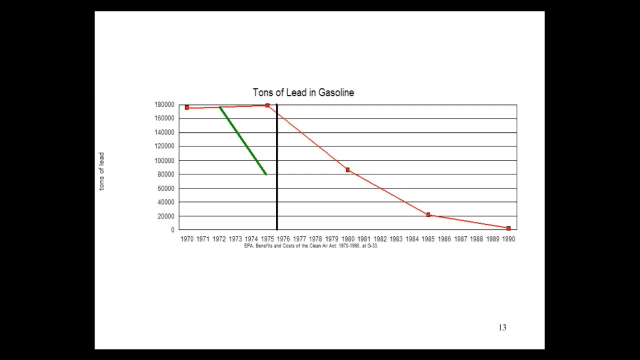 would have done Now. things wouldn't have stopped there, though, for the same reasons that things didn't stop going down on lead later on either, Because, first of all, there'd be more and more new cars coming along that couldn't use the lead in gasoline, And, second of all, ultimately, 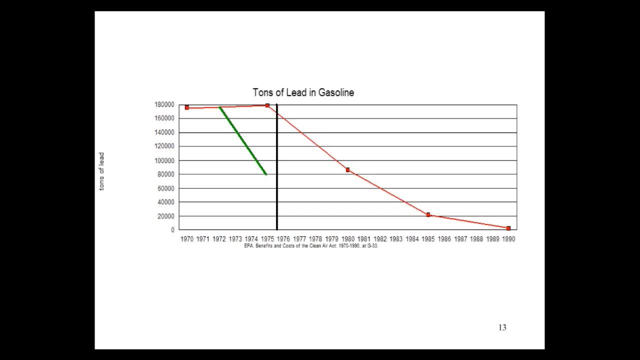 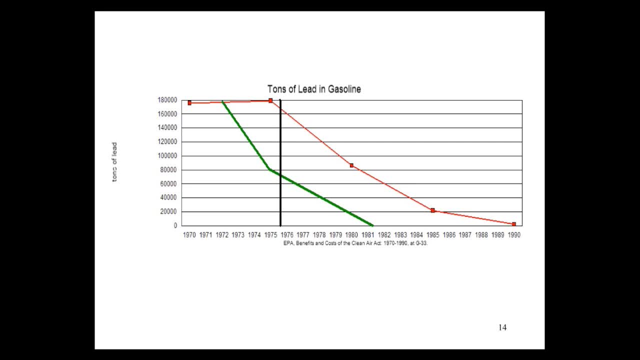 the big refiners wouldn't want to carry two grades of gasoline, So we're in a projectory. The next slide, please. Projectory like this, Okay, Something like this, Okay. So let's think about what the health consequences are of. 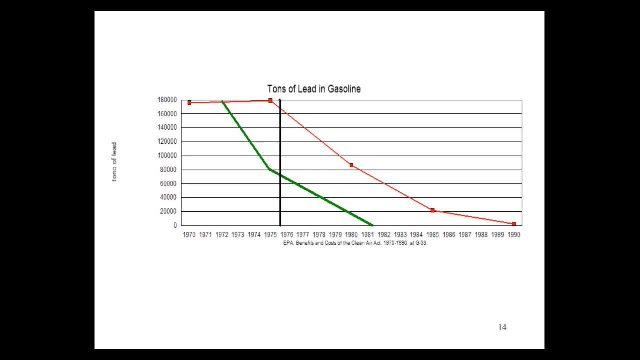 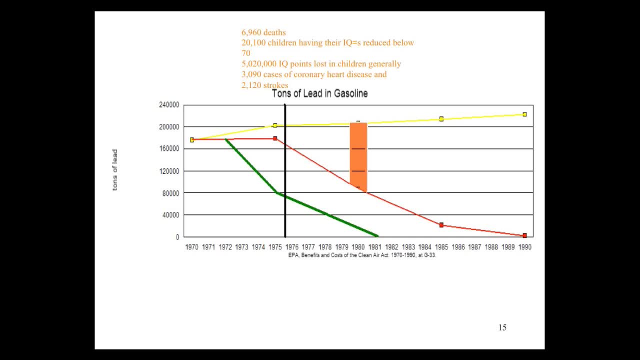 being on that slower red trajectory for getting rid of lead, rather than the green trajectory. We need the next one. Okay, On this graph you have EPA's reduction in yellow of how much lead there would have been without the Clean Air Act. The area in orange is EPA's calculation of how much lead its regulations got out of gasoline. 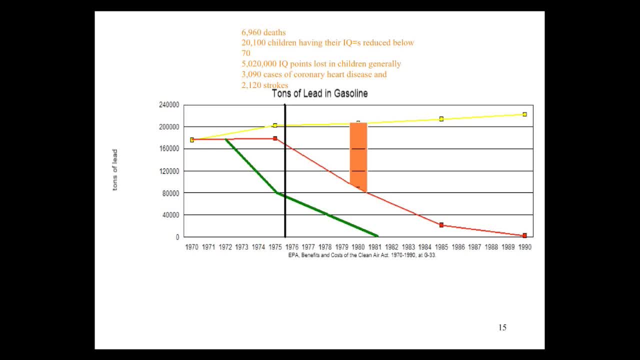 in the year 1980.. Okay, The figures on the top are its estimates of the health benefits of that reduction for just that year: 6,960 deaths averted, and so on and so forth And so on and so on. Really big payoffs from reducing lead. Okay, Now let's think about what we 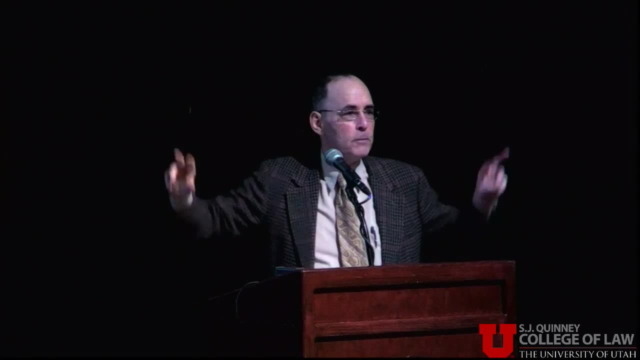 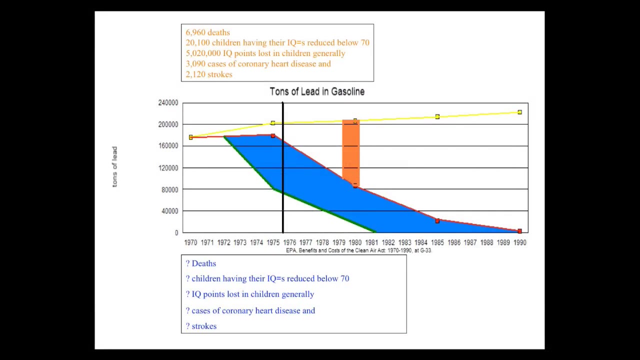 lost by Congress's new, supposedly perfect way. Okay, That's how much extra lead Americans breathe in because of the new way, And you just think about how many deaths came from all this And I would estimate, extrapolating from what EPA says, that the deaths caused in this country. 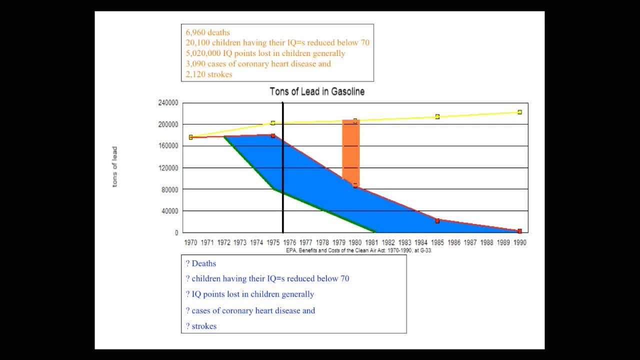 by the new way were about equivalent to American casualties in the war in Vietnam, plus several hundred thousand children lived for life with permanent mental disabilities. That's the consequence of the big talk in Congress. Now it's not just with lead that the new way has. 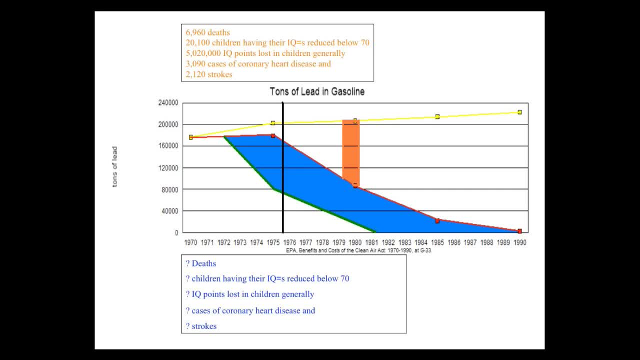 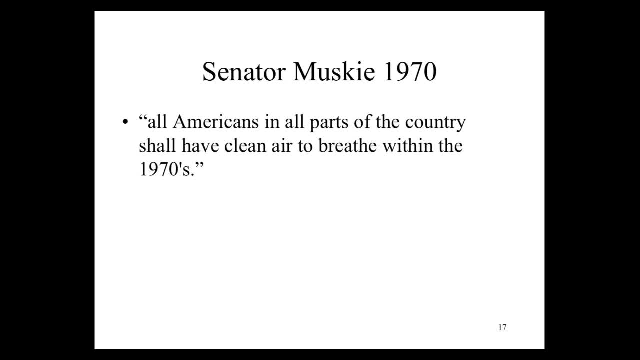 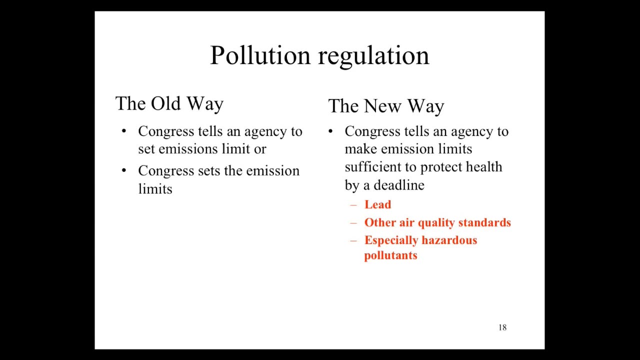 disappointed us. Here's Muski's promise of healthy air in the 1970s for all Americans, with what the new way produced: Not just lead, but the ambient air quality standards in much of the country were not that Muski said would be achieved in. the 70s weren't achieved until the 1990s and into the 2000s, And with hazardous air pollutants- The stuff that's not listed- EPA didn't even begin to regulate most of them until the 1990s. 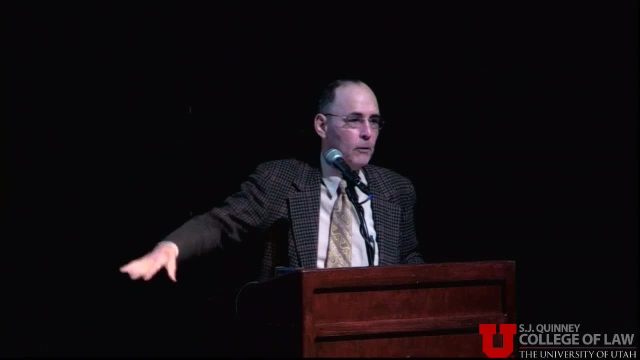 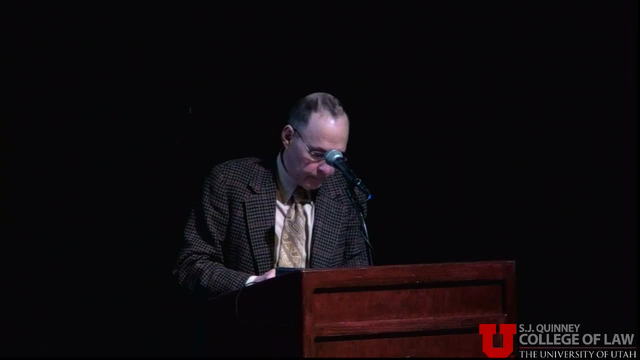 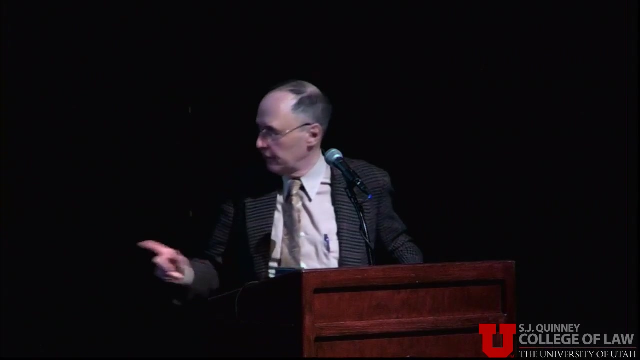 until actually Congress changed the statute to take some more responsibility. The new way was a big, big disappointment, And now let's compare that with what happens when Congress does make the rules. Thank you, There we go. Talked about the new cars already. 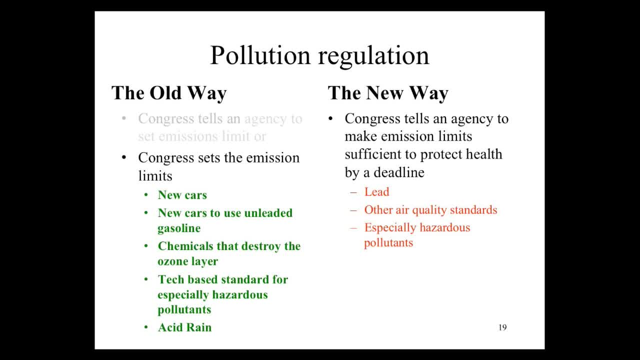 Got more than a 90% reduction. ultimately We got almost 90% by the deadline in 1975.. The new cars have to use unloaded gas. Congress has basically banned the chemicals that destroy the ozone level. It provided in 1990 for tech-based standards for especially hazardous pollutants. 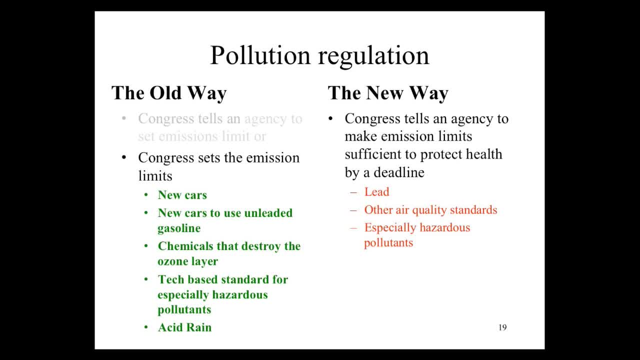 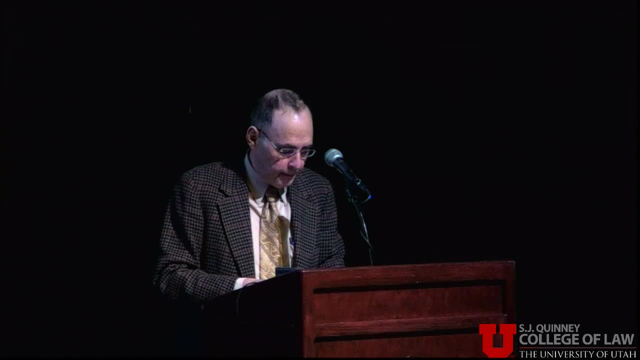 that finally let us have some progress on them. And in 1990, Congress also passed the acid rain program that reduced acid rain emissions by 50%. Some really big changes, Some really big successes that came from Congress making compromises that actually got carried out. 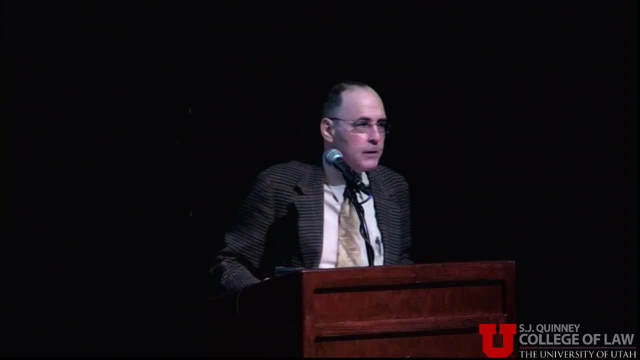 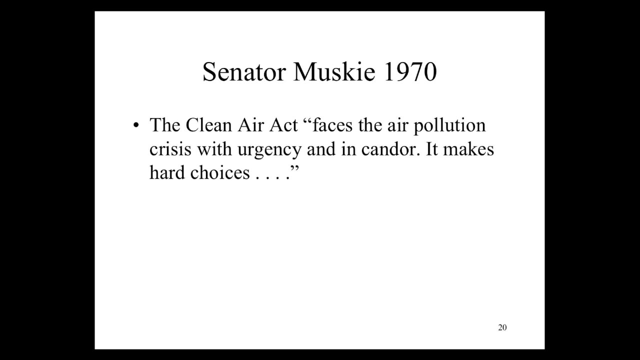 These things actually worked as promised, So why does the new way work so badly? Well, my case is that it's basically dishonest, for all that must be said about candor and honesty. Okay, So there's an analysis of this by Bill. 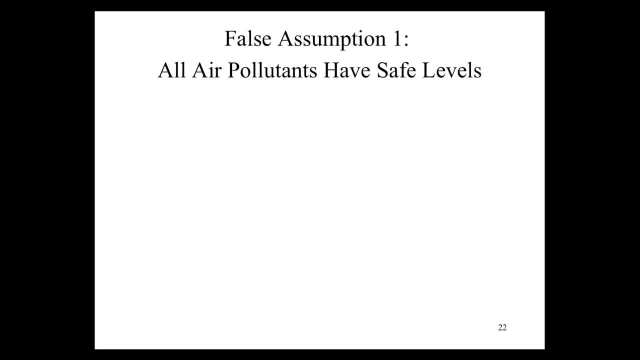 Bill Peterson, who I think some of you know. Some of you must know Bill Peterson- Whoops, I think we're Next one. There it is. This is an article that Bill and I wrote. former Deputy General Counsel of EPA. 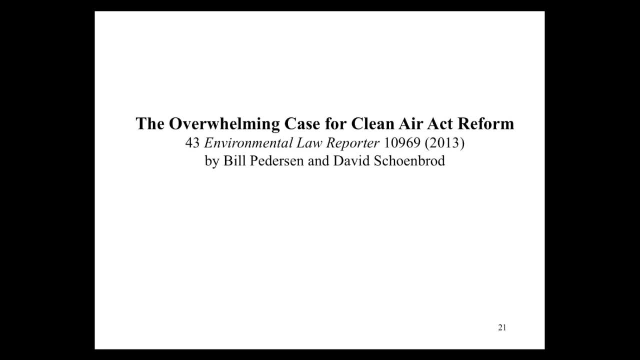 And we point out in that article, is that the clean air access we have today is built upon two false premises. The first one is that all air pollutants have. The first one is that all air pollutants have Safe levels. Muskie acknowledged, however, in 1977 that this is false. 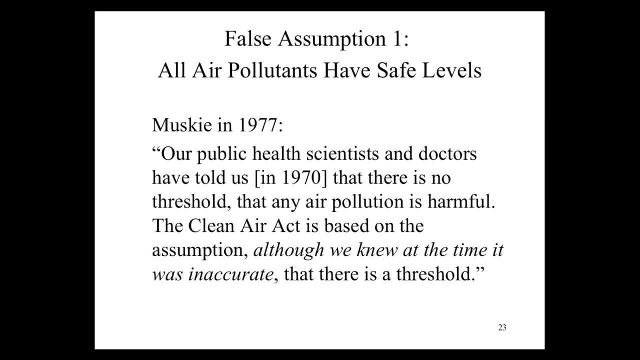 Our public health scientists and doctors told us in 1970 that there is no threshold, that any air pollution is harmful. The Clean Air Act is based upon the assumption- although we knew it at the time, it was inaccurate- that there is a threshold. 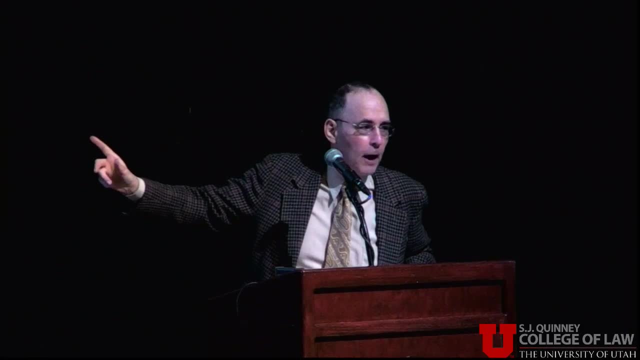 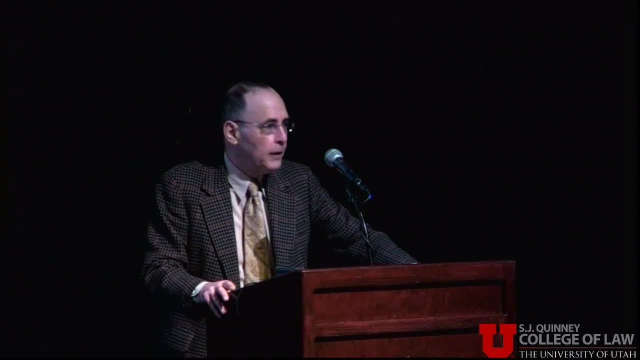 My mother had a word for that type of talk, Called a lie. Okay, Okay, Now This lie. let legislators pretend that they had made the hard choices by instructing EPA to set an ambient air quality standard to protect health, without regard to cost. 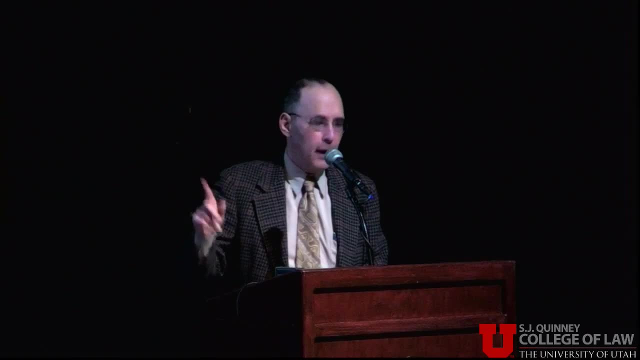 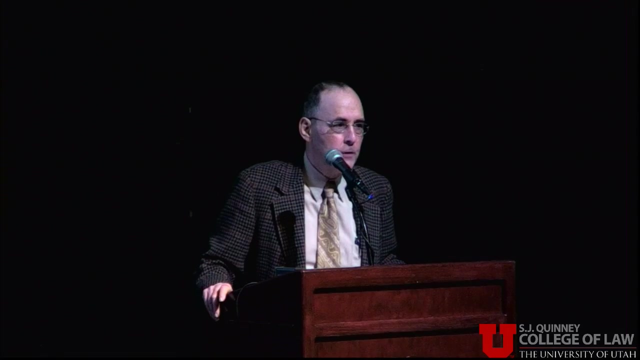 This instruction is gibberish because the only safe level is zero for many pollutants. Zero is impossible literally to achieve, And getting even close would freak out the most eco-friendly legislators because of the costs involved. So in setting national ambient air quality standards, 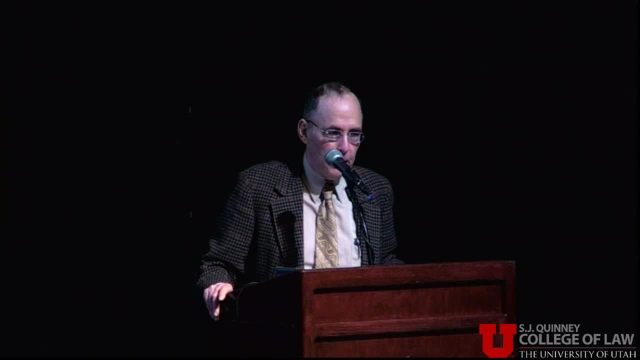 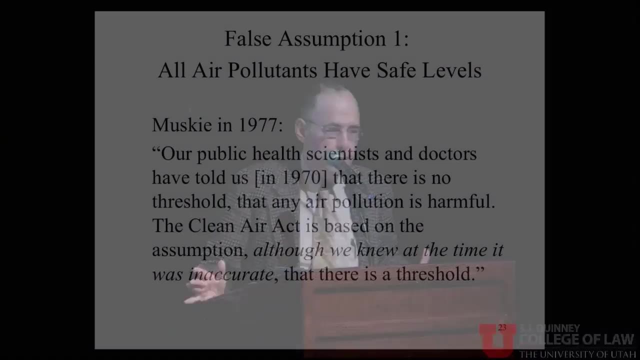 the EPA must lie, It must claim that it is ignoring costs when it really is, because that's the only way it could figure out what to do that makes sense. And so what it does is it sets the standards not on the basis of protecting health, but what's publicly feasible. 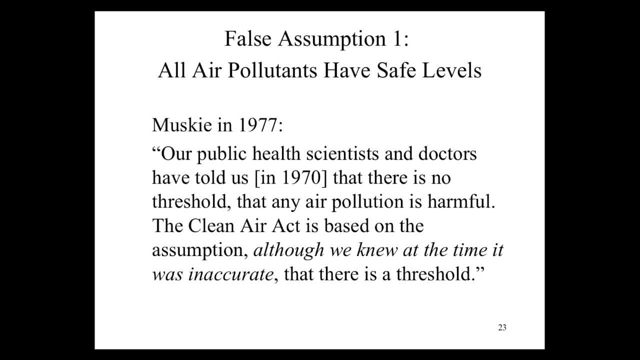 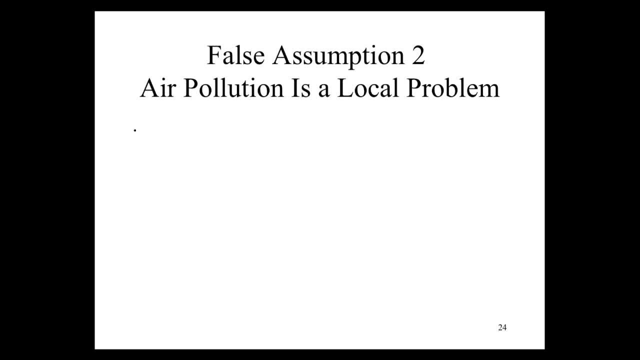 You're doing that to make me feel better, Okay. The second false assumption is that air pollution is basically a local problem. Yet, as we all know, the lion's share of the most dangerous pollutants are regional or international in origin, not local. 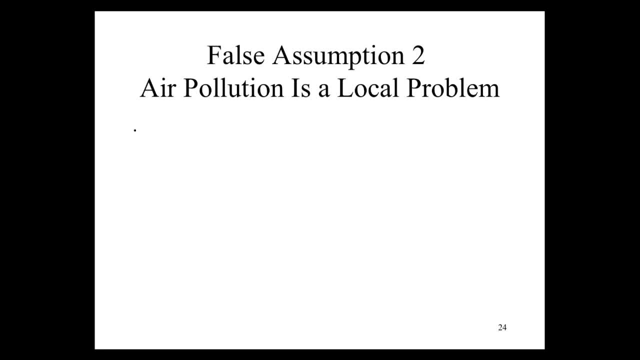 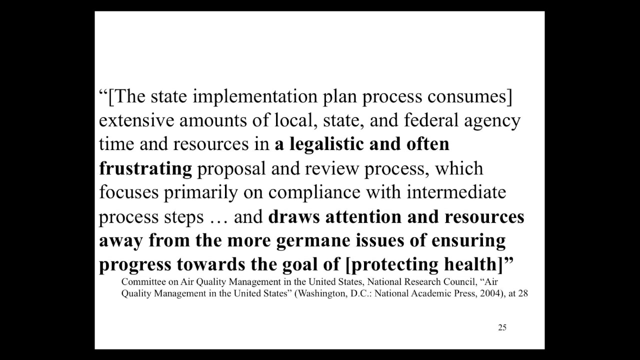 But this false assumption. let Congress take credit for announcing healthy air and then put the blame for not achieving it on state and local officials. Pretty neat if you could work it out. Meanwhile, however, the false assumption makes cleaning the air less feasible. This is a statement from the August National Research Council pointing out that the state implementation plan process is a bureaucratic mess. 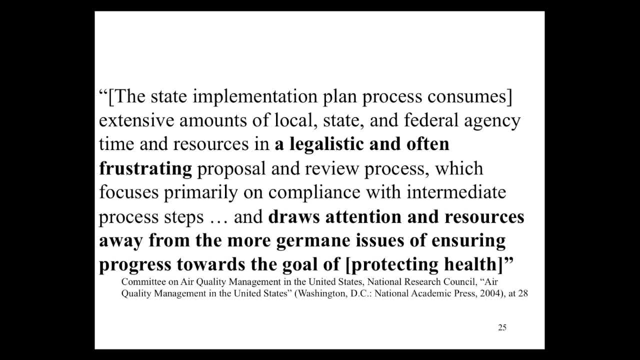 Distracts from the real job of cleaning the air, protecting our health. So compare this bureaucratic mess. So compare this bureaucratic mess With the emission limits on acid rain that Congress itself imposed in 1990 using the old way. Yeah, That's the acid rain program, the one with the lower left hand. 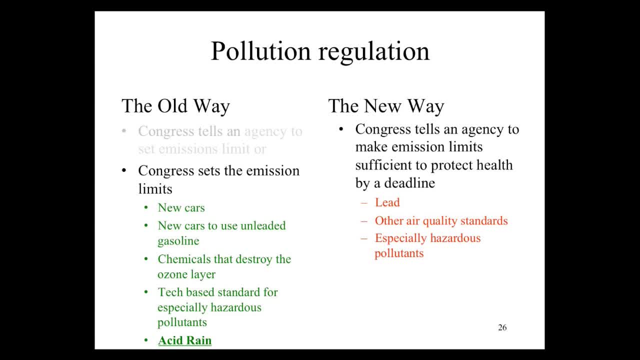 Okay. It achieved its 50 percent reduction target on time. We didn't need state plans or bureaucracy because it used. cap-and-trade Is run by fewer than 50 EPA staffers, Not like the State Implementation Law. the EPA cheered us up over here. 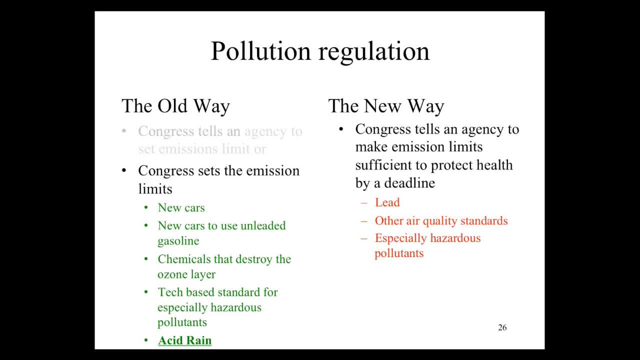 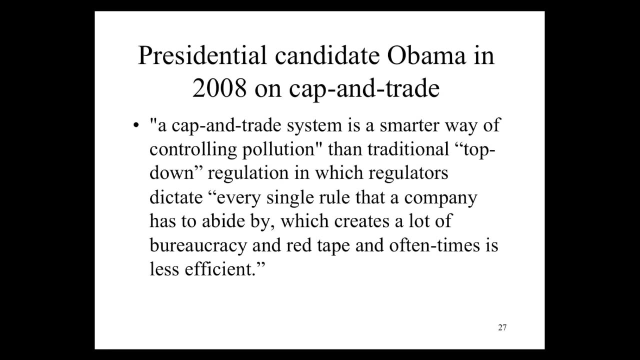 plan process requires thousands of EPA and state staffers to run the thing And, according to Barack Obama, speaking in 2008,, cap and trade is smarter, he said, less bureaucratic and more efficient. Now, under President Clinton, Bush II and Obama, EPA has worked hard and ingeniously. 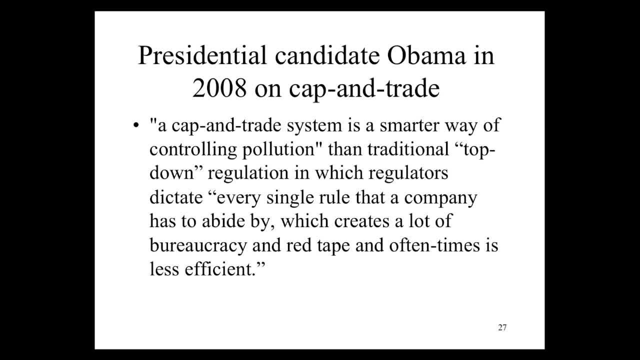 to impose cap and trade through the state plan process. but backfitting it into the state plan SIP process is slow and cumbersome and fraught with legal dangers. Sometimes EPA can work its way through, sometimes not, but it's slow and a mess. 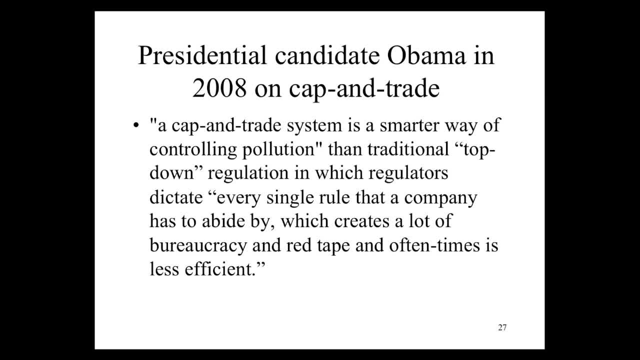 To make cap and trade work well, we need new legislation Now. it's perfectly feasible for Congress to apply something like the acid rain program to the largest stationary sources. We need to get rid of pollution, please. Richard Stewart, former chair of the Environmental Defense Fund. Katrina Wyman, his colleague. 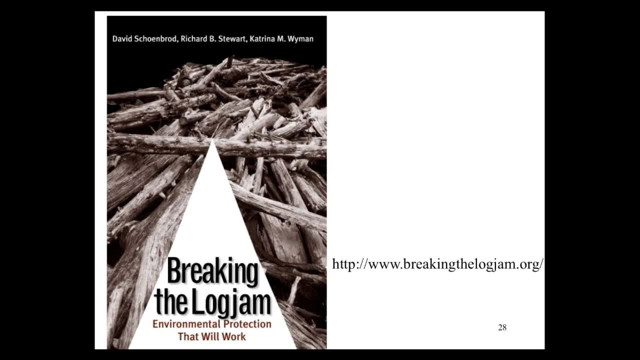 on the faculty of NYU Law School and I showed how in our Breaking the Logjam Project, there's our book up there- how to do this If you want to actually not buy the book, which is fine by me, but get our free report. 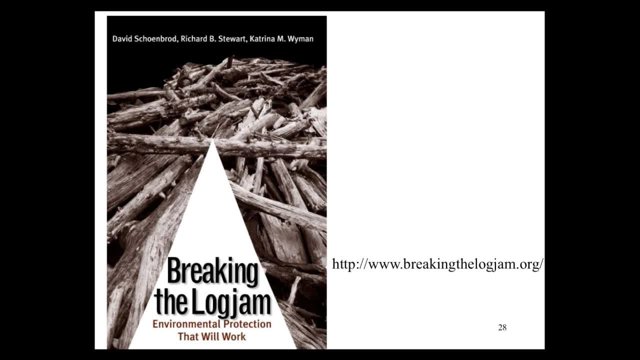 this thing here. it's on the website there, the link on the lower right. Okay, With such a reform, Bill Peterson and I estimate we could cut the most important conventional pollutants far more than EPA could using the current statute. so much more so that there. 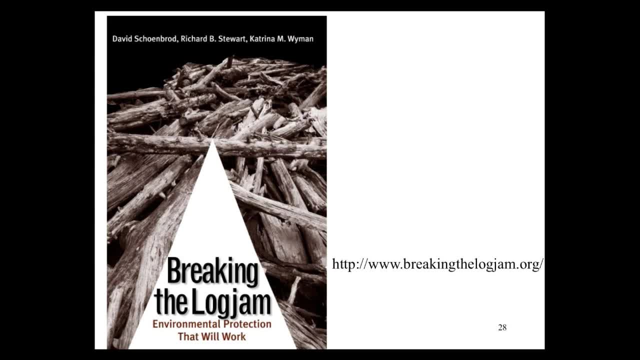 would be huge health benefits and a cost that is modest in comparison to the benefits and at a cost far lower per unit of pollution reduction than could be achieved with the current bureaucratic mess. Okay, Now Dick Stewart and I went around with this report, went around Capitol Hill and talked. 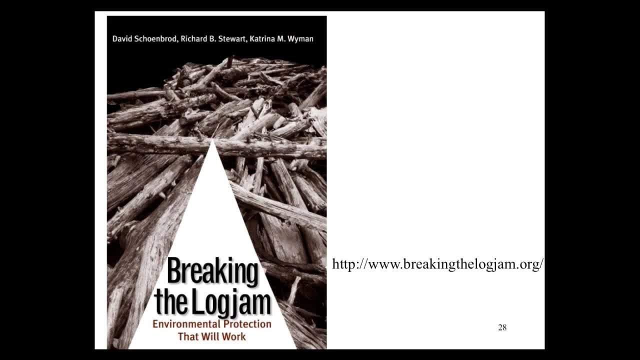 to all kinds of Democrats and Republicans about it and you know what they told us. They said it makes sense. We wish it were the law. You know it's not going to be the law. And why? Why won't it be the law? 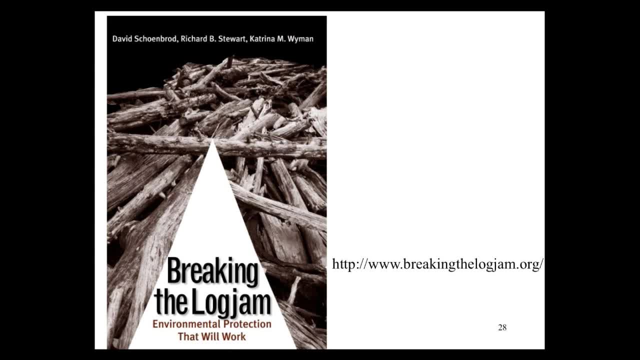 Why won't they do anything about it? Well, partly, it's that the current regime allows legislators to blame the EPA and the states for all the problems. Right, It's perfect for them. We're not responsible for everything. We mean the best for you. 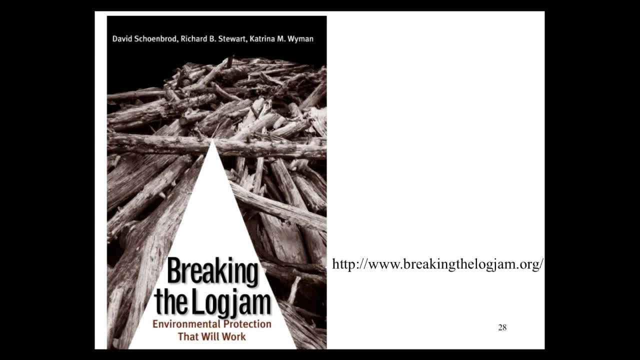 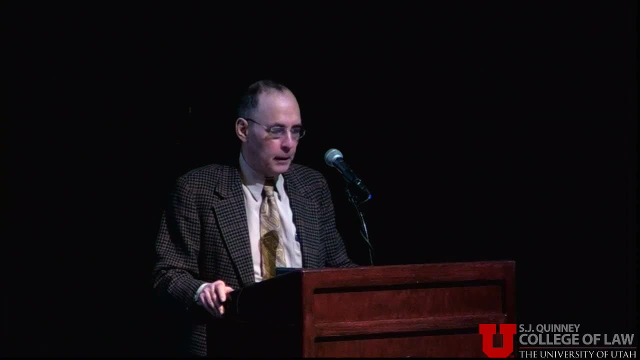 We want to save your jobs, We want to protect your health, It's just great, Okay, But it's not just them. The old approach also benefits other people whose jobs, income or power come from it, And there are a lot of jobs, a lot of income and a lot of power that comes from the current. Clean Air Act. Okay, Just to see why, Think of the legal fees, the headlines in newspapers and other payoffs that come from running this system. I read the old Clean Air Act in 1971 in about an hour. The current thing is 450 pages long. 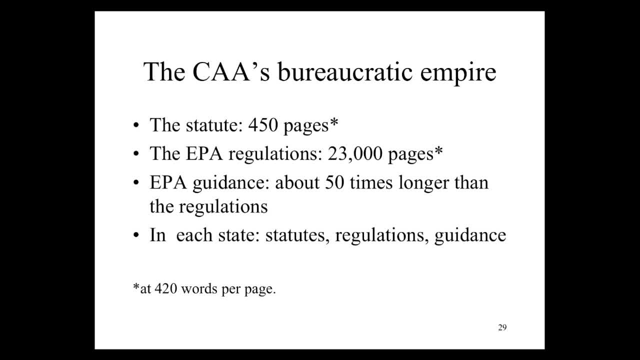 There's 23,000 pages of regulations about. There's about 50 times as much EPA guidance document, which you'll ignore at your peril. Right, Right, Right, Right, Right, Right, Right, And every state has their own version of all this stuff. 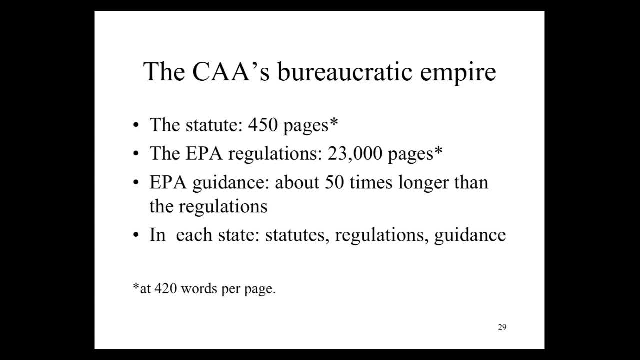 So what we got with the Clean Air Act? the Clean Air Act has done some really great things. I'm all you know. I'm grateful for it. I mean, today in New York City I could leave my window open and the window sill does not. 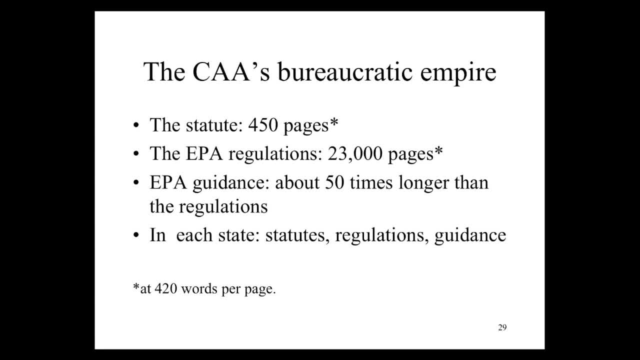 get black, It's great, But Peterson and I estimate that we could add another half year to the life of the average American with the type of approach we're talking. if only the people in Congress, if only the in the government would take some responsibility. 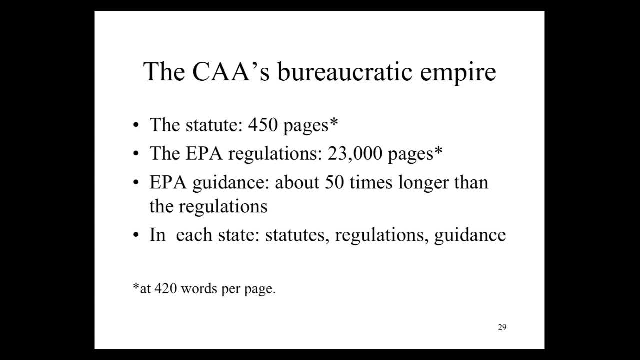 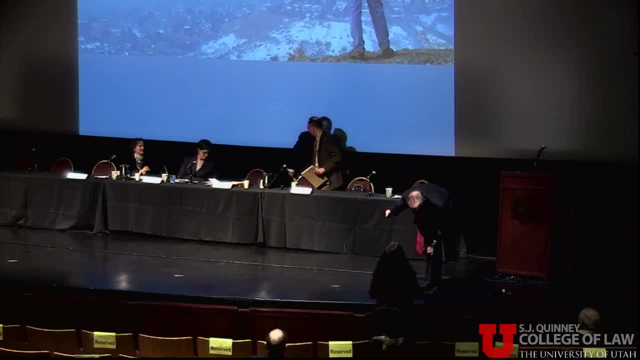 If only the people who are privileged under the current regime look to the public interest and look to the not to the public interest, And then we can go into a little further into the time there. But we've been here a lot and looking this way and looking at it quite a bit. 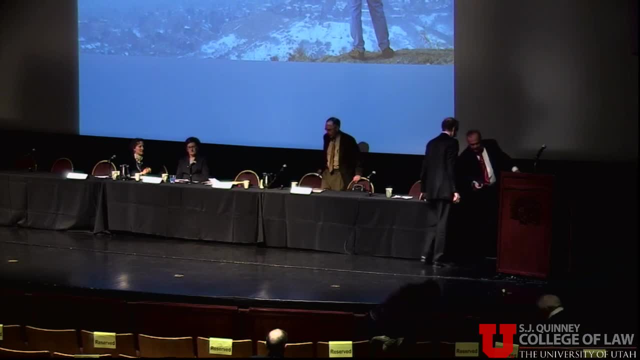 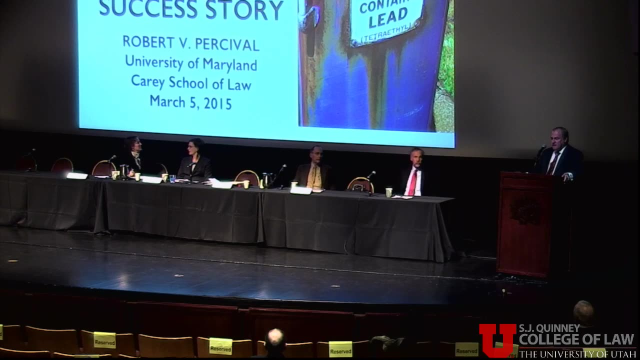 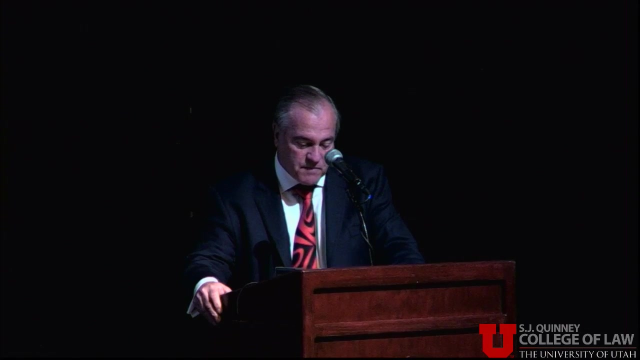 And one of my706, you know we were two years ago when we decided at that gift we probably don't want to have a brand. And one thing I would add is that I don't care if you don't get paid. Yesterday in the Stegner lecture, I discussed the long struggle for clean air in the United States and the current global dimensions of that. 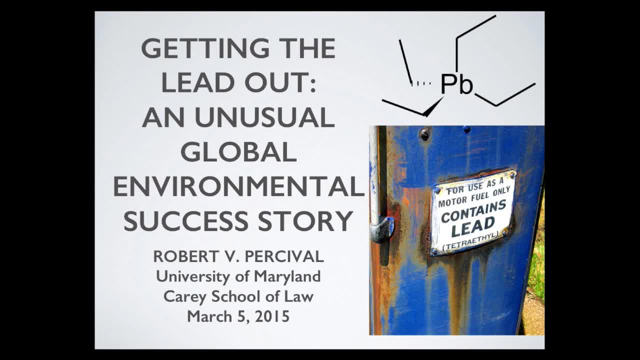 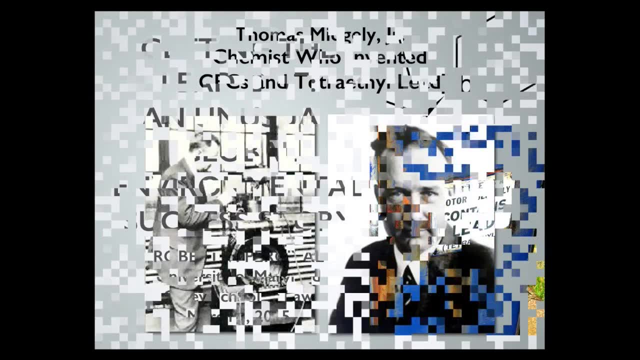 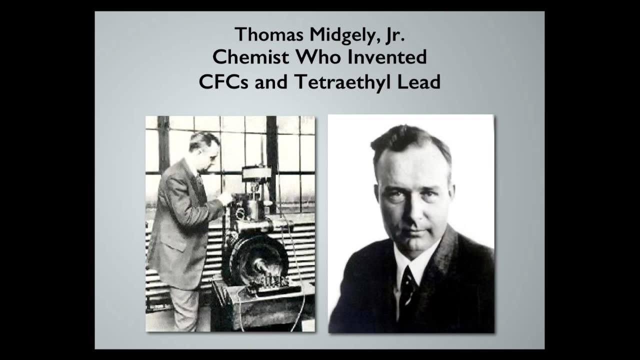 And I gave a general overview about the history of lead and gasoline, which David just discussed as well, And I mentioned that I would go into it in more detail today. It really starts in the 1920s, when this chemist, Thomas Midgley, invented both chlorofluorocarbons and tetraethyl lead. 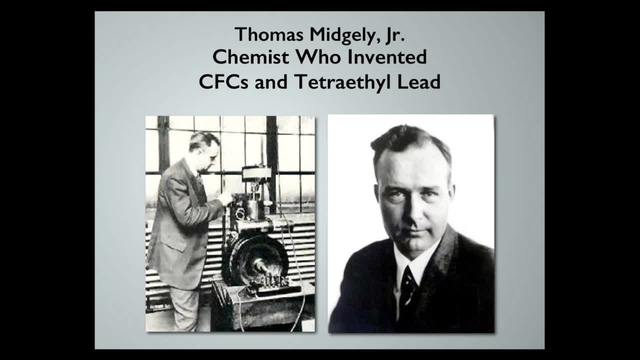 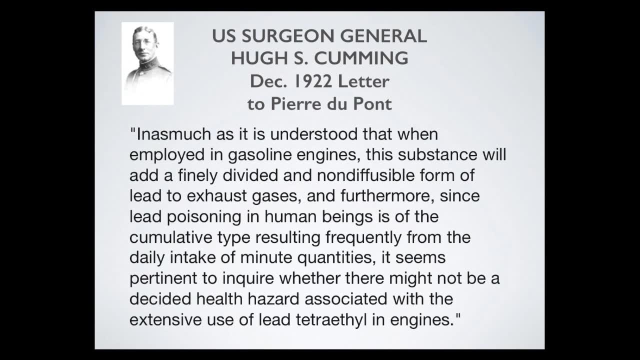 Tetraethyl lead as a cheap way to boost octane in gasoline, But there were immediate public health concerns about it. The Surgeon General in 1922 followed the logic of some of the public health officials who said: if we're putting lead in gasoline, it will get into the air. 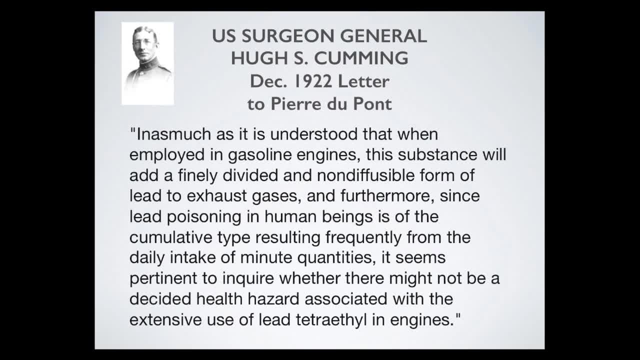 It will If we increase lead exposure. we already have a lead poisoning problem. We should investigate this. And after several workers died at a tetraethyl lead manufacturing plant in New Jersey, the Surgeon General in 1925 called this conference. 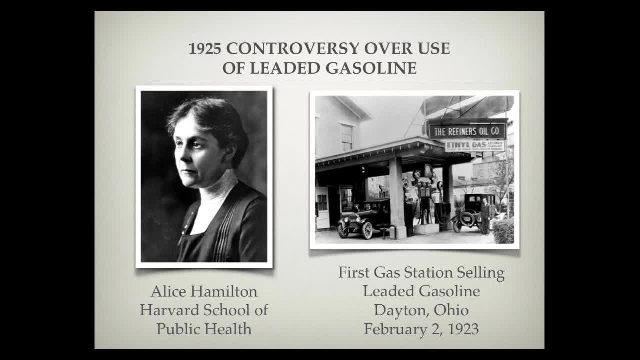 At the time, we didn't have national environmental legislation, So the way of dealing with public health problems was: let's get all the experts together, And several cities had banned the sale of leaded gasoline. What the experts decided to do was they decided to do a quick six-month study where they compared the health of workers and chauffeurs. 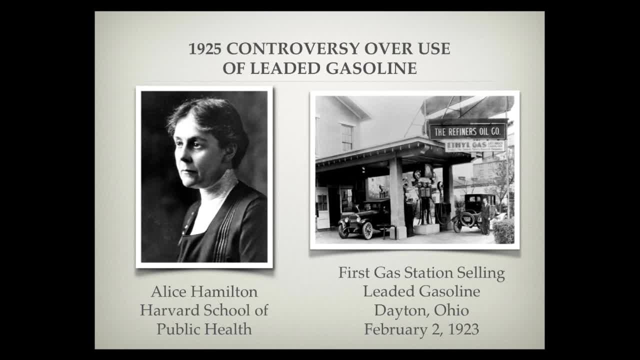 who used leaded gasoline or unleaded gasoline. They didn't see any visible differences, so they decided to let lead and gasoline go on the market, Even though Alice Hamilton of the Harvard School of Public Health said this is going to, as more and more of this is used, it's going to build up in our environment and cause major health problems. 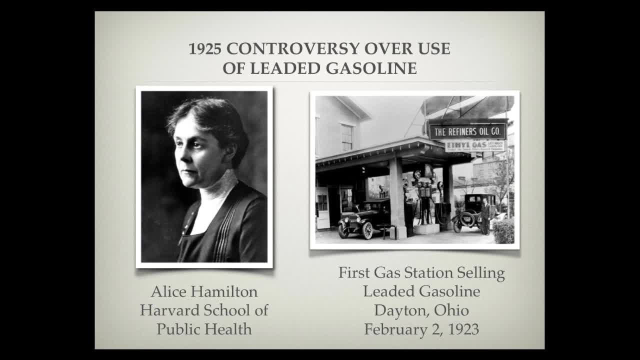 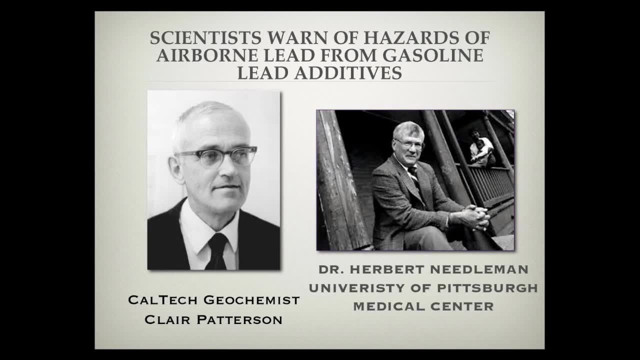 By contrast, the lead industry said tetraethyl lead was- quote- a gift from God. The Surgeon General in 1925 said the Surgeon General said we have to carefully monitor this over the next several decades. In the 1960s, Caltech geochemist Claire Patterson participated in these studies. 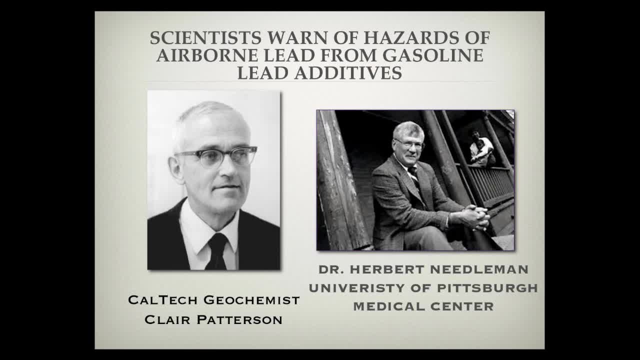 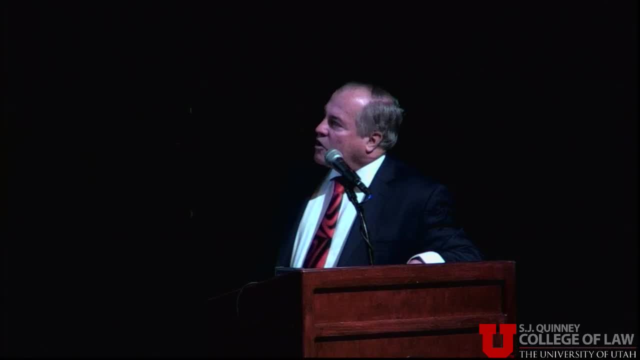 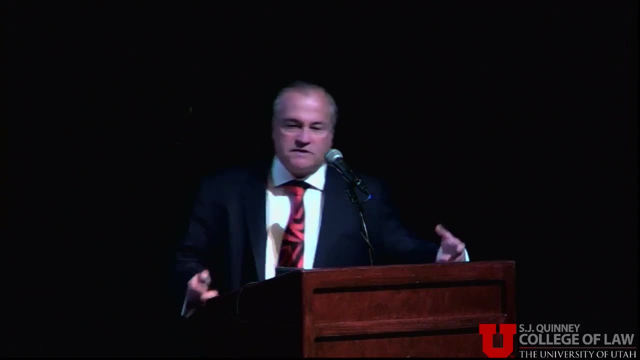 where they looked at lead levels in various cities and came to some alarming conclusions about the buildup of lead from leaded gasoline. A pediatrician at the University of Pittsburgh, Herb Needleman, collected baby teeth and found that the high lead children exposed to higher levels of lead. consistently increased their lead levels Consistently had lower IQs. Lead causes neurological damage And this caused a great deal of concern. When the Clean Air Act of 1970 was adopted, EPA was authorized for the first time to regulate fuel additives. that quote will endanger public health or welfare. 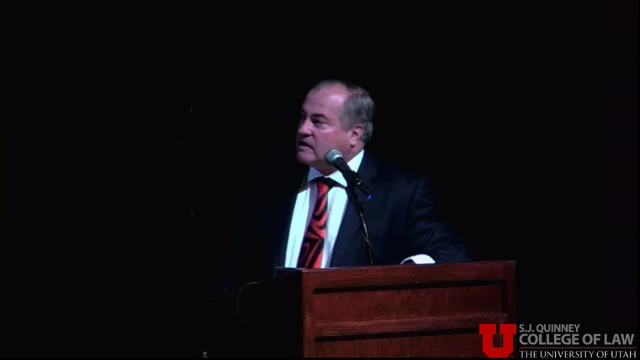 And that was directed in part at lead in gasoline. At the time there had been about an average of about four grams of lead per gallon. EPA then used that authority in part because of prodding from David and the Natural Resources Defense Council in some of the lawsuits that they brought. 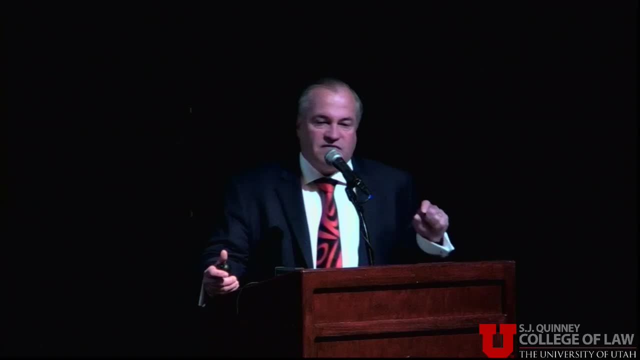 Initially, EPA announced we want to limit the amount of lead in leaded gasoline to protect public health. At the same time, of course, oil refiners are going to have to start making unleaded gasoline for the new cars because their catalytic converters 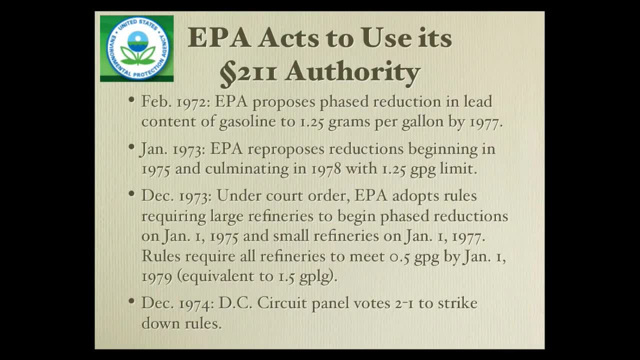 would be poisoned by it. EPA, finally, in December 1973, adopted these first regulations limiting the amount of lead in gasoline. but they also required that, to accommodate smaller refineries, that they'd not have to phase down the amount of lead in gasoline as fast. 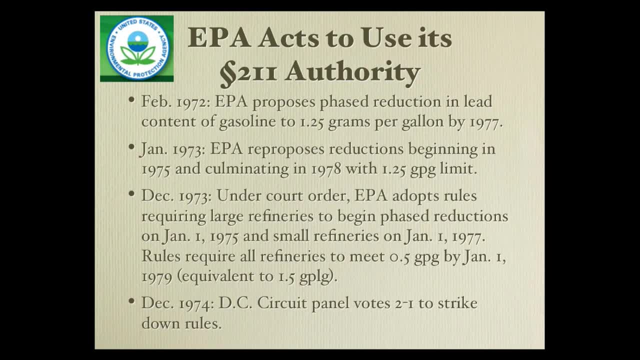 That was then challenged by the lead industry in court and in December 1974, by a vote of two to one, A three-judge panel of the DC Circuit struck down these regulations, saying the case against lead in gasoline was speculative and inconclusive because EPA couldn't prove that specific people 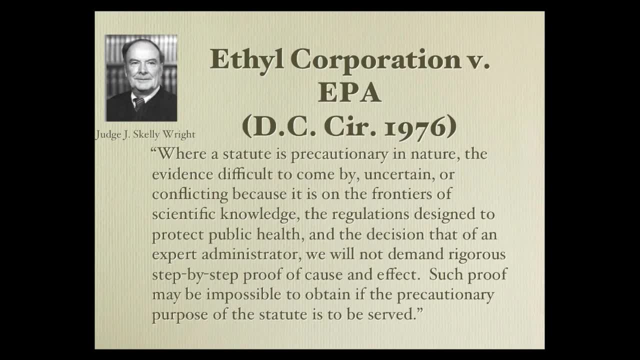 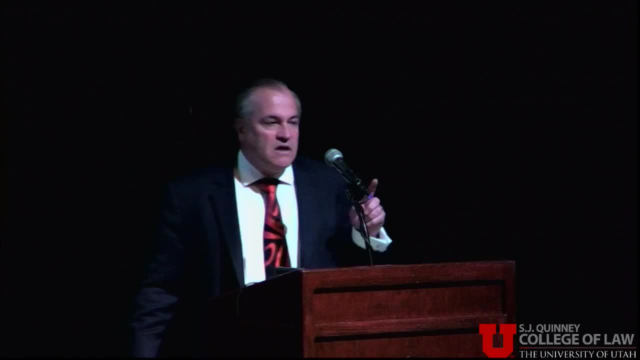 had been harmed by it. Fortunately, the DC Circuit took this case en banc. The full court reviewed the panel decision and, by a vote of five to four- a single vote in the Ethel Corporation decision- endorsed this notion of precautionary regulation. 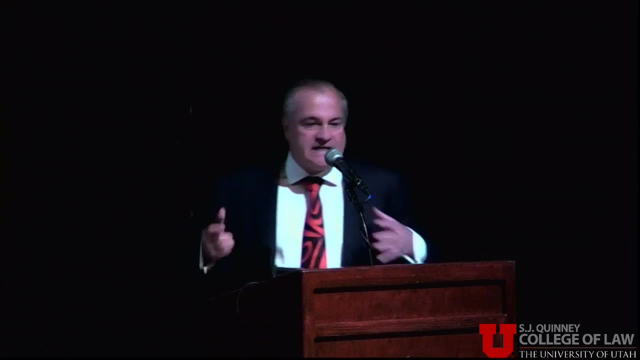 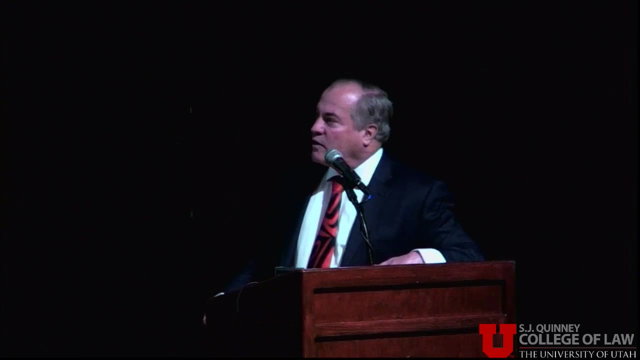 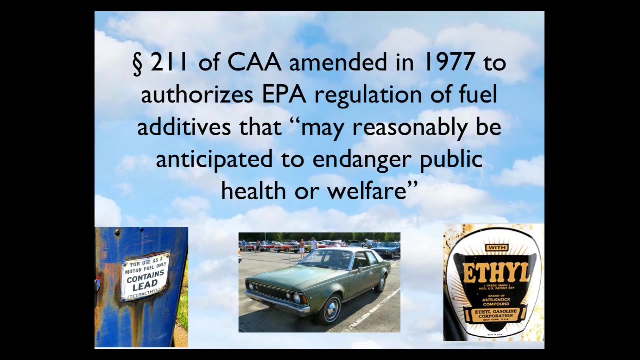 Amazing. It was a major precedent establishing that you don't have to show the kind of proof of causal injury that you would if you were bringing a tort suit. And in 1977, when the Clean Air Act was amended, the Congress changed the statutory standard. 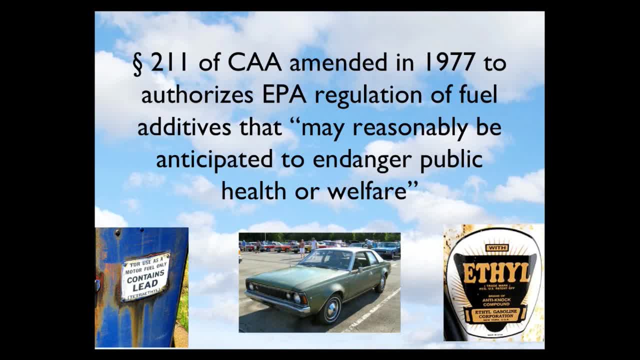 instead of will endanger to, may reasonably be anticipated to endanger public health or welfare, which some have said is essentially codifying the Ethel Corporation decision. Now, you recall, in the 70s, with the Arab oil embargo, we had a time when there were 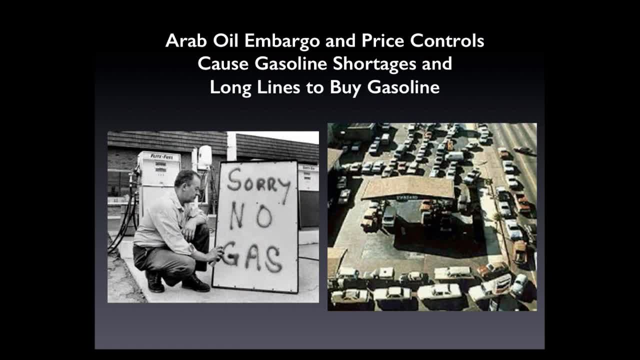 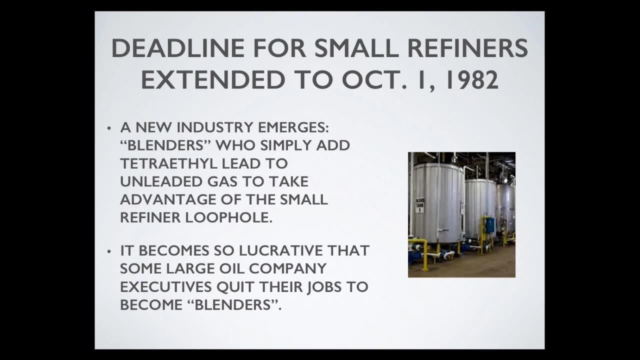 gas lines and gasoline shortages because we had price controls on gasoline, Not as much gasoline was being imported And this was exploited by the lead industry and the refiners to postpone the deadlines for raising down the amount of lead in gasoline. And in fact, for a while they said that, based upon how small a refiner is, they were not. 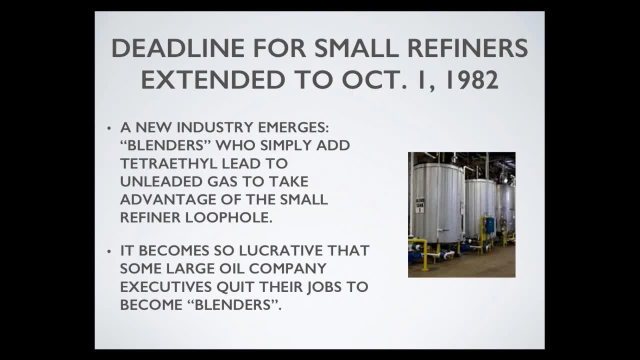 going to be able to get a lot of lead. That's not true. You could put more lead in your gasoline. It created an entirely new industry of what were called blenders. Some oil company executives actually quit their jobs with big oil and became their own. 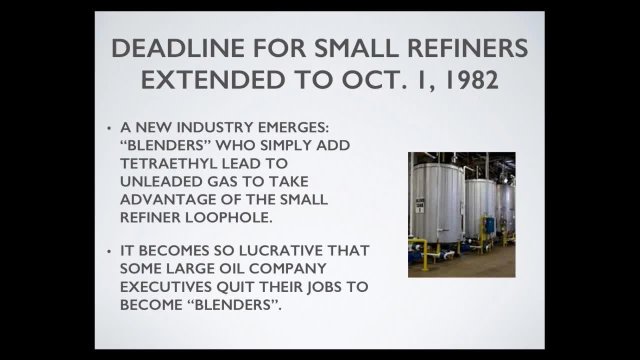 blenders, where they would just dump lead in unleaded gasoline And they could sell it at the prevailing market price. but it would cost them less to make the unleaded gasoline. So it was incredibly profitable And it was increasing the emissions of lead in the environment, despite the fact that there 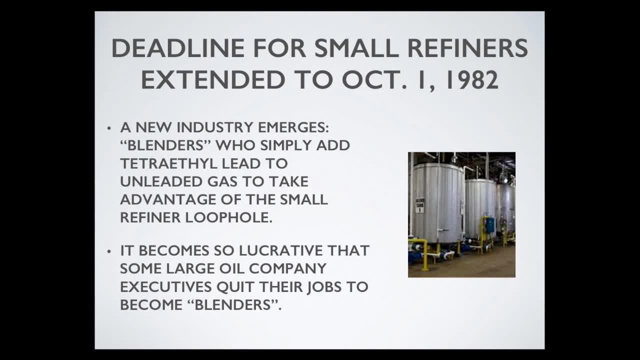 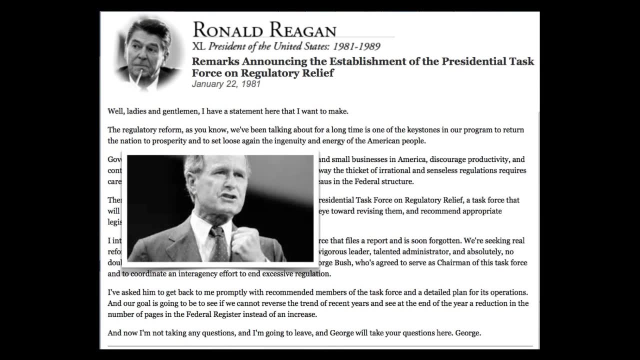 should have been this natural force, natural phase down when new cars took over more of the market. Then, when Ronald Reagan came to power, he created this Task Force on Regulatory Relief, put Vice President Bush in charge and the Vice President wrote to major executives about. 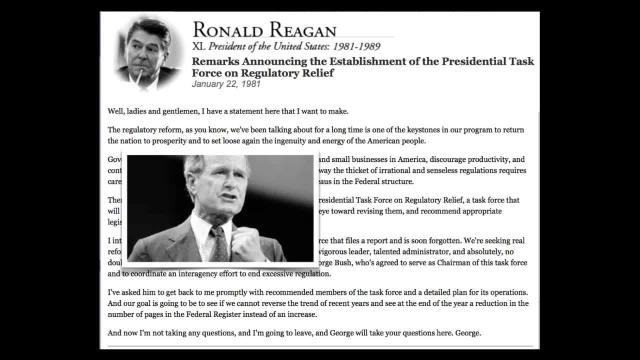 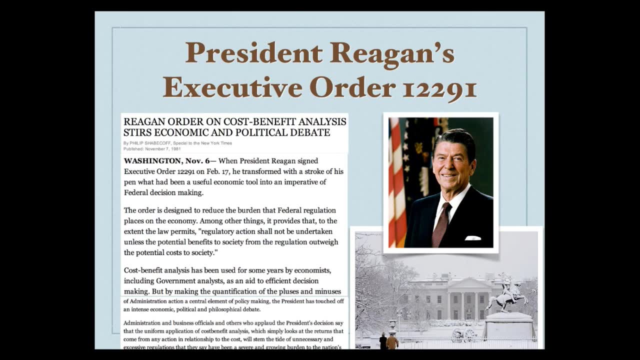 what regulations we should repeal. And since Bush was from the oil industry, his friend's most popular regulation was the limit on lead in gasoline. So the EPA was forced to propose to eliminate the limits on lead in gasoline, the logic being: well, eventually we'll all have new cars that run on unleaded gasoline. 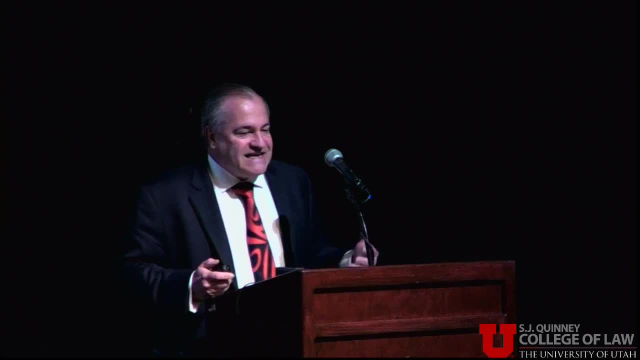 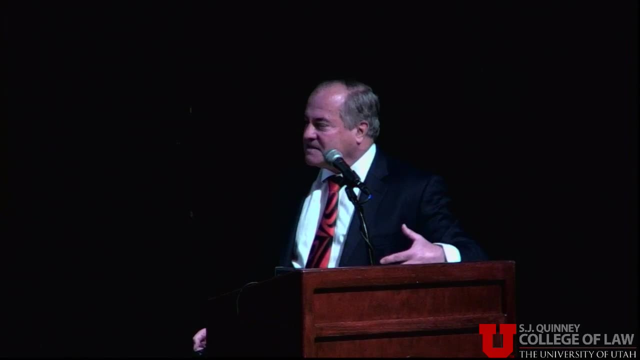 The irony here was that President Reagan had mandated that all regulatory changes, all new regulations, should be subject to cost-benefit analysis And yet, because they were proposing to repeal an existing regulation, they didn't do any cost-benefit analysis. I had argued at the time, as a young attorney for the Environmental Defense Fund, that this 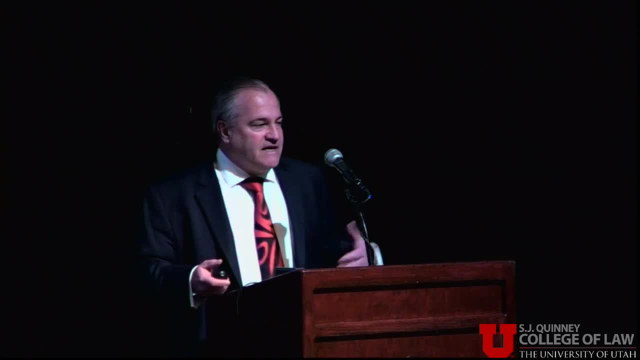 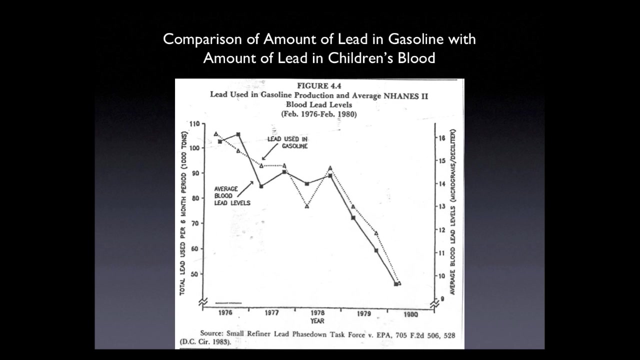 was crazy and hypocritical. If they did a cost-benefit analysis, they'd show that the savings to the refiners from repealing the lead regulation were tiny compared to the hundreds of thousands of children who would have increased lead poisoning. And yet that was ignored on the grounds that we're lowering cost to industry. so it's got. 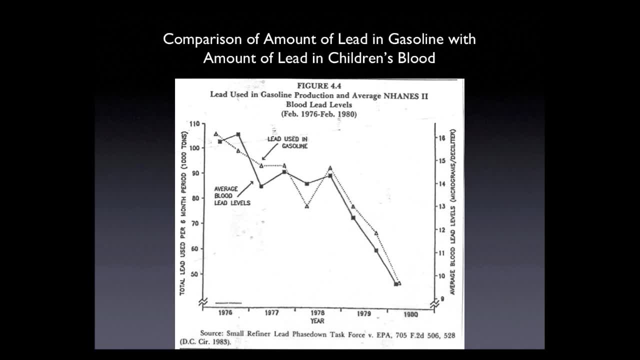 to be a good thing. One crucial thing that helped turn this proposal around was the end-to-end. The end-to-end study came out, which showed that over this four-year period- this five-year period where they were studying the health of Americans- they had found this tremendous. 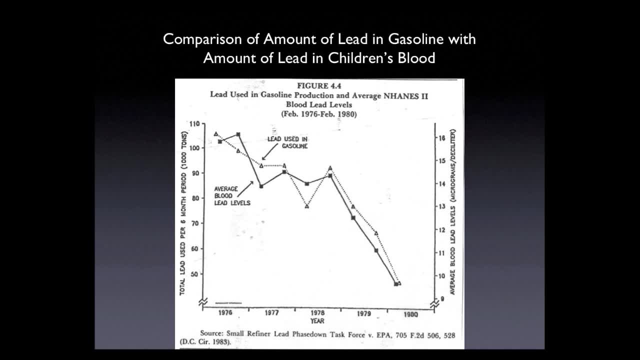 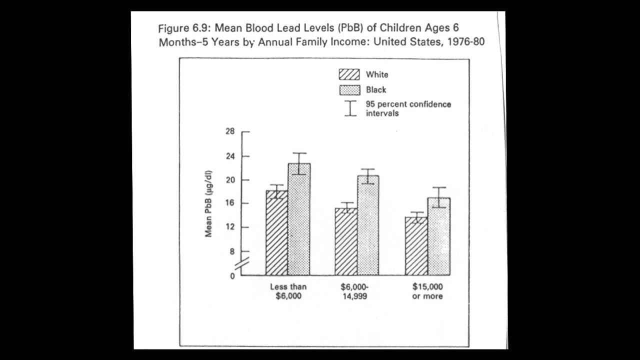 decline in levels of lead in children that was associated with the natural decline that was starting to occur because of more cars burning unleaded gasoline being on the market. The data also showed that there were substantial environmental justice problems where, even if you controlled for income or geography, minorities had higher levels of lead in their 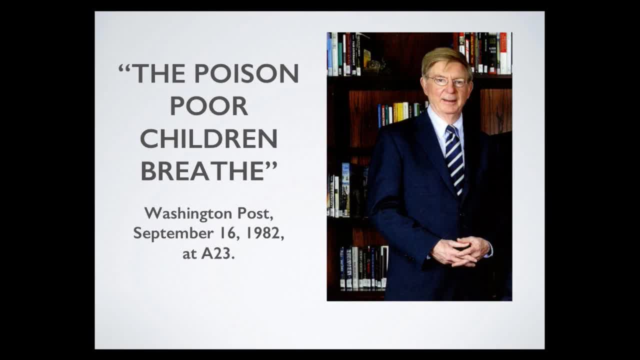 blood than did the white population. One of the crucial heroes here- and this is so ironic today because he regularly demonizes environmentalists- was the columnist George Will. He wrote a column called The Poison Poor Children Breathe, He said we conservative Republicans are supposed to be in favor of equal opportunity, but how? 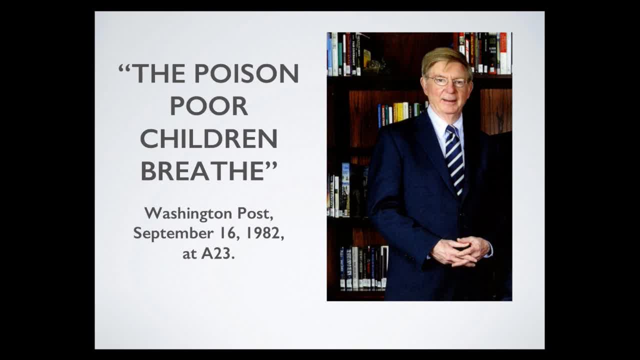 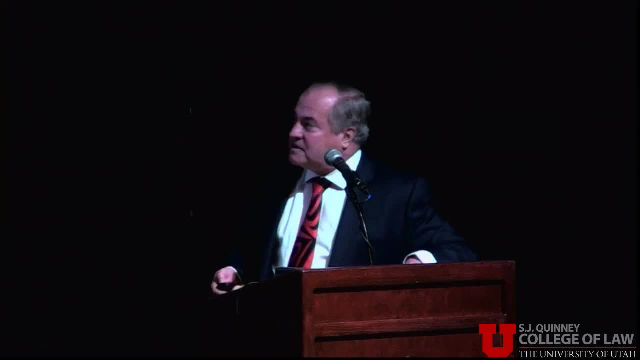 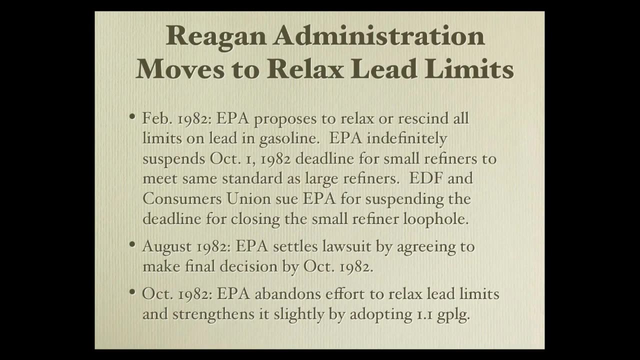 can you— We say that opportunities are equal if poor and minority children start their lives with higher levels of lead in their blood that do neurological damage to them, That helped turn the White House around as well, And so EPA had initially proposed to relax or rescind the regulations. 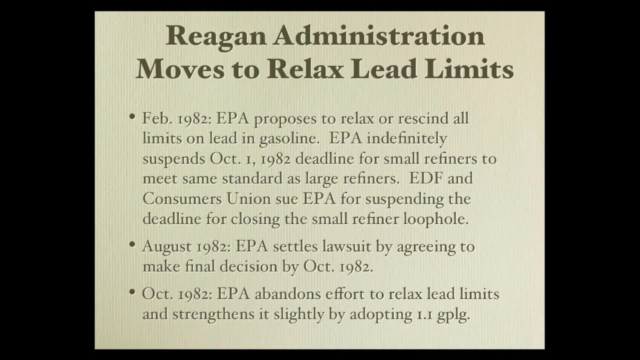 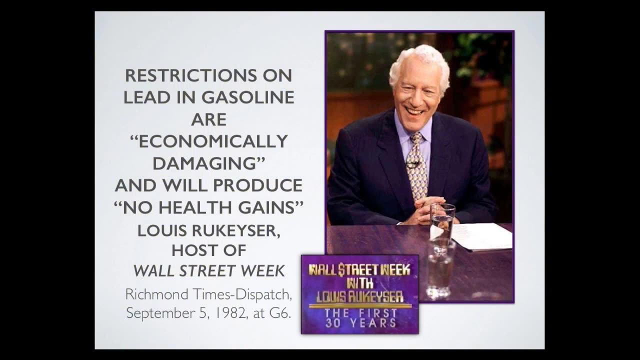 They suspended the deadline for the small refiners and blenders to come into compliance. We then sued EPA. We reached a settlement with them where they agreed to a final decision before the 1982 elections, And then, in October 1982, they abandoned this effort to relax and they actually strengthened. 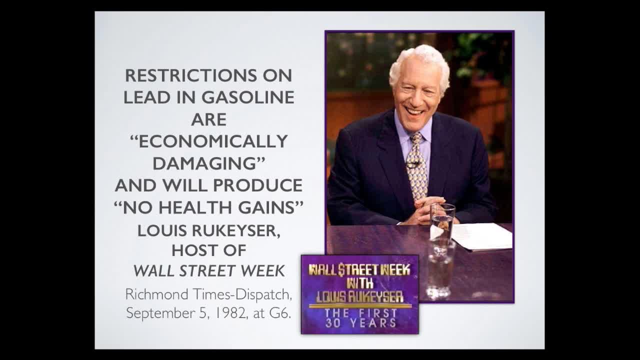 the regulations a little bit, because they adopted our idea of: instead of regulating on a pool-wide average of all gasoline a company produced, which would allow you to jack up lead levels in the leaded gasoline as you produce more unleaded, they instead limited it to the amount of leaded gasoline you produce. 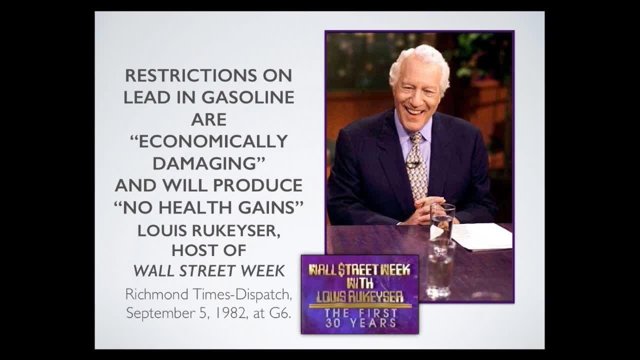 Now, of course, This was, as I mentioned yesterday, decried by some commentators. Louis Rukeyser of Wall Street Week said this is going to be economically damaging and produce no health gains. The Wall Street Journal ran an editorial that pooh-poohed the problem of lead poisoning. 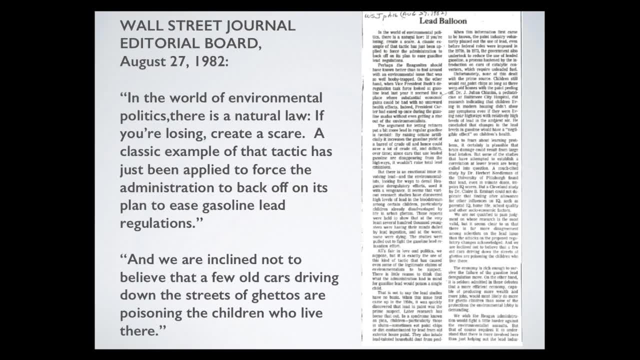 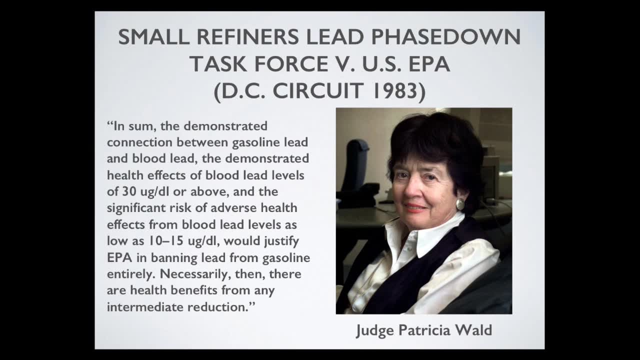 from gasoline and concluded that the worst thing about this was that the Reagan administration had caved in to those environmentalists. The small refiners then challenged the case, the decision in court to make them—and of course they did— make them comply. 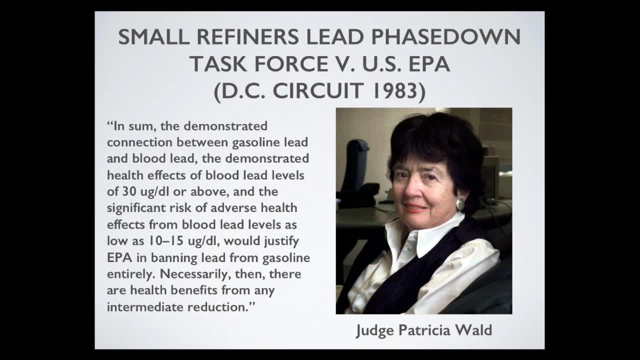 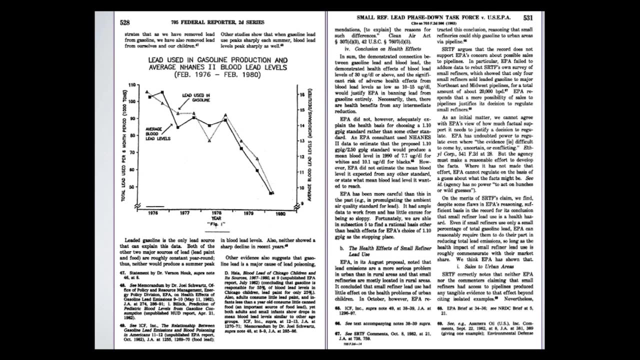 And this was really odd- bedfellows, because Exxon and some of the big oil companies who hated the small refiner loophole actually joined us in court in supporting what EPA had done. Nevertheless, the court ended up giving the small refiners more time, But I did the oral argument in this case and I was admonished by Judge Wald for spending. 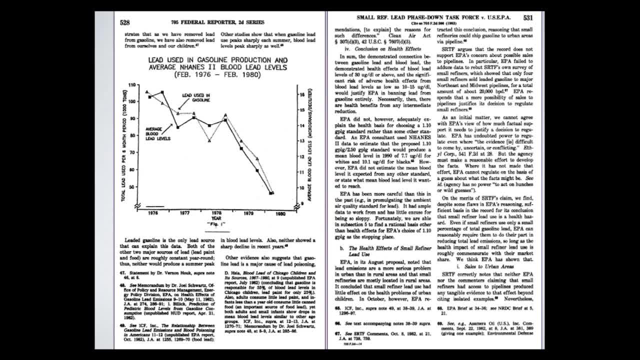 too much time in my argument stressing the incredible damage to public health that lead was doing. But what— But what later happened? in her opinion she included the NHANES 2 chart and she actually said we can't understand why EPA is allowing any lead in gasoline at all. 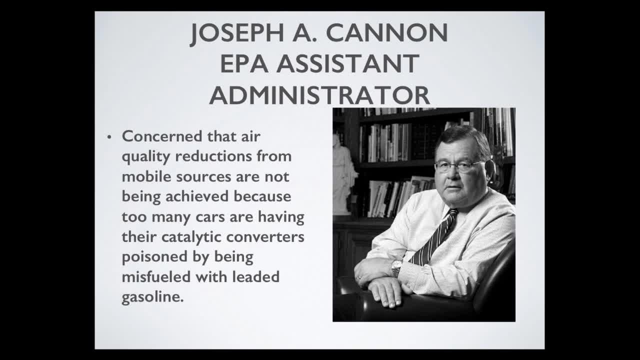 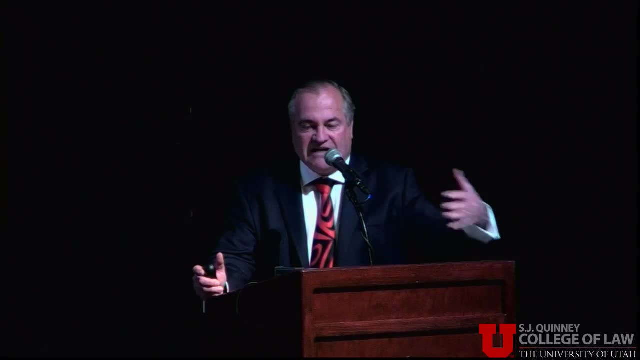 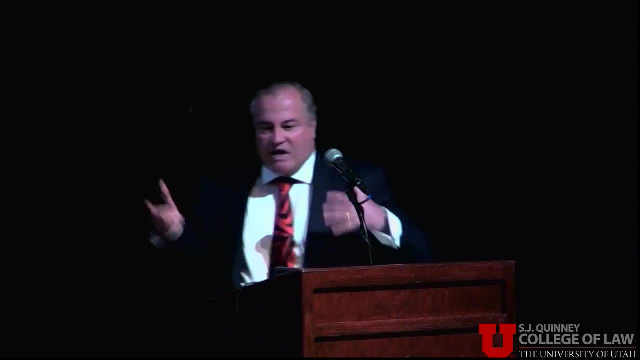 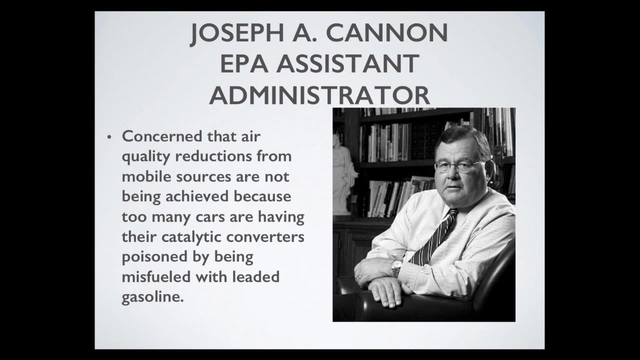 gasoline, which killed their catalytic converters. so EPA was not getting the emissions reductions from the tailpipe standards that it had expected. So what we pitched to EPA was: you can solve the misfueling problem by just getting rid of lead in gasoline. 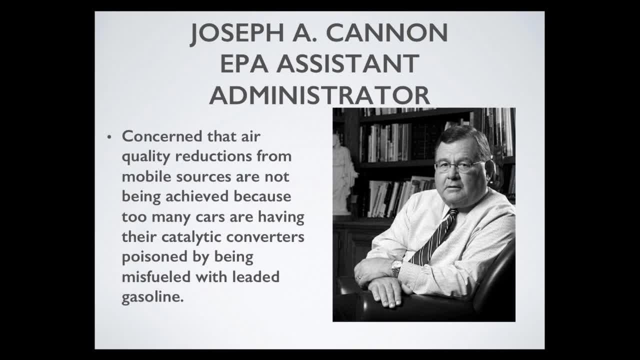 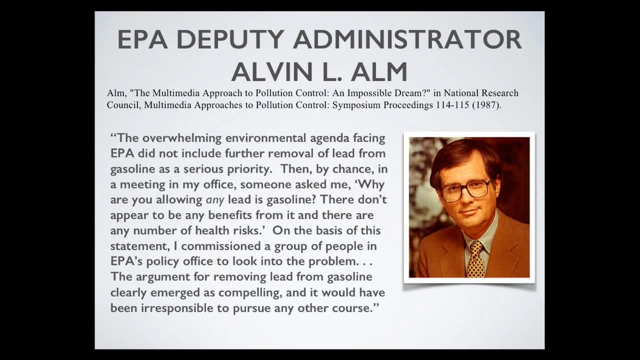 Then you won't have to spend so much time on the politically controversial inspection and maintenance programs. I once had a meeting with Al Alm where I pitched the notion of why doesn't EPA do a cost-benefit analysis? the Reagan administration is supposed to like that of getting rid of lead in gasoline. 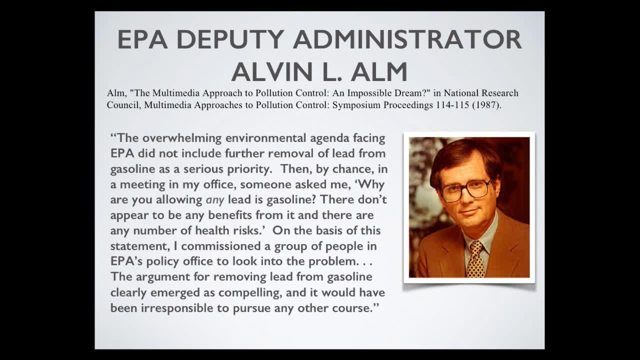 You'll find that there are overwhelming net benefits. It wasn't until years later when he wrote this article in a National Academy of Sciences proceeding where he said the weird thing about how EPA sets priorities is the phase-out, ultimate phase-out. It occurred because someone said to me one day: why don't you do a cost-benefit analysis? I can't say for sure- it was me, but EPA then did a cost-benefit analysis. Their epidemiologist, Joel Schwartz, played a major role in this. He discovered some really great data sets that allowed EPA to show that there would be enormous net benefits from phasing out lead in gasoline entirely. 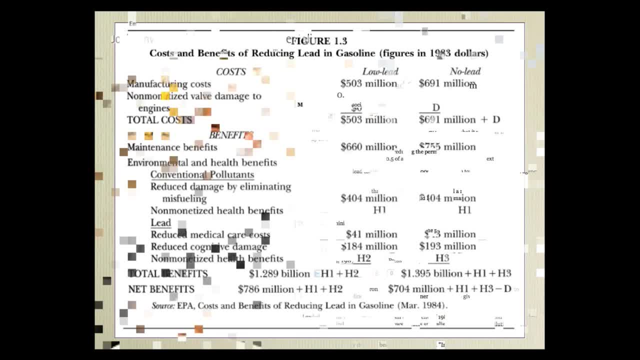 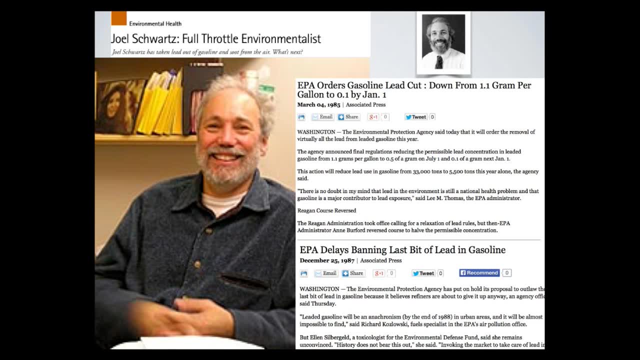 Ultimately, what EPA decided to do to placate the cost-benefit analysis- they decided to go with the IPD, not EPA- was to lead one-tenth of a gram of gallon of lead in leaded gasoline because of the concerns of OMB that older cars would be damaged because of their valve. 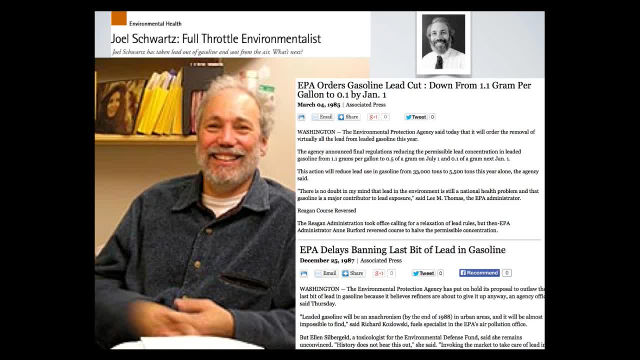 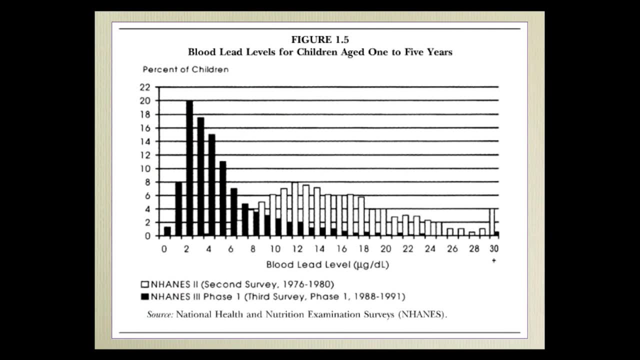 seals being damaged, even though Schwartz's analysis proved that, if anything, it was going to be just the opposite. Finally, what EPA did Congress in 1990? Clean Air Act Amendments simply banned the use of leaded gasoline. It was not ersten. 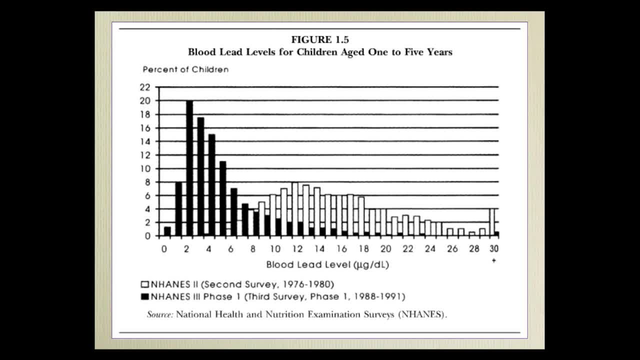 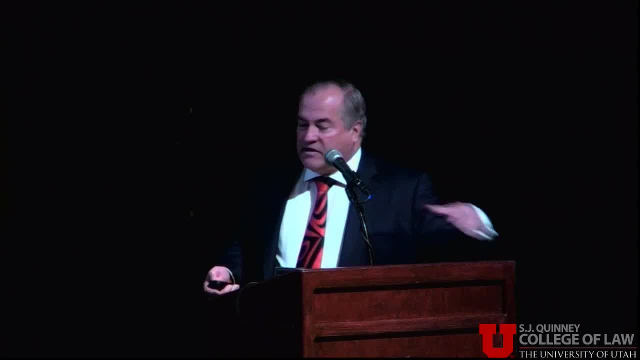 It was the first time, uh, that EPA was over the line of use of leaded gasoline in a two-year time, 1996.. So now we've gotten rid of lead in gasoline. The results have been totally dramatic in reducing lead levels in children in the United States. But the other aspect of the story that I mentioned, 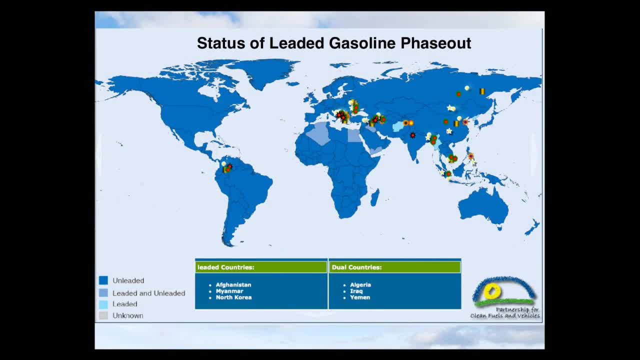 yesterday is other countries have followed suit. The US took the bold initial move. Sure, it took a long time, as David emphasized in his talk, But now virtually every other country in the world- the only leaded countries entirely- are Afghanistan, Myanmar and North Korea. 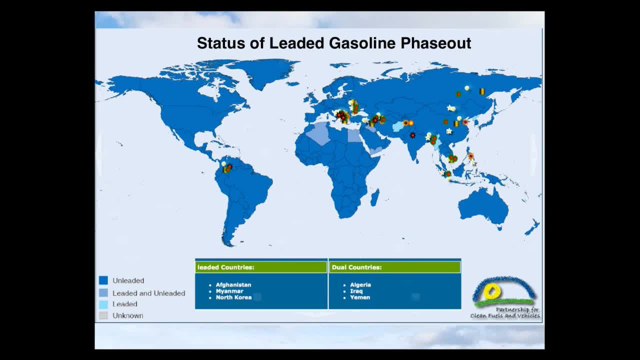 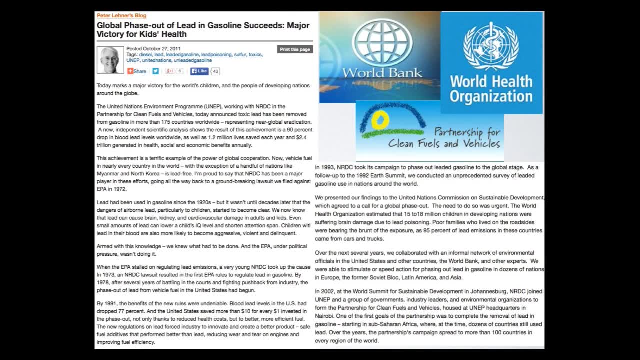 today, They realized the enormous health benefits. In part, this was due to NRDC and other environmental groups, networking with the World Bank, the World Health Organization and the formation of the Partnership for Clean Fuels and Vehicles, And the latest cost-benefit analysis of 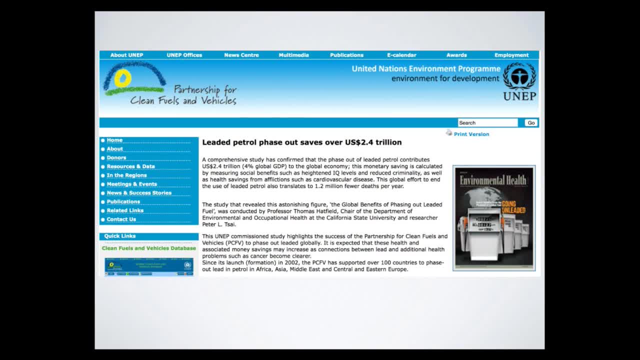 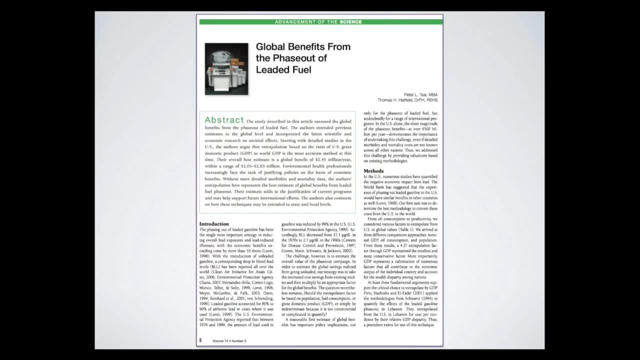 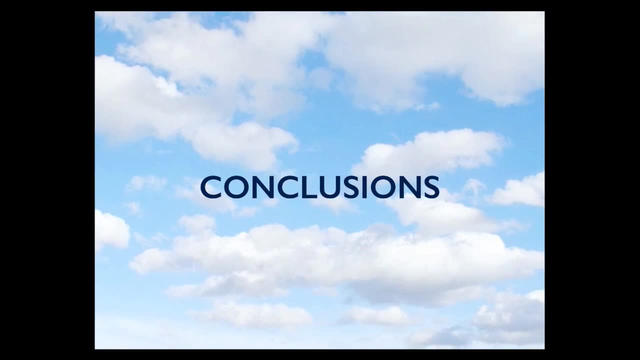 the global ban shows that it actually has produced net benefits to the world. In fact, the World Bank has produced net benefits to the world of $2.4 trillion by phasing out lead in gasoline around the world. So conclusions First. this whole history, I think, illustrates one problem. 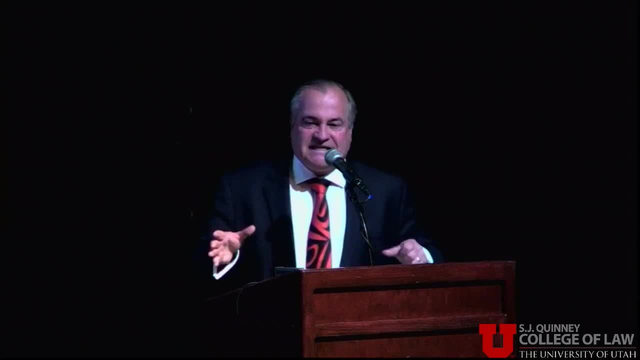 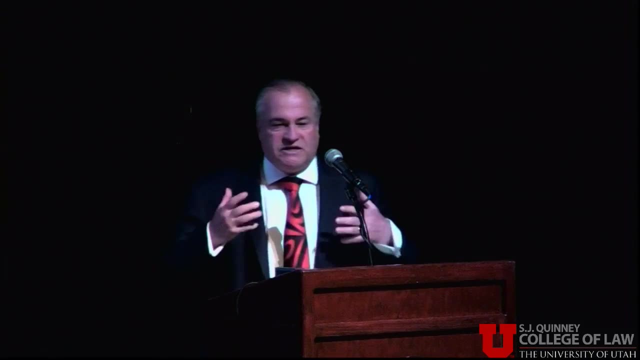 in environmental law We like to respond when there's a big disaster, something really visible, an oil spill or something, But we have a much harder time dealing with chronic, less visible health problems that occur, and that's part of the whole history of lead. 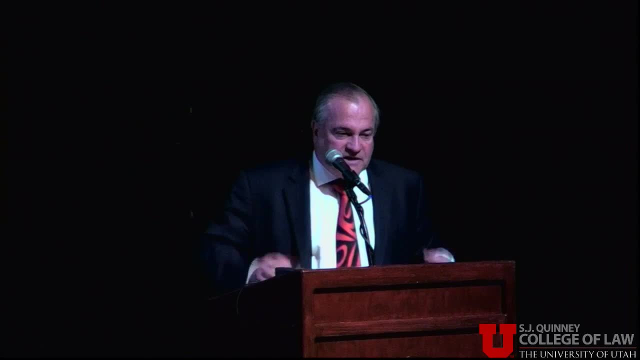 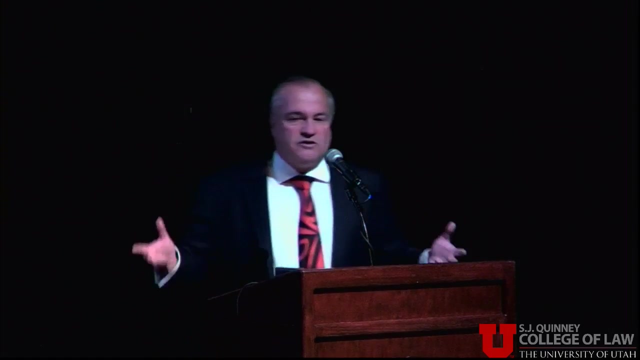 Also, it illustrates the strategic behavior by the regulated industry. Whenever there were debates on should we lower lead levels in gasoline, the lead industry, the gasoline industry, would say: it's all a problem of lead paint. When we'd have debates over what to do about lead paint, they'd say: it's all a problem of. 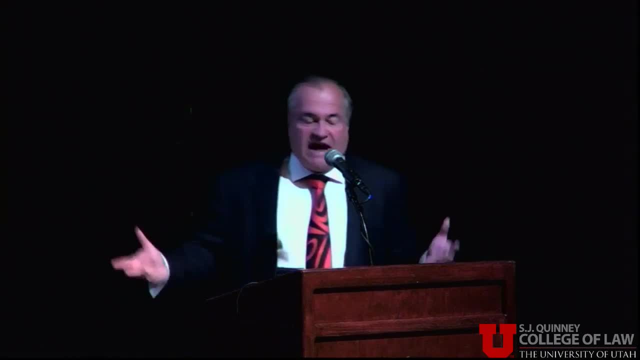 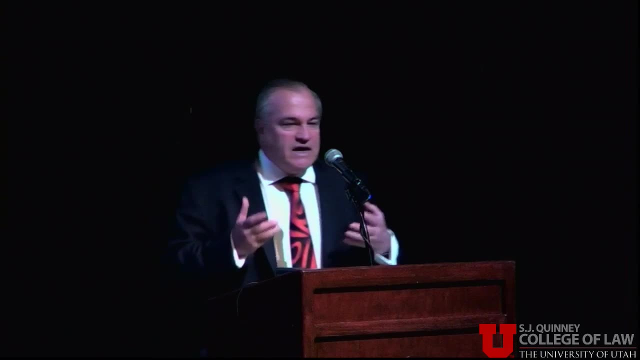 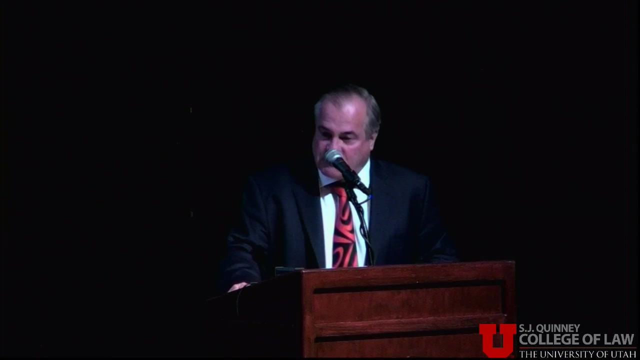 leaded gasoline And they would also say we're going to have gasoline shortages. it's going to harm the economy. people will be out of work. That stuff happens all the time but, as I showed in my talk yesterday, whenever we've resisted and not given in to those people who are crying wolf, the result has been 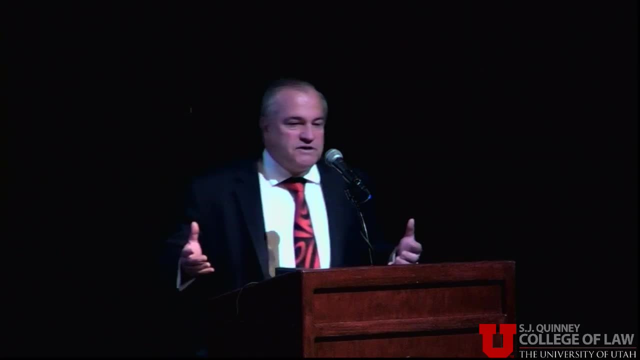 dramatic improvement in public health. This also shows that the importance of individuals and NGOs playing a role in interacting with the regulators in order to get environmental progress. It illustrates the danger of allowing a politically popular loophole. People were concerned about those poor small oil companies and the 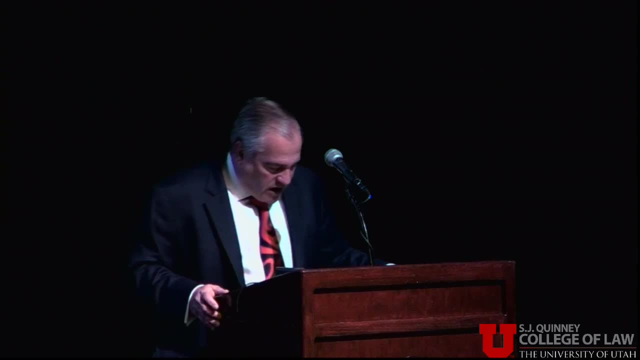 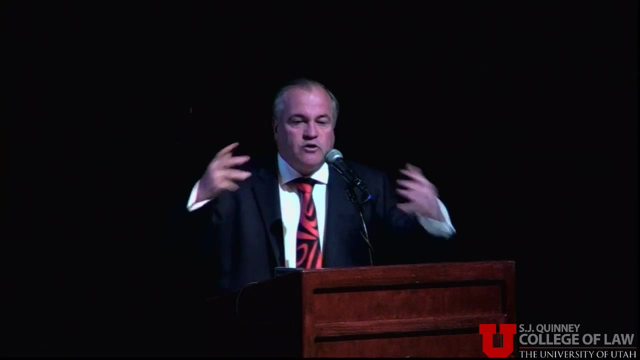 regulation of the oil industry was not a good idea, So we've had a lot of problems with that. The result was that lead use was greatly prolonged. And finally, it illustrates the wonderful new phenomenon in environmental law, and that is the globalization of these environmental networks that has meant that countries can 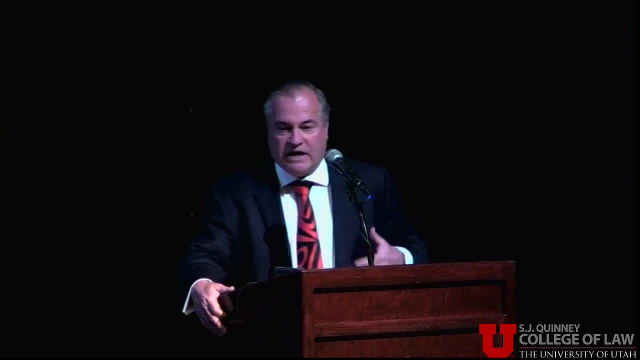 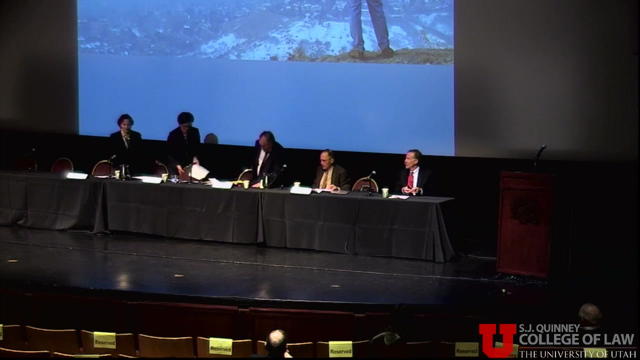 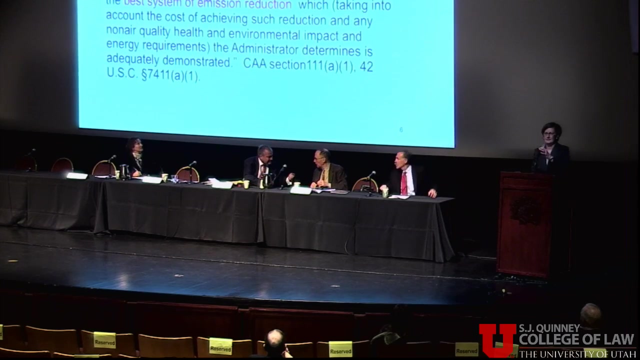 learn from each other and borrow regulatory innovations from each other so that now, as clean air has become a global imperative, the planet is living in largely a world that's free from leaded gasoline. Thank you, Good morning. You've just heard two very interesting perspectives on. you know the 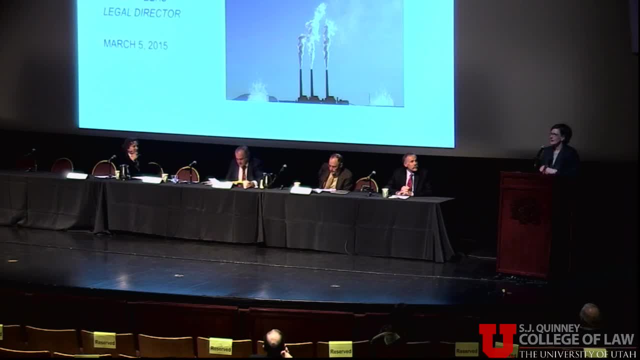 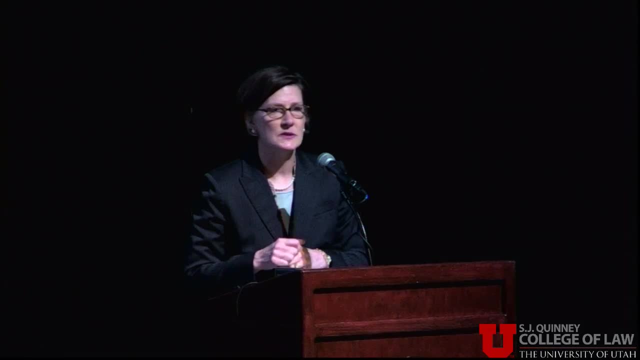 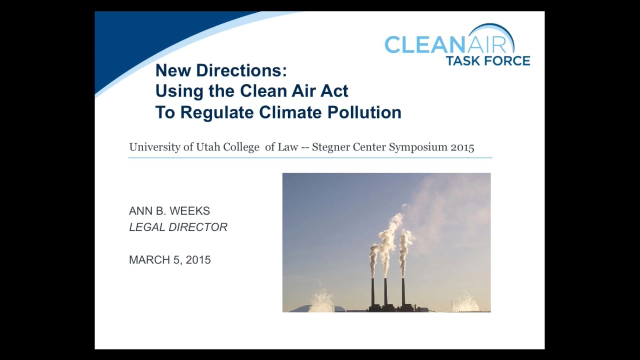 history of one portion of the Clean Air Act in its early days to the present and the benefits that the Clean Air Act has been able to achieve. I'm coming at this from the practitioner's perspective. I work for an environmental nonprofit and I'm 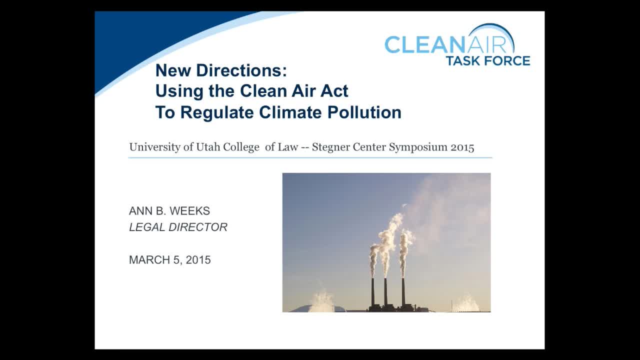 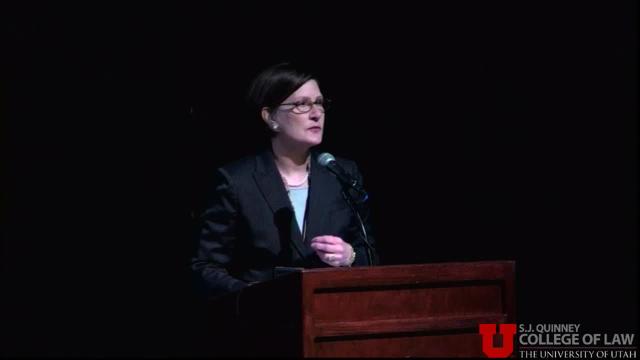 interested in where we go next and that my talk is the new directions. I'm, in a way, giving you some background on the clean air act and I'm really excited to be talking to you about some of the things that the Clean Air Act has done for the 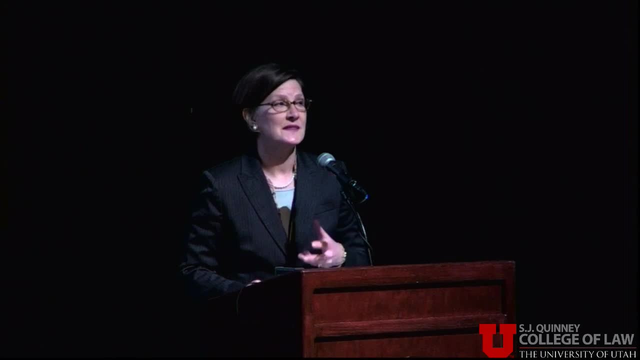 planet. I think I'm sure that if I could just jump around for Jody Freeman's keynote address, I think she's going to take this and do, I'm sure, a far more elegant and eloquent job that I'm going to be able to do this morning talking to you about where she sees the court going. I'm going to give you a little background on how we got where we are and what we're doing right now. One of the very powerful things about the Clean Air Act: from 1970 through the amendments in 1977, through the 1990 amendments, all along the 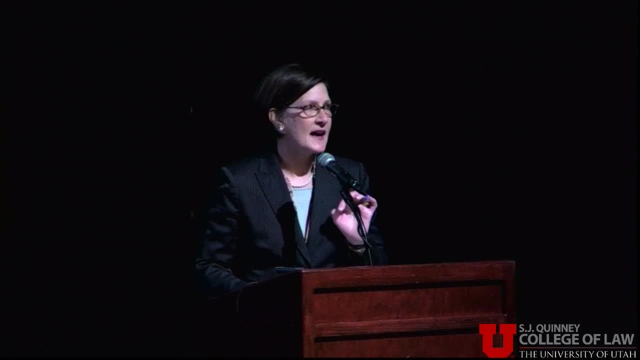 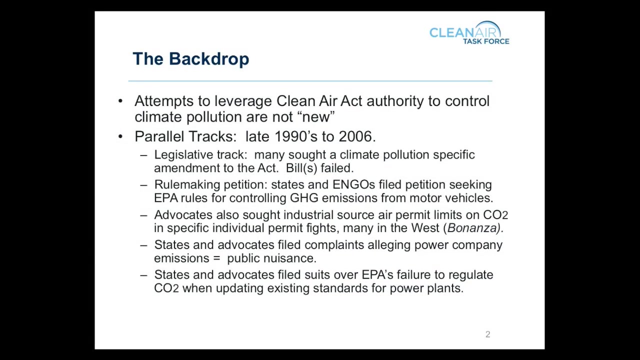 way is the degree to which this statute offers the opportunity to press for change. There are citizen suit provisions in the act. There are rulemaking, very specific rulemaking, directives. The public has a real opportunity to leverage change using the statute. I want to start by saying that, although my talk is new dimensions and new directions, 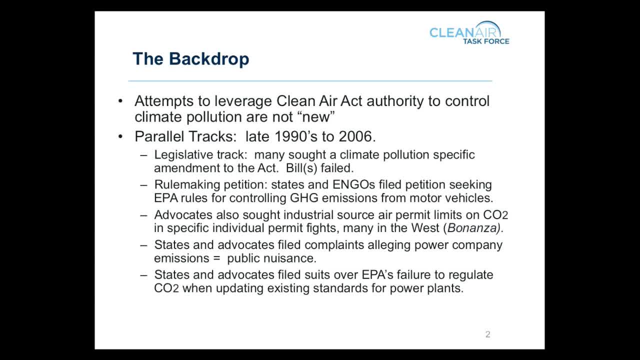 attempts to use the Clean Air Act to regulate climate change are not, in fact, new, in the sense that, although they're hitting the paper now, they've been going on for a long time, From the mid to late 1990s to 2006,. there's been a lot of change. 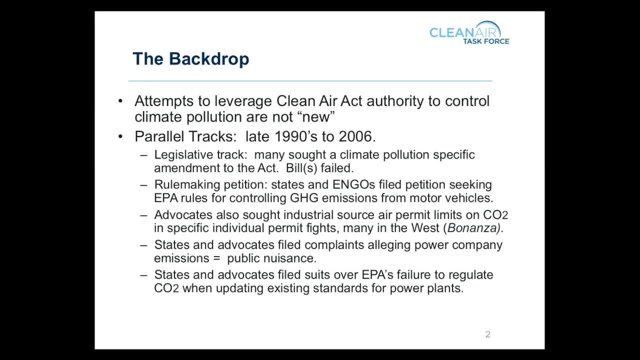 In 2006,. we had several parallel tracks going, and again this is the power of the Clean Air Act. There was the legislative track When Congress was considering economy-wide controls on pollution that causes climate change. they looked to the Clean Air Act to add those changes, to create a new system. 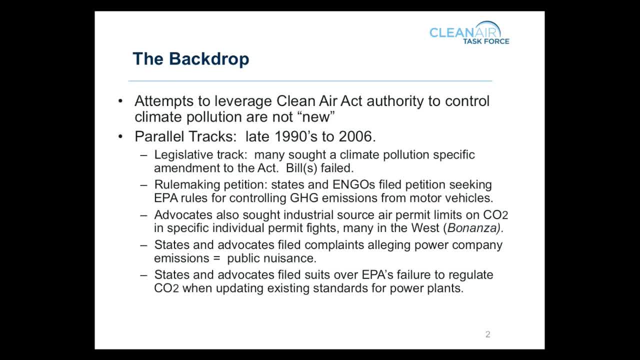 Unfortunately, in Congress that failed. So what's left? Well, there were a group of states, and environmental groups filed petitions seeking EPA rules to control carbon dioxide and other greenhouse gases from vehicles. Advocates sought industrial source air permits on CO2.. 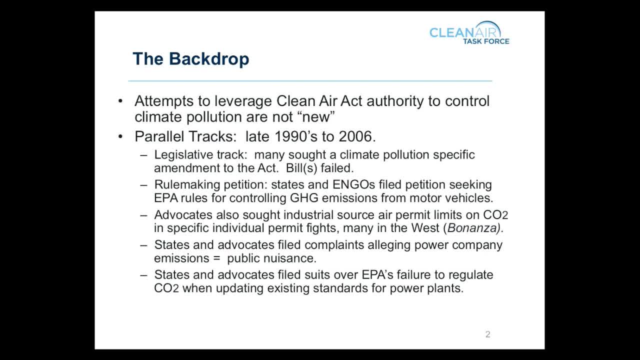 We filed complaints alleging power company emissions were a public nuisance. We also filed suit when EPA was working on updating standards for various industries, saying that in the Bible there was no sun, neither was there water, nor there was oil. That is just terrible news and I'm done. 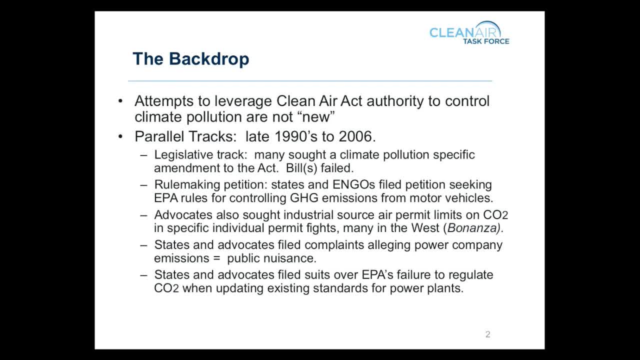 Go ahead. Okay, I'm going to stop. Go ahead, Go ahead, Go ahead In those standards. EPA should be setting carbon dioxide standards, setting methane standards, setting standards for those air pollutants that have climate effects. I'm going to go through each of those very briefly. I hope so that I'm within my time. 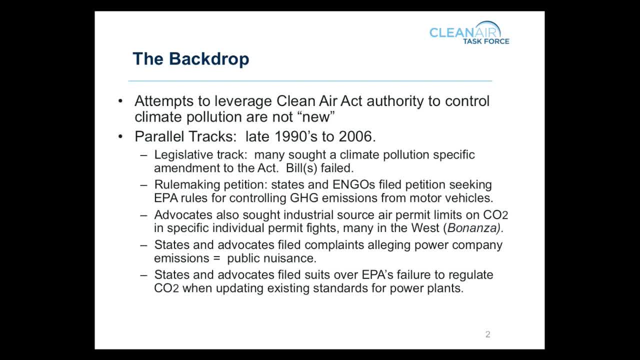 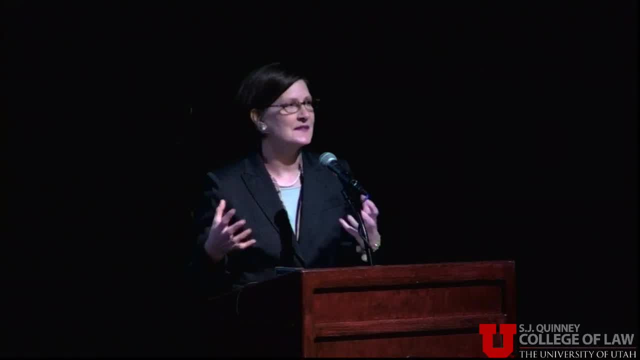 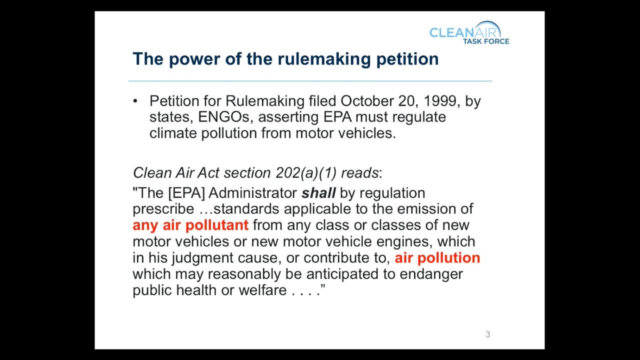 because this is a lot of history. I'm going to start with the power of the rulemaking petition. It said the Clean Air Act has these opportunities for citizens to engage in the process, and citizens did. They asked for the Environmental Protection Agency to write a detailed rule about how. 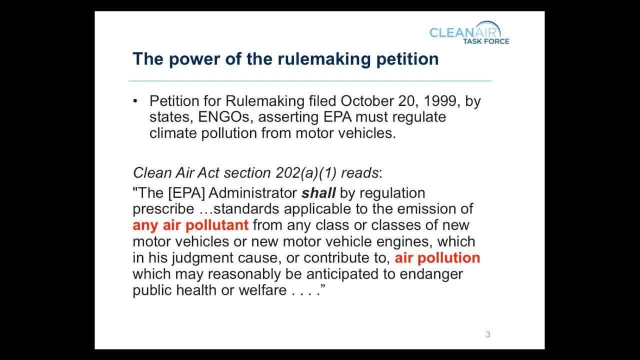 to control the carbon that is emitted by motor vehicles, which is a good part of the national problem. This is engaging the precautionary principle that we just heard about. The statutory language is up there. I won't read it, but you can see the reasonably be anticipated. 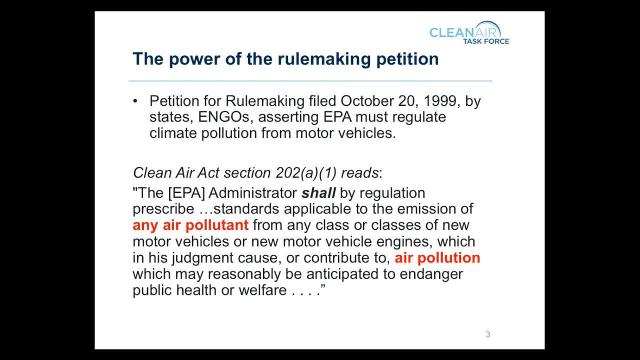 to endanger public health and welfare. The argument went: carbon dioxide is an air pollutant. It causes public health effects, it affects welfare, welfare including climate effects, as the act defines it. In fact, this rulemaking process, the act defines it. 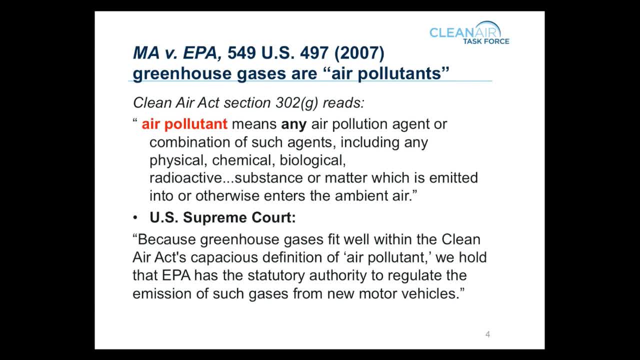 I'm going to stop there, Thank you, I'm sorry, Thank you, Thank you, Thank you. The process went through several iterations, with changes of mind in the inside EPA itself, several administrations and finally ended up at the Supreme Court. 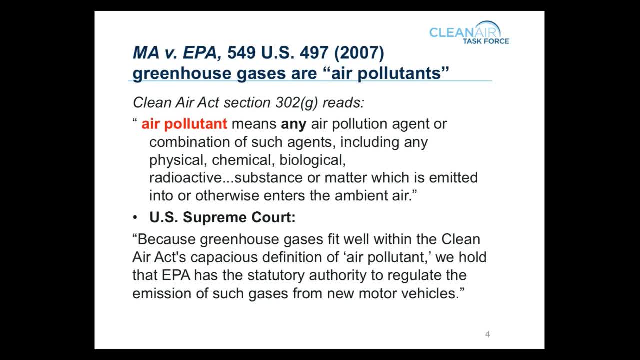 The Supreme Court said yes, indeed, any air pollutant. air pollutant means any air pollutant agent, Because greenhouse gases fit well within the capacious is the word definition of air pollutant. We conclude the EPA does have the statutory authority to regulate the abuse and pollution. 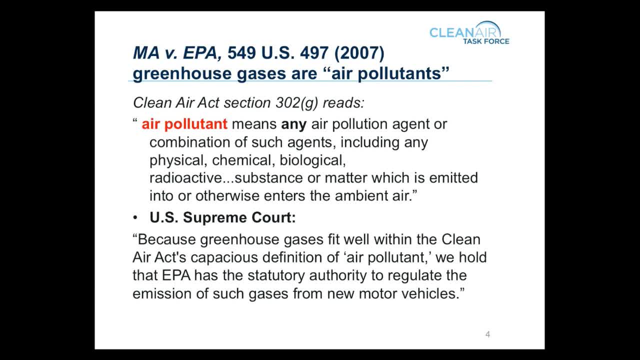 the emissions of those gases from motor vehicles. The related question, of course, is: is the agency going to decide that the emissions from motor vehicles do endanger public health and welfare, and will the agency determine to regulate? Well, immediately after this, the administration started working on that. 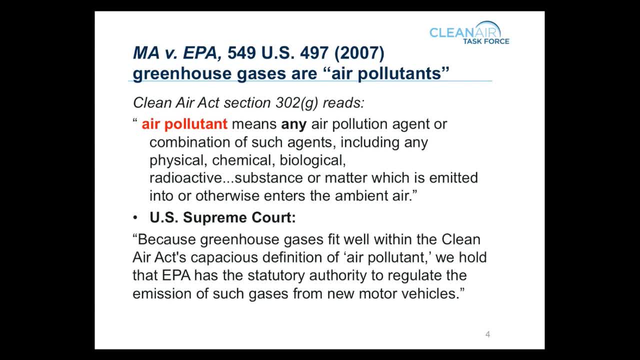 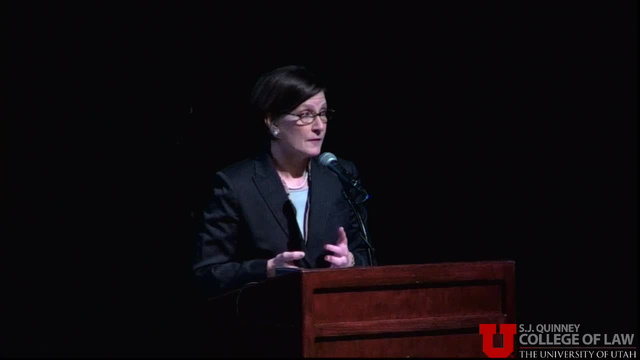 And in 2009,, promulgated something called the Endangerment Finding, which said yes, indeed, there's a basket of six air pollutants. they cause climate effects, they cause public health harms and they cause welfare effects, meaning environmental damage. 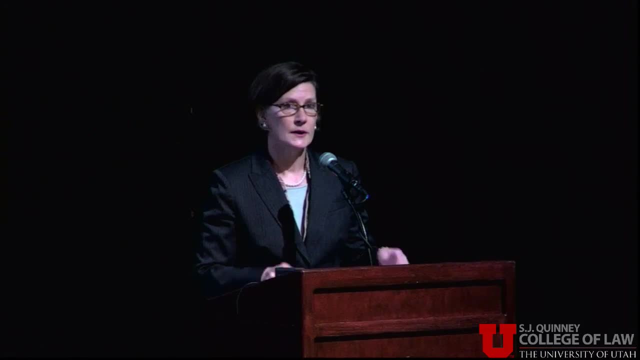 And EPA promulgated a rule for the automobile industry and EPA promulgated a rule saying that when a vehicle is damaged, it should be protected. When a new stationary source of air pollution, like a power plant, comes in, it needs to include. 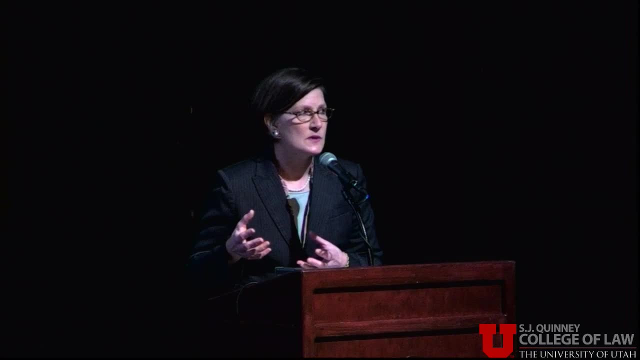 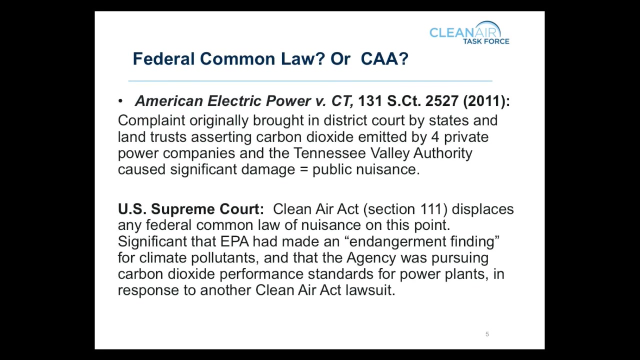 in its air permit limits on the emissions of these greenhouse gas pollutants. I'm not strong enough to push this button. Okay, There we go. All right. another parallel track was happening at the same time. Another train was on a different track. 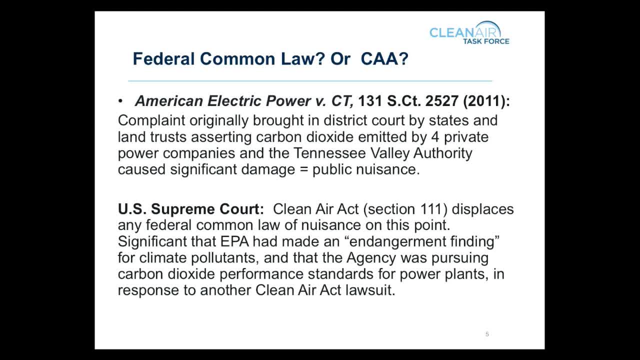 States and citizens brought a case and filed a complaint saying that four privately owned power companies and the Tennessee Valley Authority, which is a federal entity, were emitting so much carbon dioxide that it was causing them harm and that this was a public nuisance, So because the agency wasn't doing anything under the statute. the argument was this: 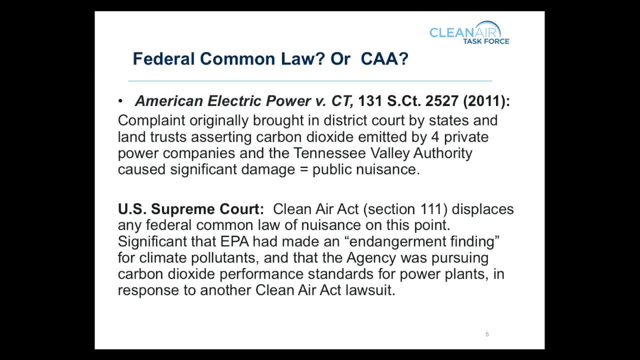 is a public nuisance. We are going to ask the court to make it right to tell these companies that they have to reduce their emissions. Well, this case got all the way to the Supreme Court and the Supreme Court said no. The Clean Air Act displaces the federal common law if there is any of nuisance. 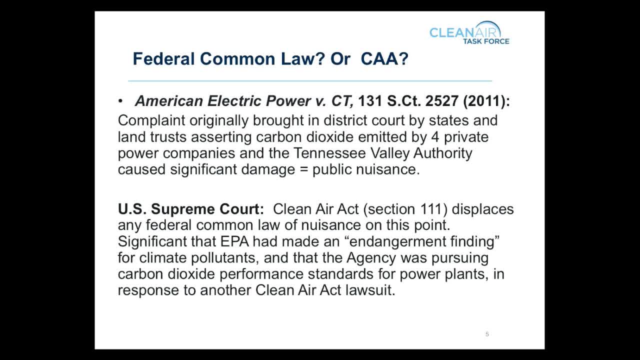 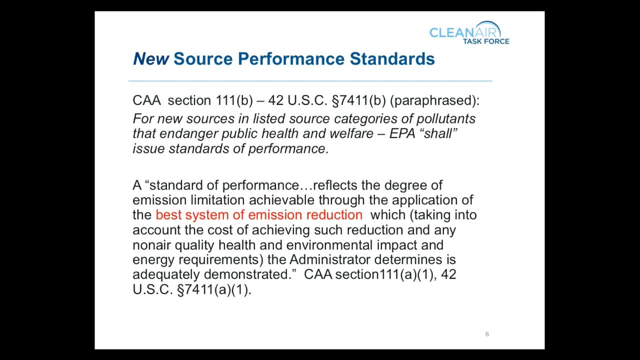 Okay, So this is a public nuisance for climate pollution and the damage it causes. So as we march through time and we use these parallel tracks, we are getting more definition about what we're going to do about this pollutant. So where are we now? 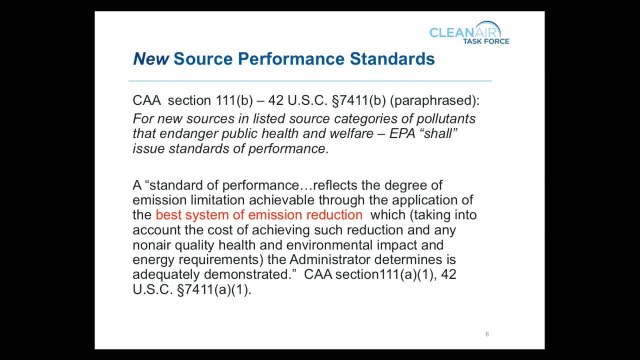 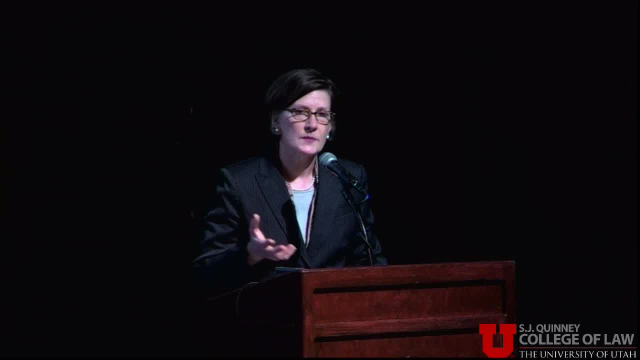 Well recall that a group of states had challenged EPA for discussion, Okay, For deciding not to regulate carbon dioxide when it updated performance standards for power plants back in, say, I think it was 2005.. There have been standards for power plants since the 70s, controlling their emissions. 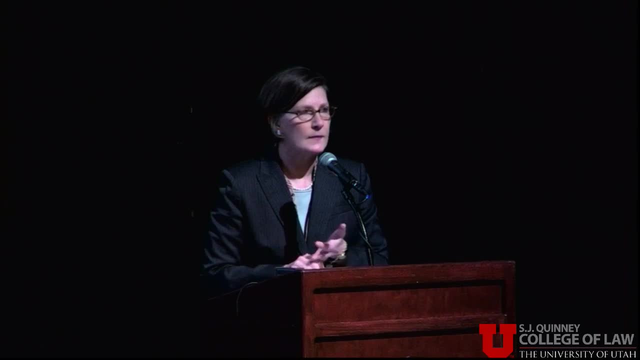 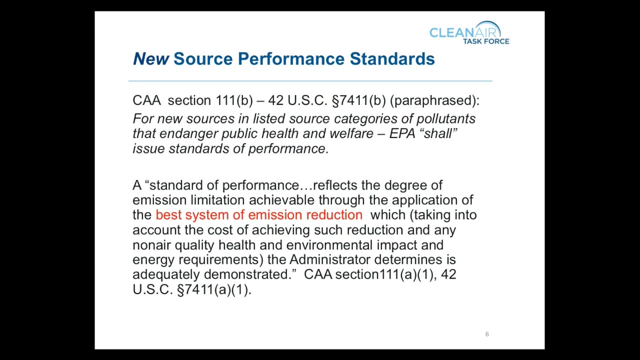 of smog forming and particulate forming pollution, And when those were updated, the challenge came in: No carbon dioxide, No carbon dioxide, No carbon dioxide regulation. Why So, coming out of that, now that we have the Supreme Court saying there's no federal common? 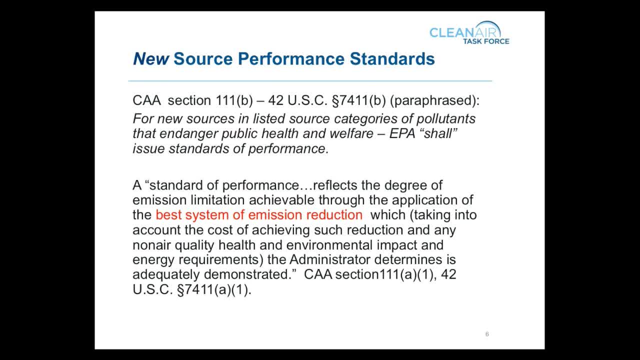 law. the agency should be using the performance standards section of the Clean Air Act, because that's what Congress intended. We now have the agency working on performance standards for carbon dioxide from new sources of that pollutant, particularly in the power sector. That's the first one. 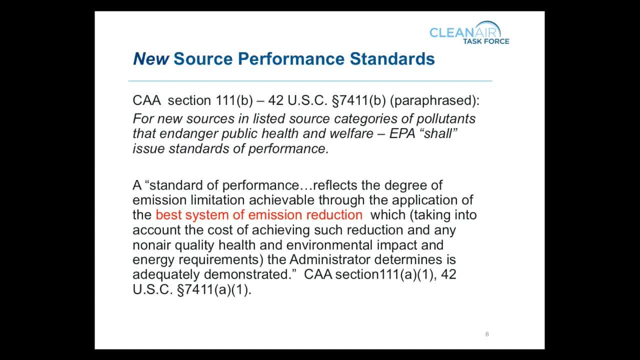 So there are. the section in the act we're talking about is Section 111.. Section 111B basically says: if you're a listed source category, if your industry is one that reasonably will contribute to damage to public health and welfare, and I'm paraphrasing here: 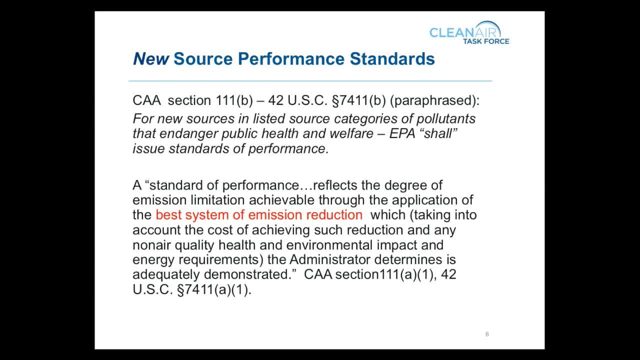 EPA shall regulate your air emissions of the pollutants that cause the damage. And I have again put the language of the statute up here And I'm not going to dwell on it too much, except to say that the key thing here is this: 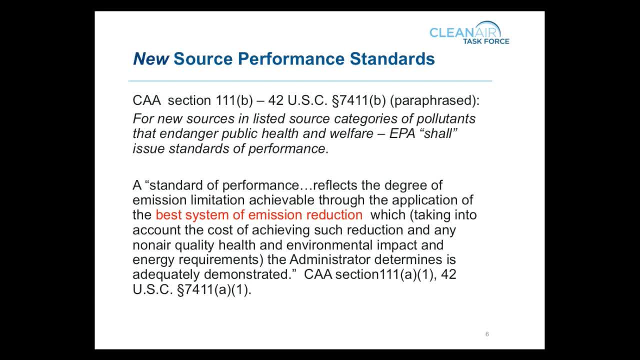 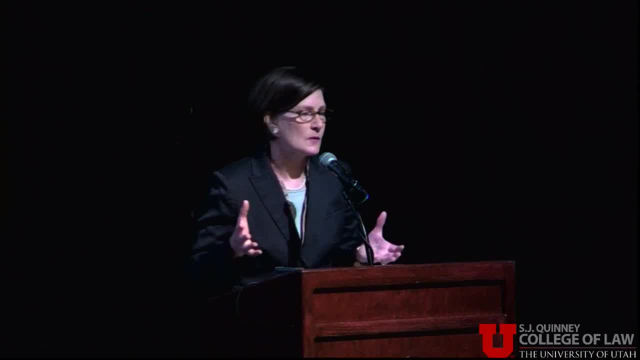 best system of emission reduction, which forms the basis for how much improvement we can expect to get Right. So that's always the question: Okay, So you can do this, But what are you going to get from that? And recall also that another subsection which I touched on briefly, another subsection of 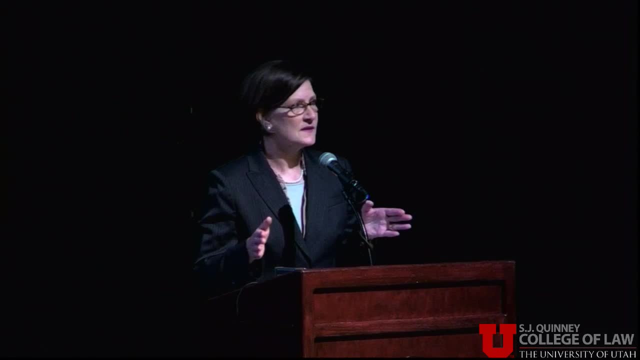 this part of the statute says: Once EPA sets the standard based on the best system of emission reduction, it has to look back at it every eight years And it has to tighten it up if the improvements in technology have so warranted. And I'm not quoting a statute. I'm just giving you the idea. So you have this best system of emissions reduction idea that we're really looking for something that can cause some improvement. That will. You know, move technology And this section of the act has been around since 1990.. 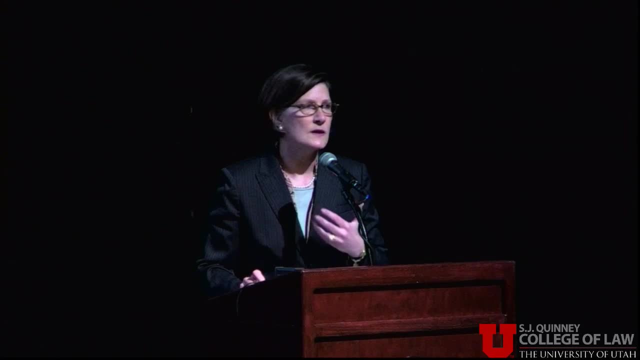 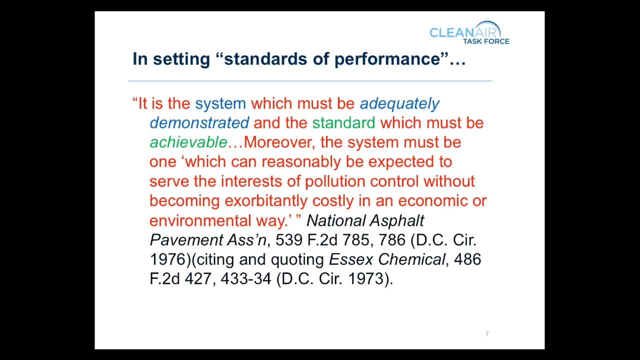 So we have a pretty good amount of history with it in the conventional pollution arena. Try my button again. So, for example, in setting sulfur dioxide standards or NOx standards, the agency has typically- And I think you probably heard a lot about this- 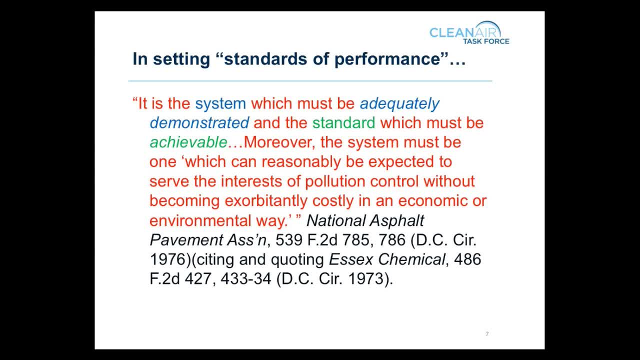 You probably heard a little bit of this from the first two speakers- Maybe not gone as far as it could have. It's sort of looked at the industry and seen what was out there And it set a standard that's fairly stringent and in fact does move technology. 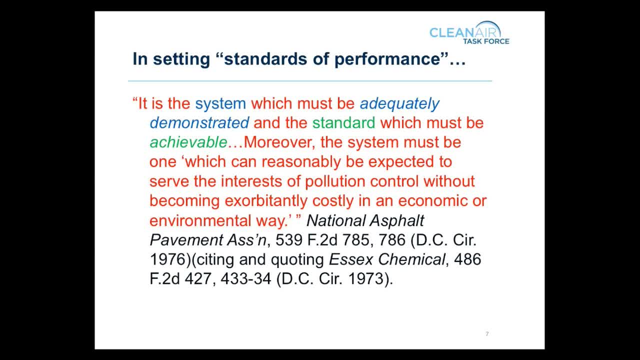 There's a good body- and I won't get into it too much, but there's a good body of research that suggests that a stringent standard setting process actually provides financial incentives. It provides policy incentives, it provides all sorts of incentives to private companies. 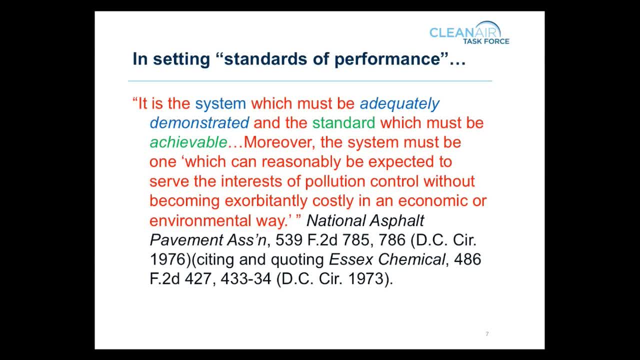 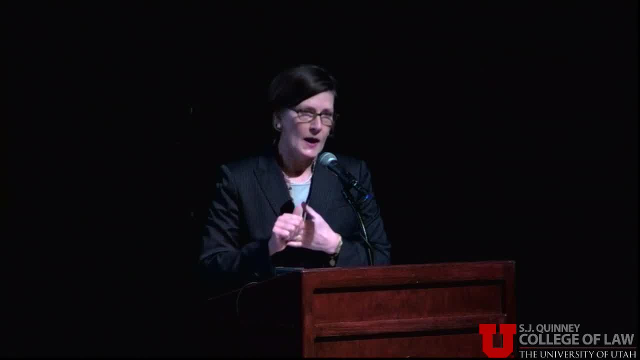 to develop new methods of more cheaply getting the reductions that are required. It really does force technology. People challenge the rules. That's how the act works. Not only do we have these hooks to get the rules in the first instance, but we also have 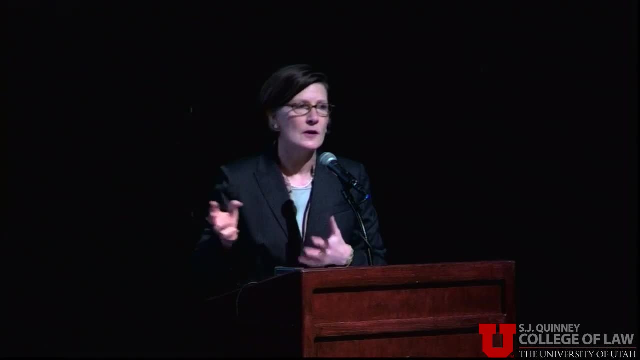 the ability to say: agency- you haven't gone far enough. or, on the industry side, agency- you've gone too far. The courts look at the statute. the courts make that decision. we all know that We have now this case, this body of case law, about new source standards and setting standards. 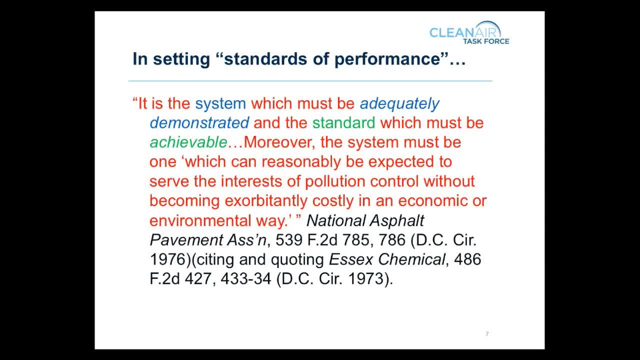 of performance And this is one of the cases- and you can see how old they are: 1973, 1976.. The system has to be adequately demonstrated. the standard has to be achievable. When considering costs of the pollution control, they can't be exorbitant. 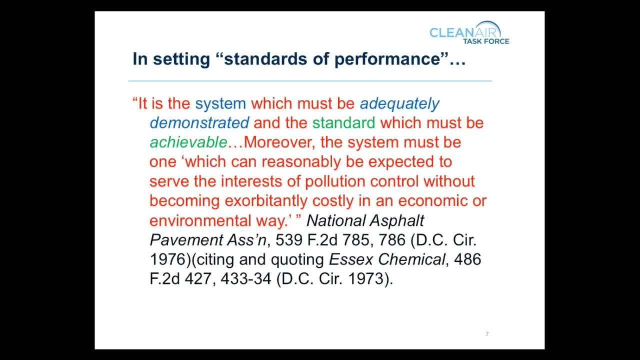 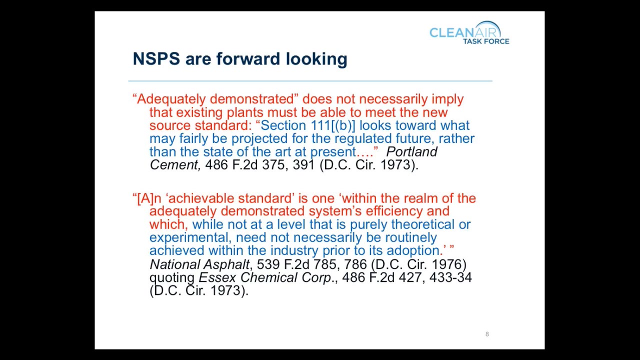 Exorbitantly costly. that's a pretty broad, pretty high low bar. I guess great discretion, low bar, Exorbitantly costly can allow a lot of technological improvement. it seems to me We also know, at least in the new source context, that they are supposed to be forward looking. 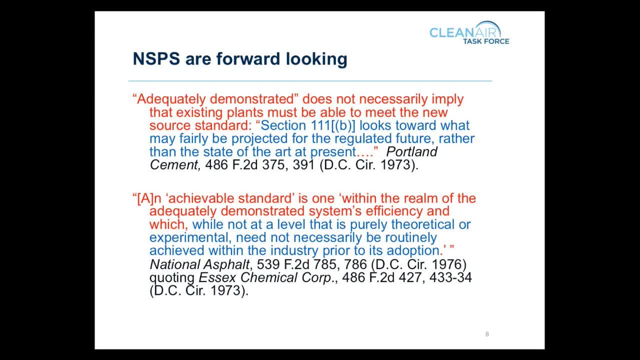 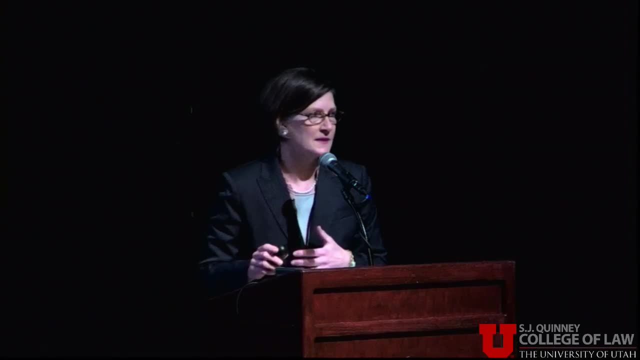 They're supposed to look forward to what could be achieved. They're supposed to be in the industry over the period of time. remember, these things are supposed to be good for eight years and then you're supposed to reevaluate them. They are within the realm of achievable standard is within the realm of possibility, basically. 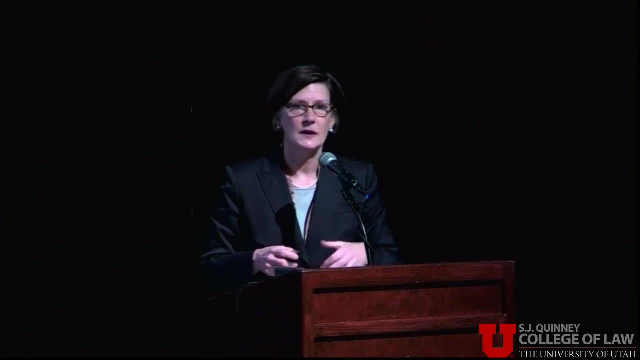 But it can look forward. It doesn't have to be what every facility in the industry is doing now And then. my technology forcing piece, EPA, is allowed to extrapolate from a technology's performance in a different industry. So for example, in NOx, control the nitrogen oxides, control the pollutant that causes. 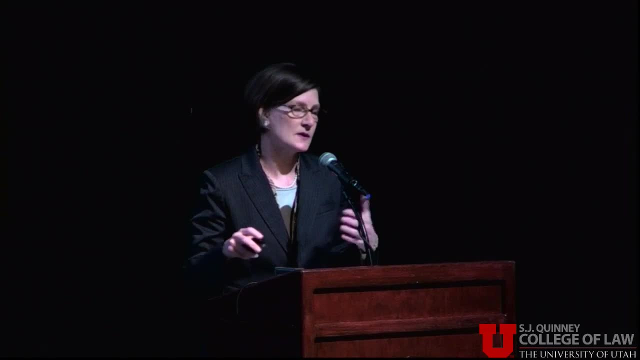 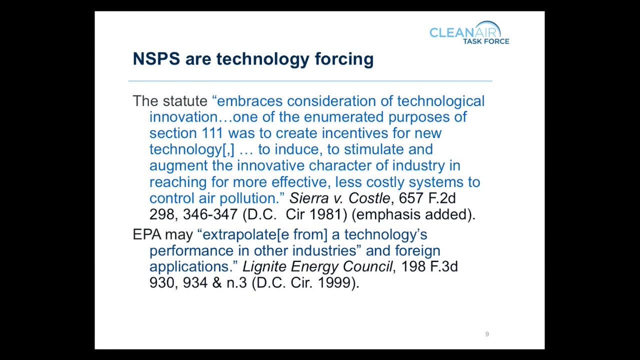 smog. what we saw in the application of this section of the act was bringing control technology for smokestacks over from one industry and another country into our industry, into the electric power sector. here And now. it's pretty much ubiquitous, Okay. 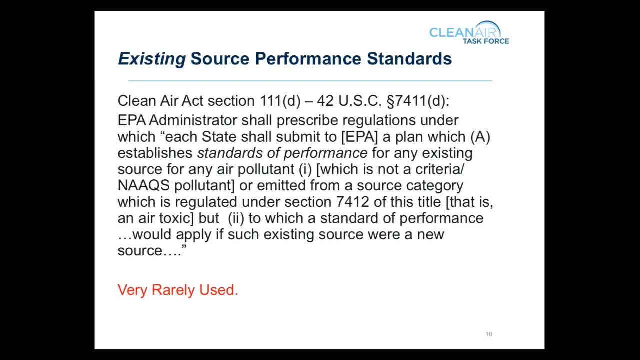 So once you issue new source performance standards for an industry, the statute says that for certain pollutants you may also regulate existing sources, And carbon dioxide and other greenhouse gases are that kind of pollutant. They're not a NAx, not an ambient pollutant. 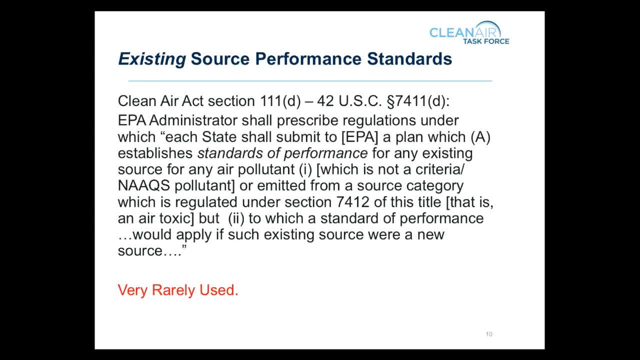 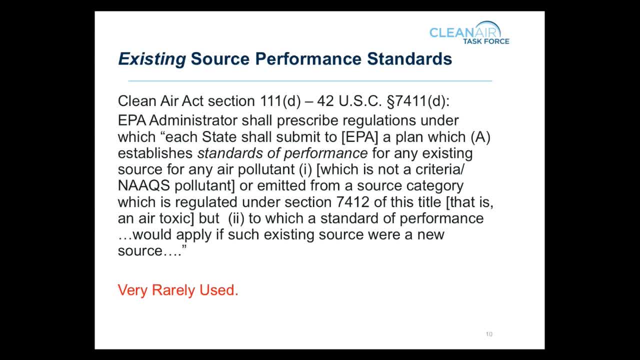 So if you have a listed air toxic, remember in 1990, EPA was told it had to regulate a list of 189 air toxics. Congress told it that, whereas previously EPA got to pick, from 1990 on there's a list. 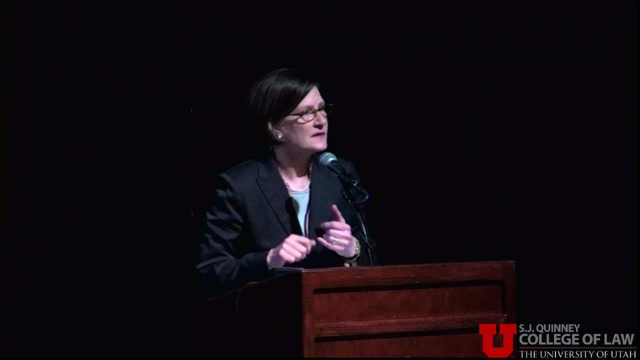 of air toxics And if you're not an air toxic and you're not a conventional pollutant but you're still emitted in large quantities from an industrial source, you can be regulated under Section 111D- the existing source performance standards. 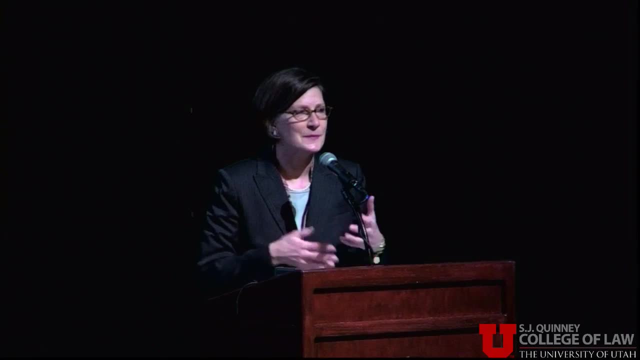 standards once that pollutant has been regulated for new sources in that industry. This section is very rarely used. One of my colleagues likes to refer to it as the 40-year-old version. There are maybe four to five rules total since the 70s. 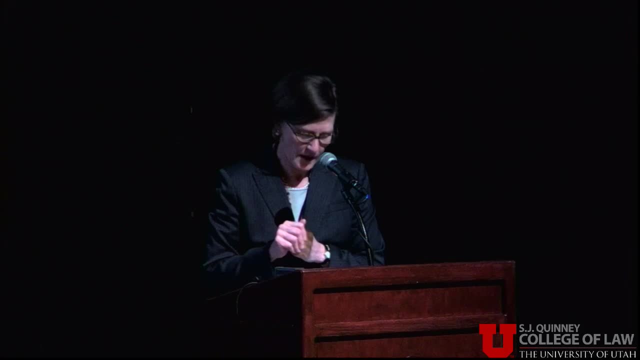 And the way it works is this: EPA directs the standard setting process, defining the minimum for acceptable plans and standards, And then the states implement them, Sort of like that state implementation plan. although this is specific to these gap pollutants, The rules that EPA developed that govern this process refer to guidelines. 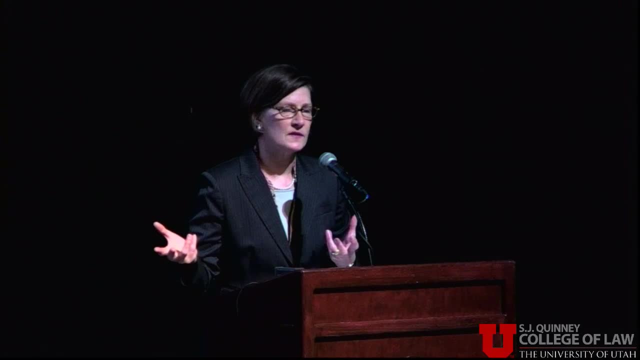 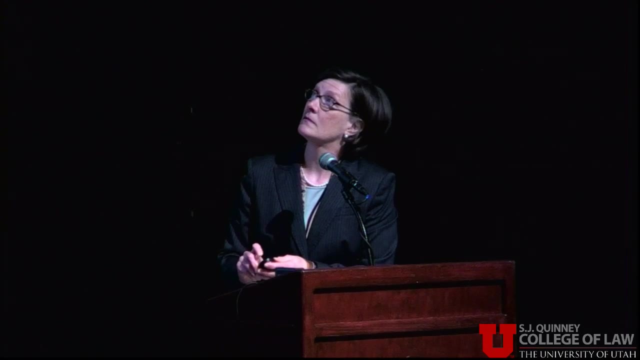 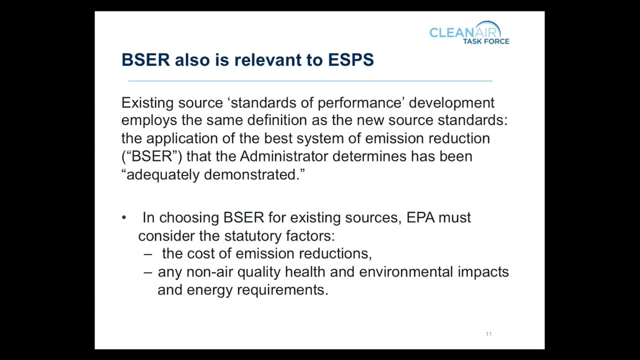 So EPA will issue guidelines to states about what they're supposed to do in order to get their SIPs approved. So what's interesting about this to me is that the statute uses the same definitions for existing and new source standards. So even though we don't have a lot of experience with the existing source standards, we know 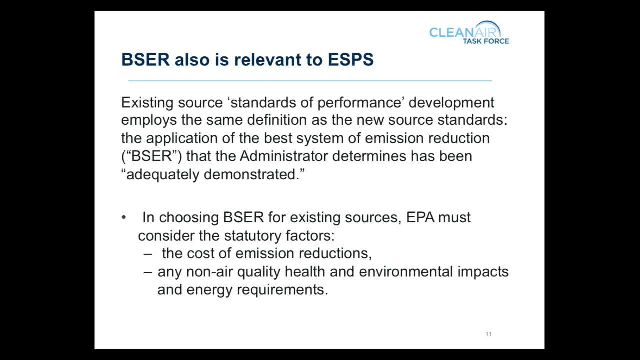 that the best system of emission reduction is going to be limited for existing sources or defined in the same way it is for new sources, as a legal matter In choosing end Or directing, if you prefer, a BSCR for existing sources and setting a standard that the states 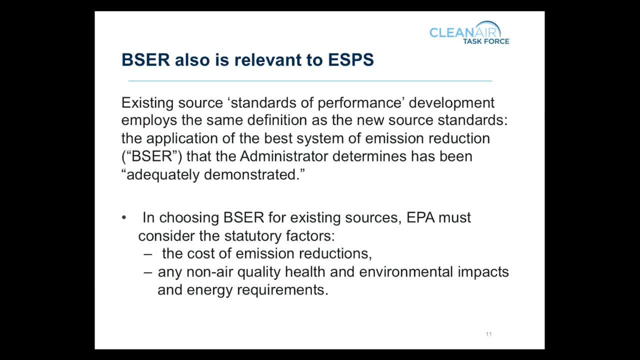 have to meet. EPA has to consider all the same statutory factors: the cost, the non-air quality, health and environmental benefits. So what has EPA done? EPA set a 111, or proposed- it hasn't been finalized yet- set a new source performance. 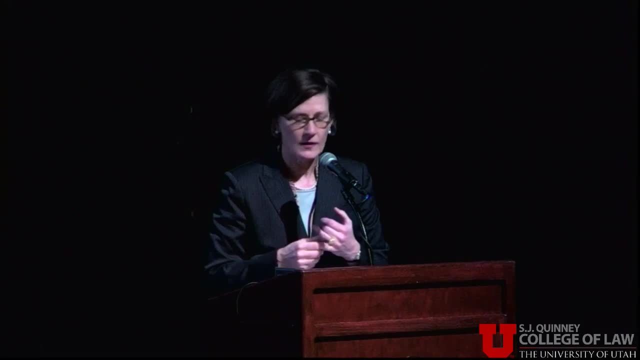 standard for carbon dioxide for the power sector. It's set roughly at the level that a new natural gas plant achieves, And relying on carbon capture and sequestration, which is a technology for actual capture of the carbon and sequestering it in geologic formations. 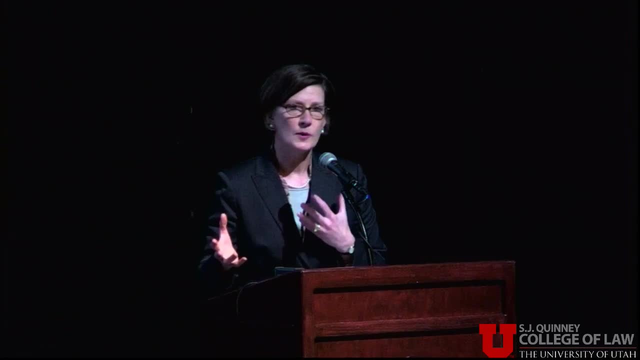 Once they proposed that standard, they also proposed- in response to a presidential directive in 2013,, the president's climate action plan. They also proposed existing source standards and the comments on those. the comment period on those standards just closed. We expect the whole package to be finalized over the summer. 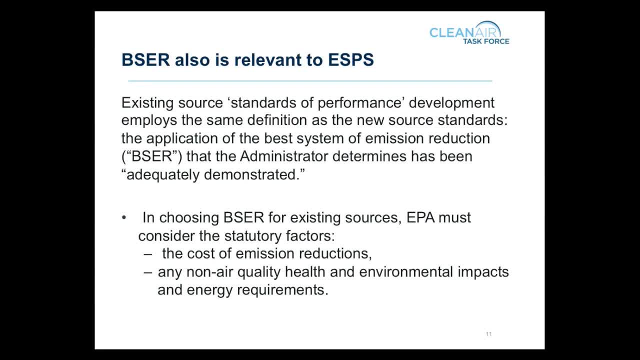 So what has EPA done? for existing sources, It's decided that the best system of emission reduction is based on state targets, based on four building blocks. What can you do to reduce emissions? You can reduce emissions at the nation's fossil fuel-fired power plants, which is the regulated 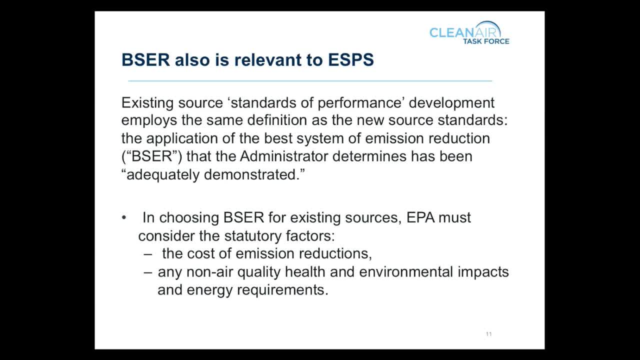 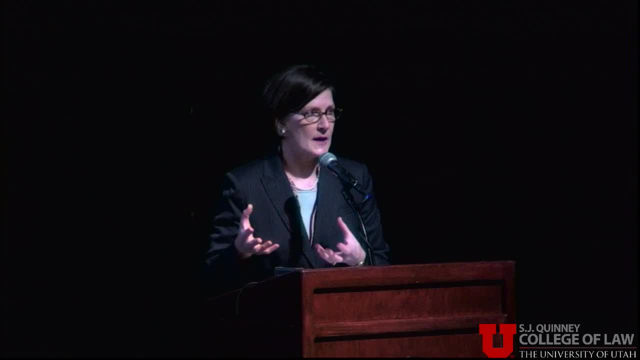 industry. Well, there are controls that you can do at the source, that's building block one. You can redispatch existing natural gas facilities, which emit half the carbon dioxide of a coal-fired power plant, to cover the load, the electric load and demand. 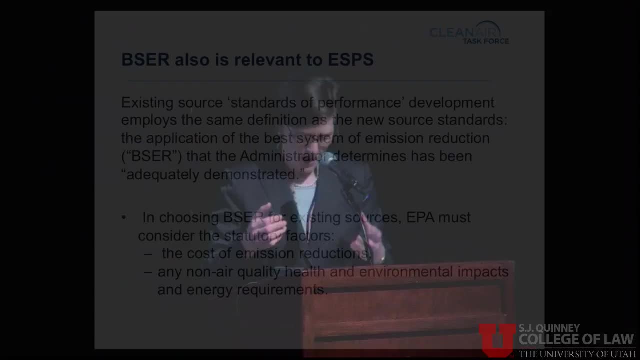 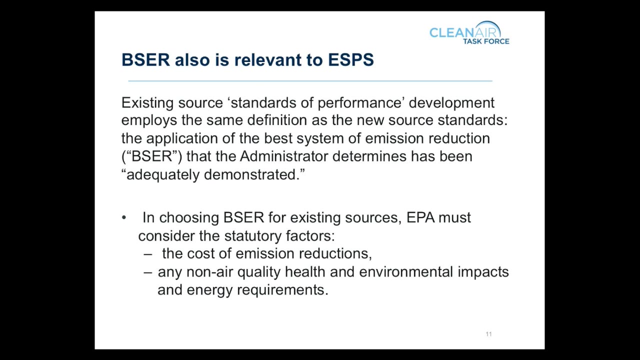 There's capacity there to be able to do that. So that's building block number two. You can promote the idea of using more zero carbon energy, like wind and solar, where that's appropriate. That's building block three. And you can promote the use of energy efficiency and demand management- electricity demand. 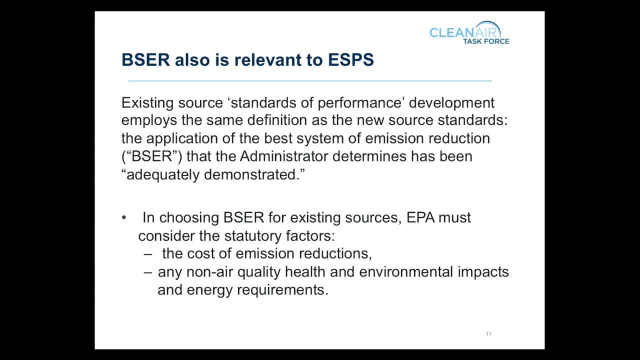 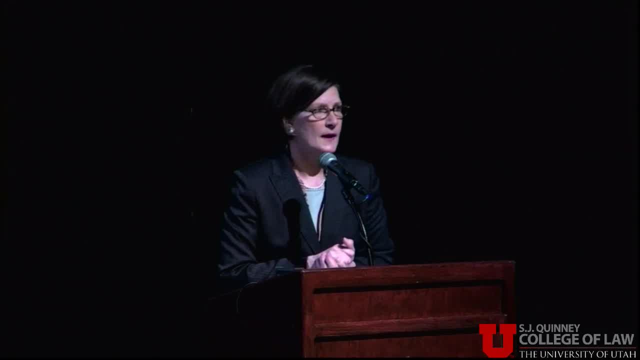 management as a way of running the oldest, dirtiest, most carbon-emitting plants less and lowering the carbon dioxide. And you can do that by using the existing electric power system in our country. It's where 40% of our carbon dioxide comes from. 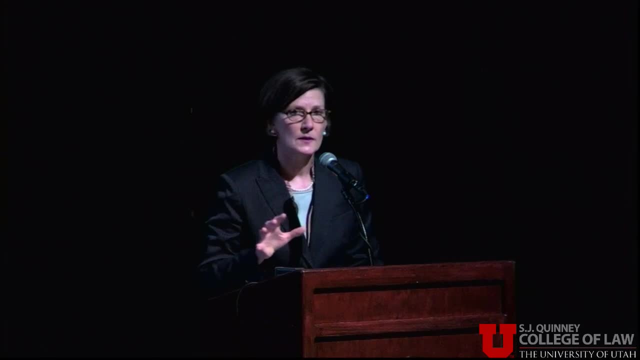 There's a lot of state flexibility in this. Basically, as I said before, EPA issues a guideline, It tells the states what to do. It uses BSER to develop state rate-based targets, So it's a great platform. I think it's a great tool. 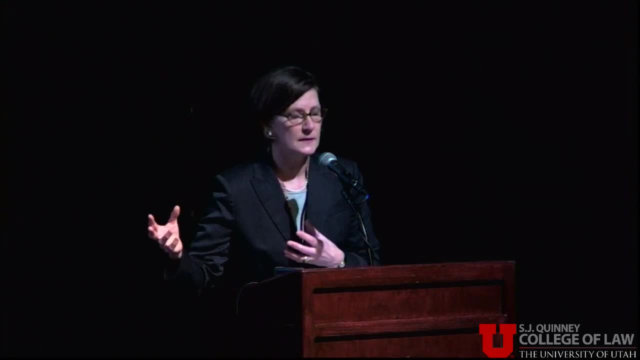 It's a great tool. Thank you. So carbon dioxide per megawatt hour of electricity for the electric sector And the states get to submit plans and I guess they have a year to do it. They can have extensions, But the state plans are not limited to the building blocks. 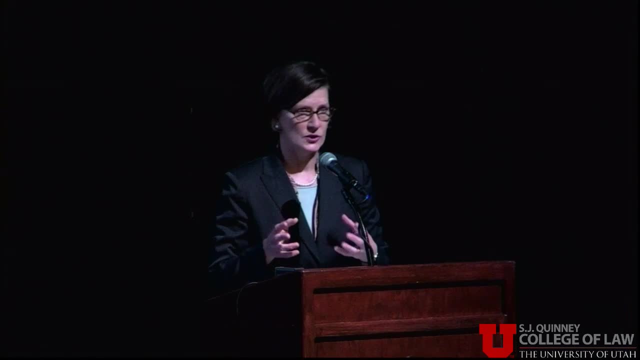 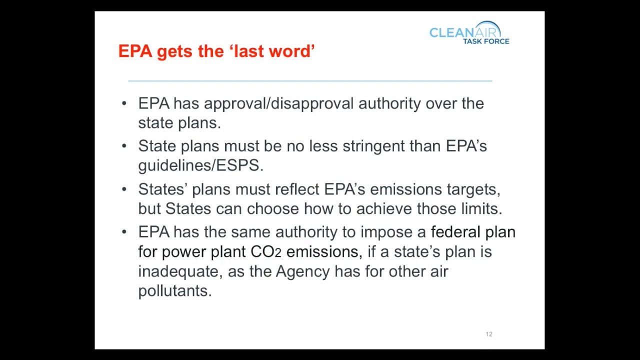 They don't have to do the things that EPA says you can do. They can achieve those rates in a lot of different ways And quickly, because I'm running out of time here. importantly from my perspective, EPA gets the last word. 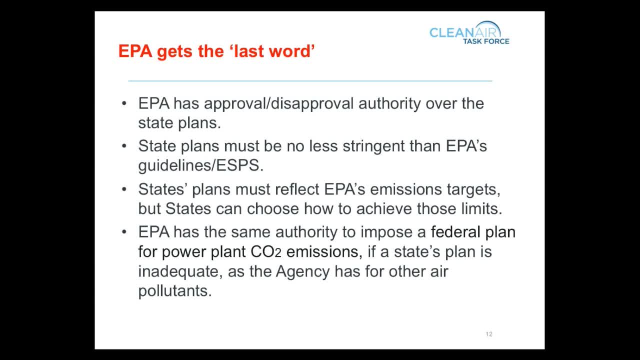 EPA has approval and disapproval authority over the state plans and you know, obviously is directing them through the guidelines. EPA can issue a federal implementation plan, can say to a state: your plan is not acceptable, This is the acceptable path And EPA has, in fact, recently announced that it will do that for the electric power sector at the same time. 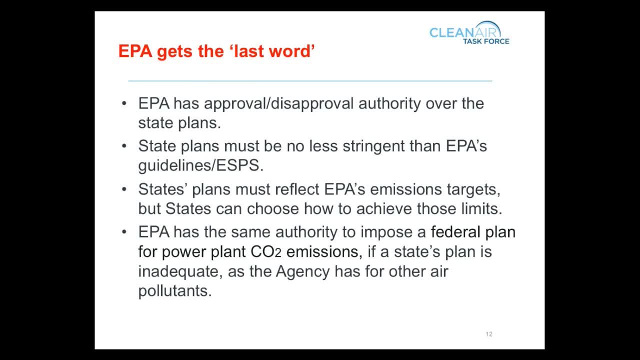 It was going to propose a federal plan At the same time it finalizes these rules coming up this summer. We- my organization and some others- are advocating for the agency to include a mechanism that sets out sort of the minimum acceptable criteria for a mass-based capitalization. 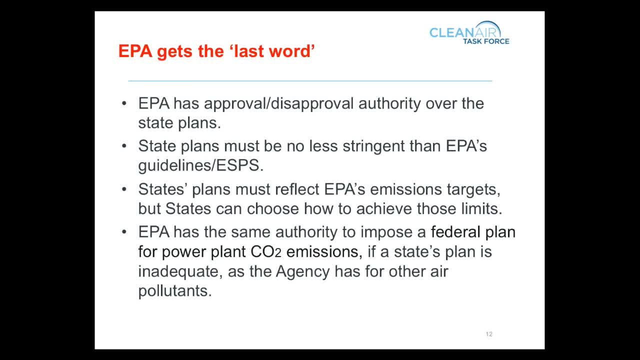 We're going to need to do a bit of a rethinking of the concept of a capitalization plan and see if there's any other action that we can take to address that. The other thing that I would say to the state is that we're going to need to have more of a national plan in place. 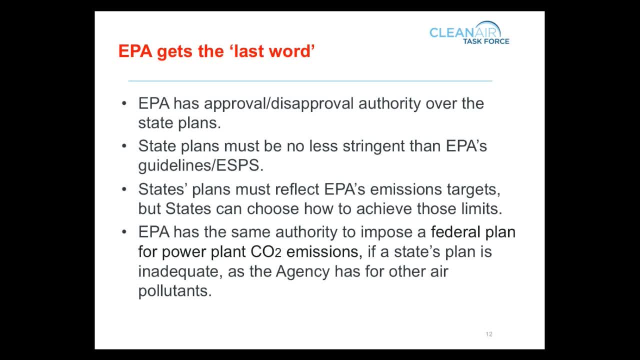 But the state has a lot of interest in how that can work in the future. So in other words, if you were going to, if you, the state, wanted to participate in deciding to achieve the state target through a process of trading emissions credits within other states' plants, that EPA would set up the minimum contours for that. 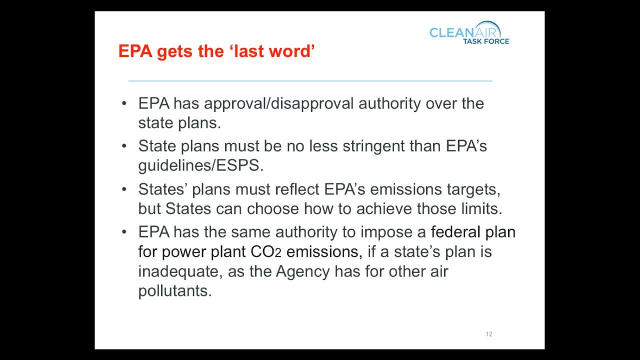 Which works in a state like Kentucky, which is mostly coal-fired power plants. The state is not going to want to have a capitalization plan that would go through the process of trading emissions credits with other states' plants- Kentucky- which is mostly coal-fired power plants. it's hard to see how they're going. to be able to get the reductions from the coal plants within the timeframes when they're needed. Whereas other states are already getting these benefits, They're already retiring Coal plants, are already retiring. New gas plants are being developed. They're generating more credit. 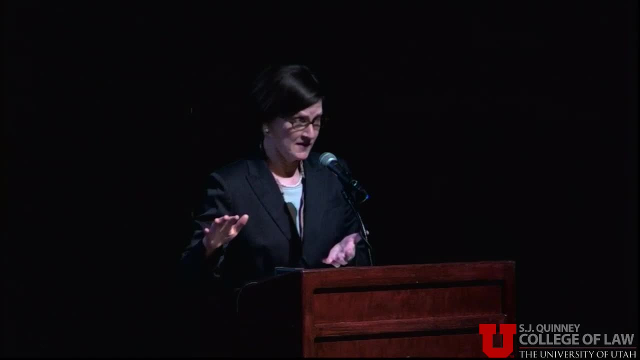 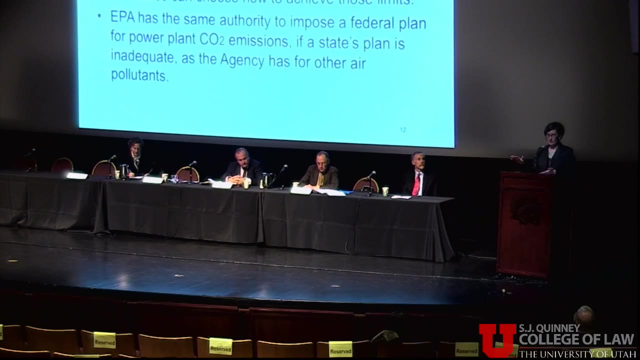 They're getting more reductions than perhaps the state targets would suggest they need. New nuclear plants are being developed in the southeast. Those are zero carbon emitting. Is there some way of sharing the benefit of the development of other kinds of renewable resources like wind and solar, which have been increasing quite a bit in the last couple? 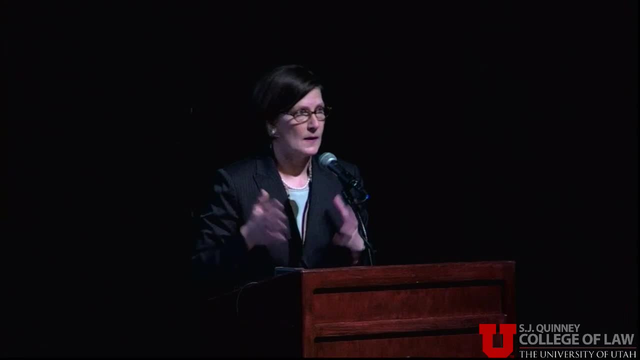 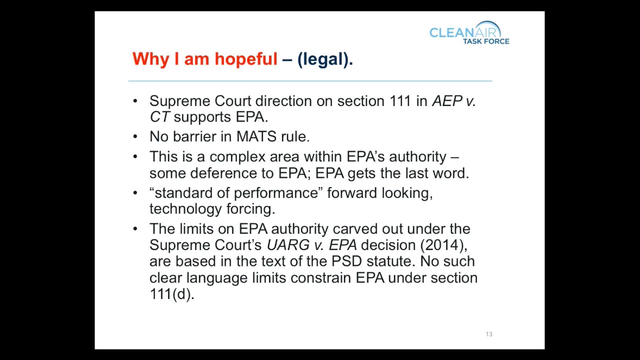 of years. Is there some way of sharing that? That's the concept behind it. That's the concept behind the allowance trading system that we're advocating. Okay, I'm going to wrap up, because I'm going to try to wrap up. 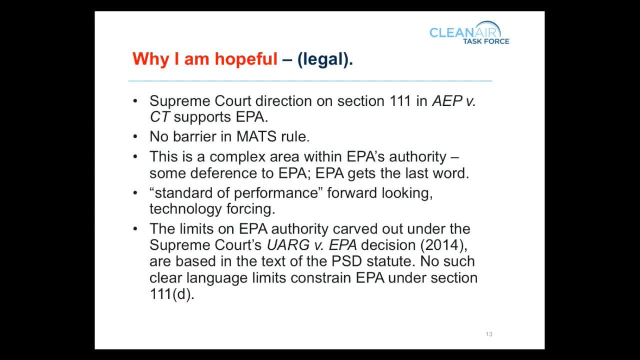 I'm going to give you a couple of pages on why I'm hopeful, a couple of minutes on why I'm hopeful. I'm not Pollyanna, but we have the Supreme Court's direction on 111 in the AEP case. EPA can do this. 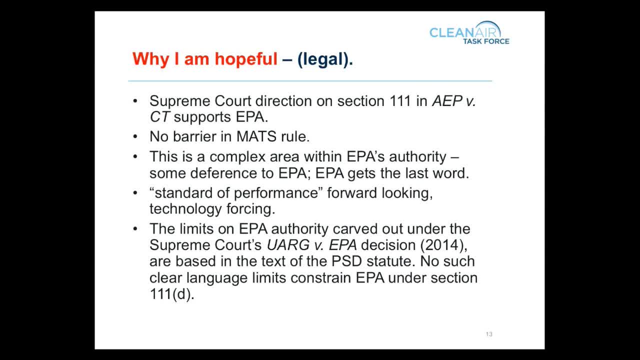 Should do. this Is doing this. It already has that blessing from the Supreme Court. My second bullet is I could spend an hour talking about, but there's a case ongoing challenging EPA for even thinking of proposing existing source standards, because they've already regulated the same industry for its air toxics. 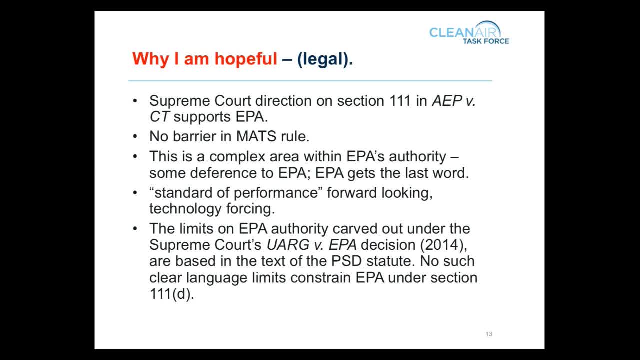 I don't see any barrier. We're in that case and we've just filed briefs in that case. I can answer questions about that case if people want to talk about it. This whole scheme is a complex area and the case law suggests that in a complex area. 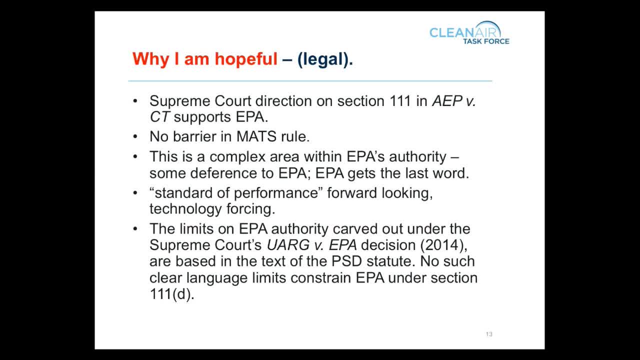 within EPA's authority. EPA gets the last word. Standards of performance are forward-looking. They're technology-forcing- I really do. One of the professors that I had in graduate school was doing the research about what happens in an industry when strict environmental laws are put in place. 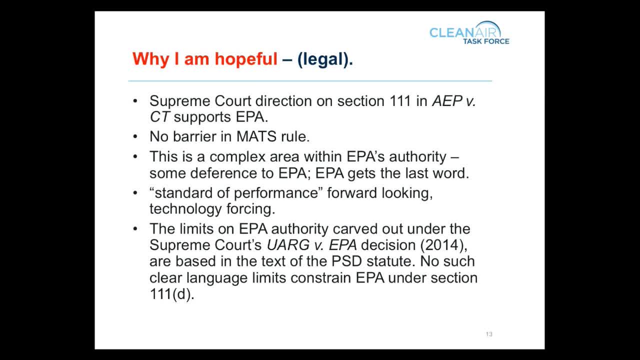 I don't see any barrier. Okay, That's a good question. I don't see any barrier. I don't think any environmental improvement is required. In fact, technology develops, It works. briefly, Then the question. This is a slide that I've used before in talking about a different 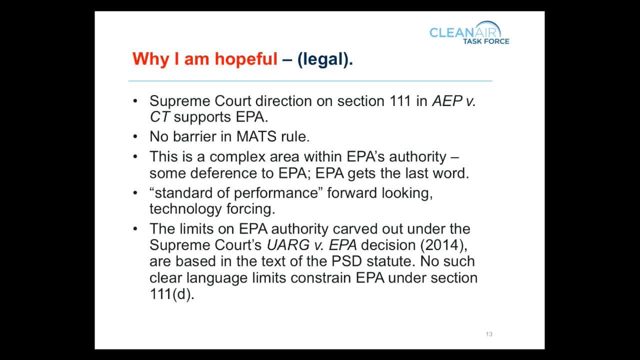 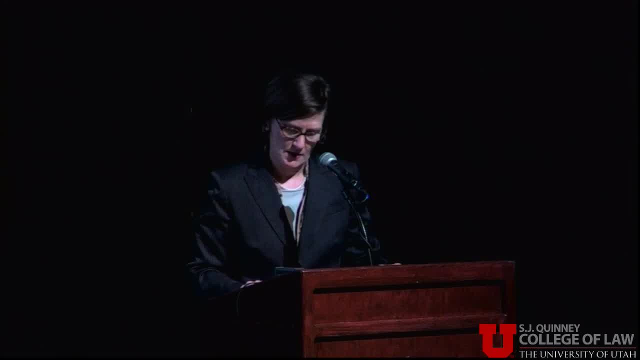 case. There are no clear language constraints on EPA's discretion here, such that they can't regulate carbon pollution under this standard. Those are the legal reasons. That's why I'm hopeful In real life. I'm hopeful because required change happens, as we just discussed. 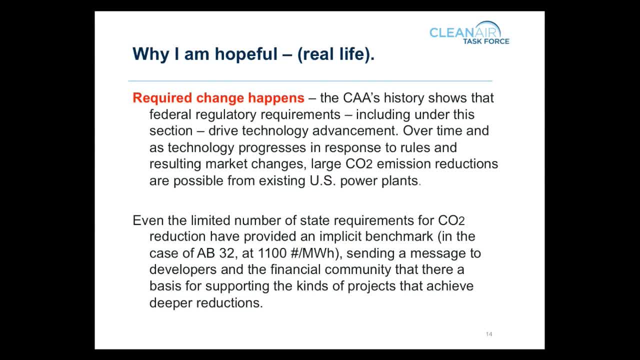 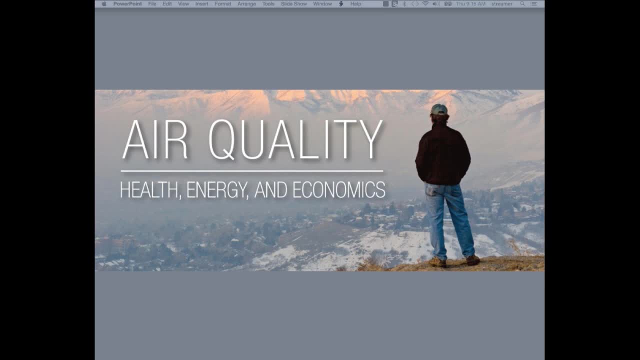 We see that with carbon dioxide, Even just the few states that have defined what their limits are on carbon emissions have seen improvements. What's next? Oops, What's next? It's the next speaker. I can't go back, but I'll tell you what's next. 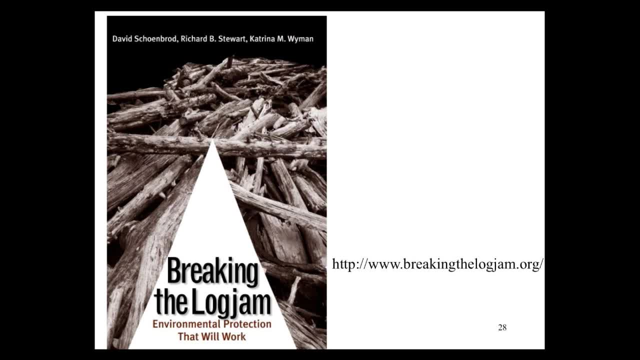 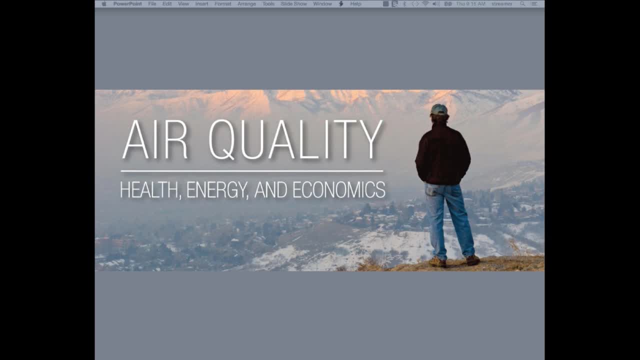 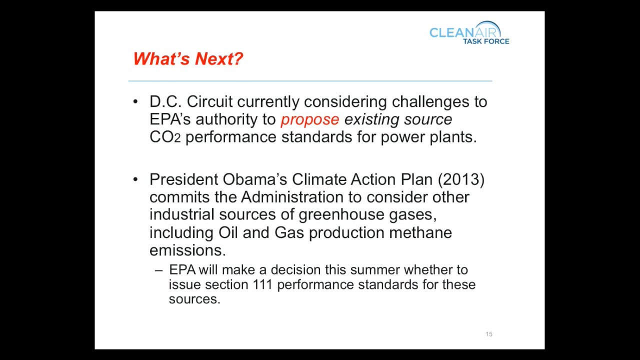 The DC Circuit, as I said, is working. It's working on this case. that's challenging EPA's audacity and even proposing carbon standards. We're going to hear from them about that. EPA will finalize its power plant rules for new and existing sources. 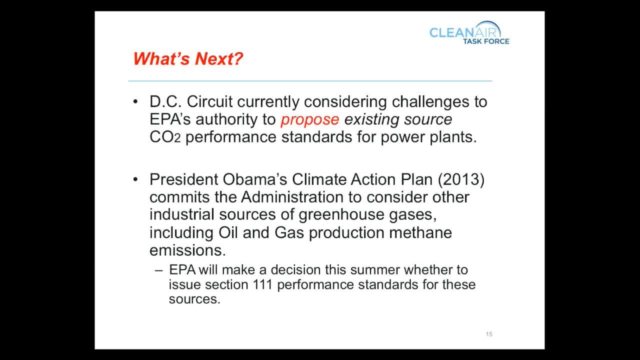 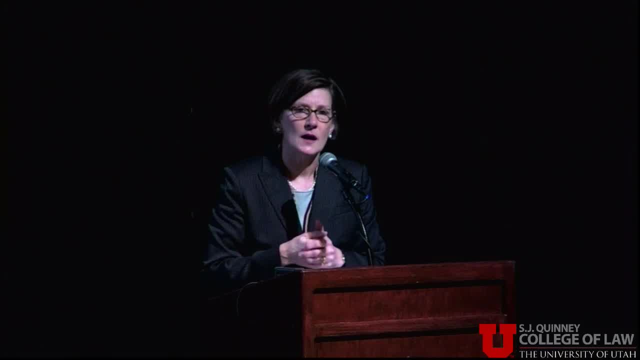 EPA will promulgate a FIP. at least that's where they say they're going, where the president has directed them to go. In addition, The agency is now working on making a decision about whether methane regulations should start being developed for the oil and gas industry. 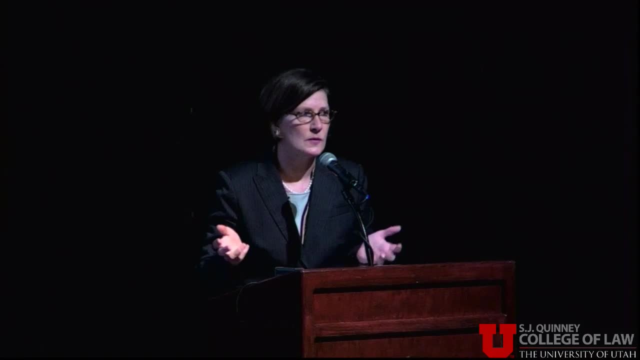 The oil and gas industry is a major emitter of methane, which is also a very potent climate pollutant. EPA has committed to making a decision this summer about whether to set performance standards for sources of various kinds in the oil and gas industry. That's what I have for you today. 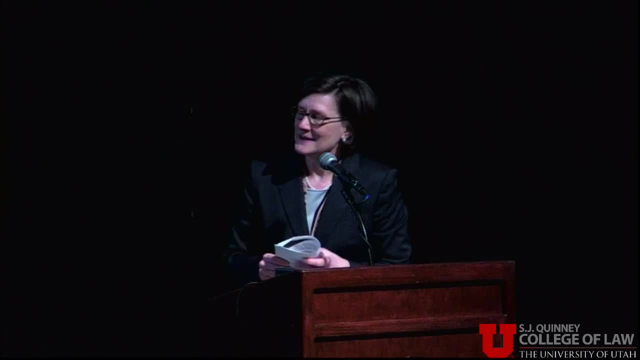 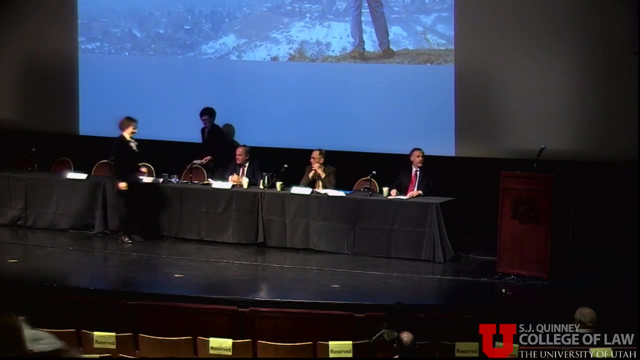 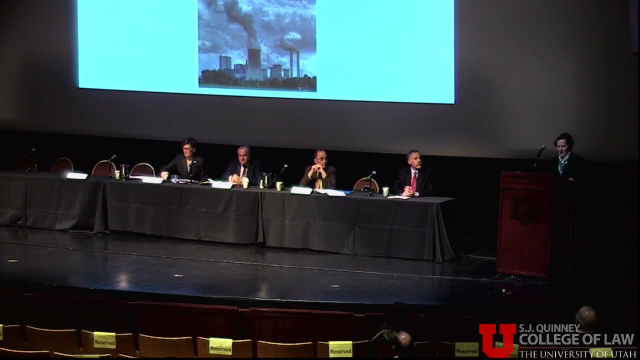 I'm hopeful. I'm continuing to work. There is, in fact, a lot of work for lawyers under this section of the act. Thank you, All right, great Well, thank you. I want to thank Lincoln Davies for the invitation and the Stegner Center for all that they've. 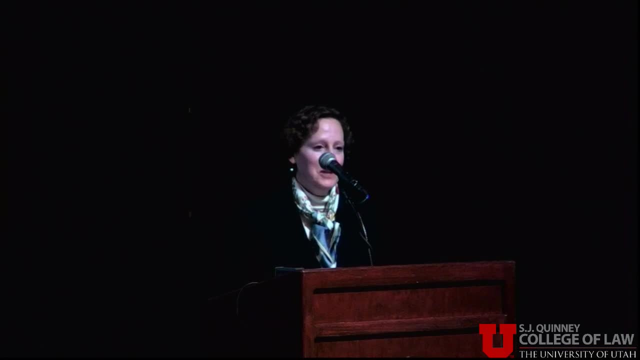 done to put this on the table. They've put together a great program over the next day and a half. I'm really looking forward to being a part of this interdisciplinary discussion. So I'm going to today continue to talk about EPA's fascinating 1-ed-11-D proposal, but 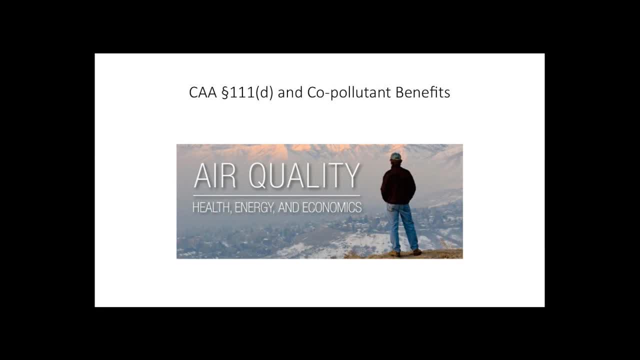 I thought since—see, I have this slide too—I thought that, since this conference is a lot about air quality and not so directly on the subject of climate, that I would use this opportunity to look at the relationship of the two, The relationship of these really new directions we have in climate policy, and how they relate. 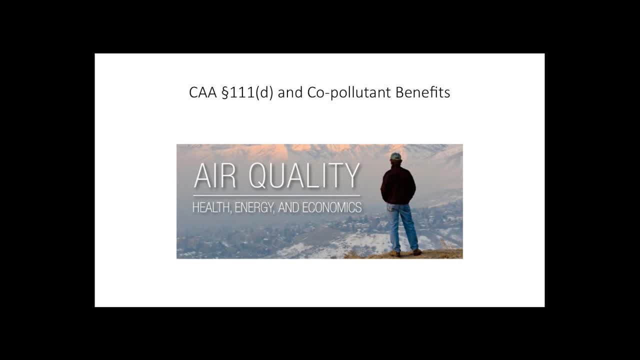 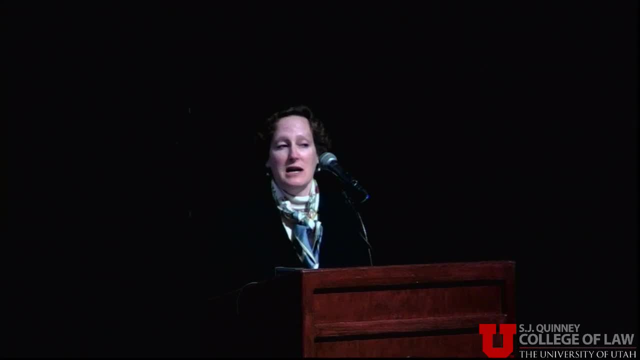 to traditional pollutants, to what we call co-pollutants, in the climate world. So I'm going to look at the implications, particularly of the existing source proposal for greenhouse gases and what it means for co-pollutants, Also be looking at some of the implications of the relationship between climate policy. 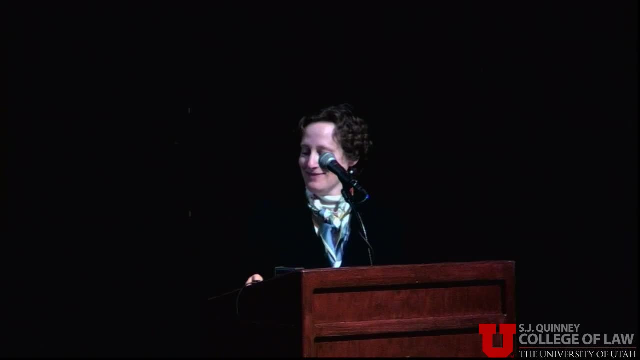 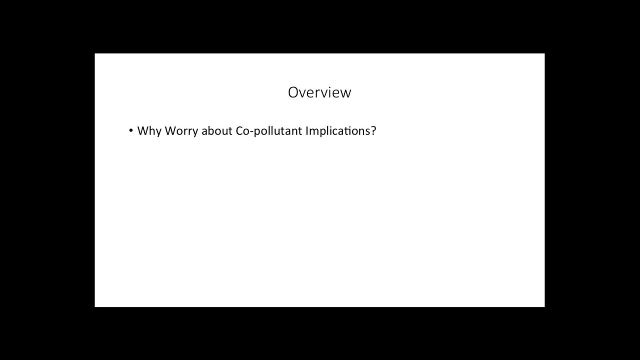 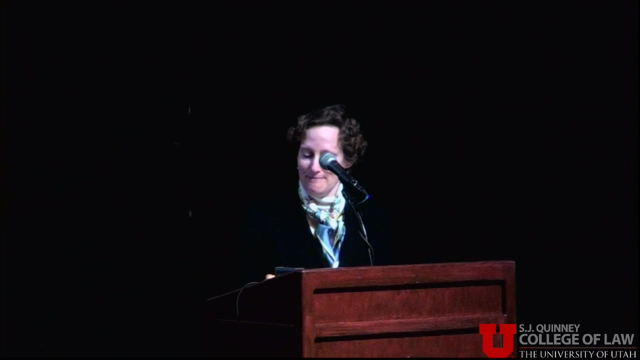 and environmental justice. There we go, So I want to give a bit of— A bit of- an overview. First is just well, if we're talking about climate policy, why should we worry about co-pollutant implications? I'm going to talk just a moment about the aggregate—a few words on the aggregate co-pollutant. 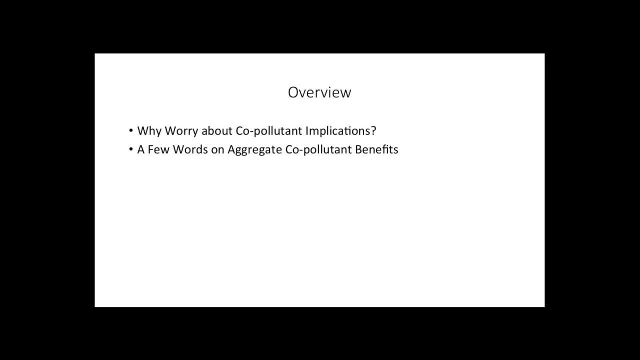 benefits of regulating existing sources. I'm going to say more than a few words about some of the distributional implications, of some of the opportunities for reducing greenhouse gases, looking in particular at the environmental justice critiques of some of the methods, And then I'm going to come back to what I think is really the central issue, if you're. 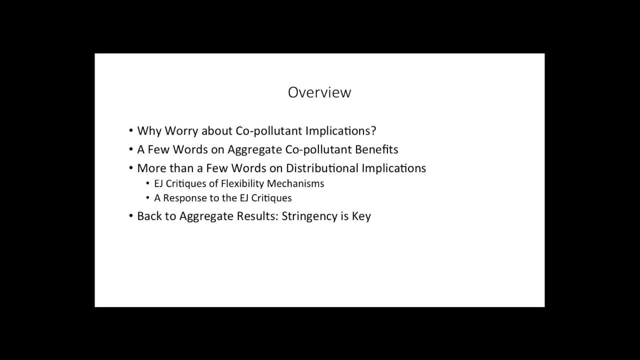 worried about co-pollutants and environmental justice, and that is stringency. And then, if I have time, I'm going to attempt to say at least a couple of words about the additional concerns that environmental justice groups have about the proposal for existing. 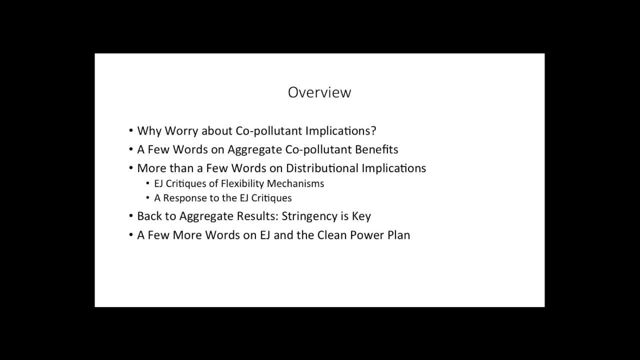 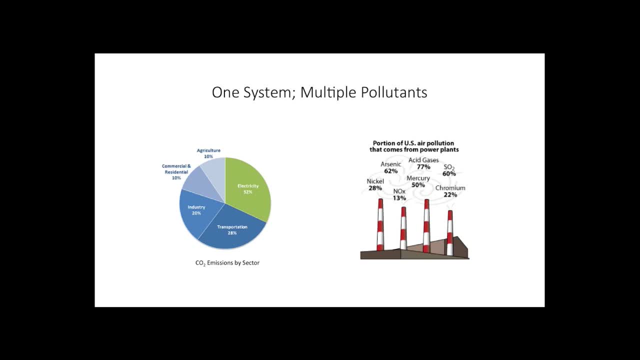 sources known as the Clean Power Plan. So let's talk about why we would worry. We would worry about climate policy's co-pollutant implications, Section 111D of the Clean Air Act and EPA's Clean Power Plan designed to implement it. 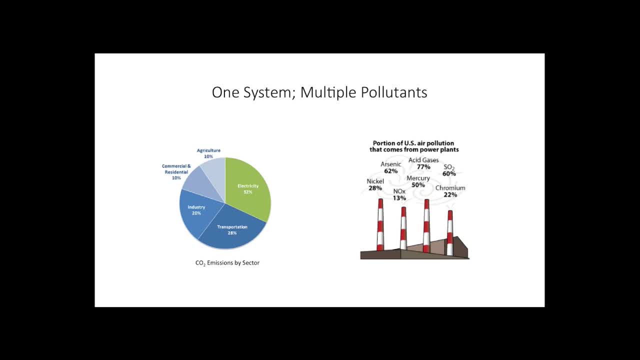 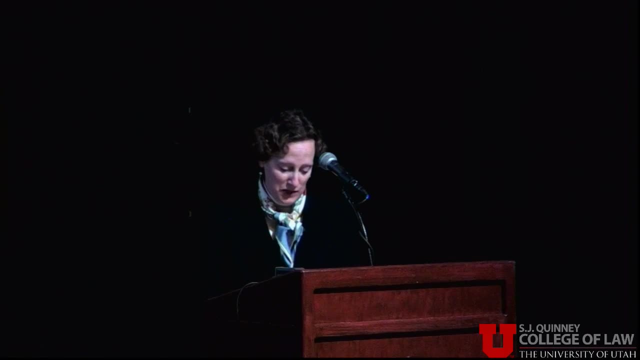 is designed to address greenhouse gas emissions, And existing power plants create about a third of the country's—or maybe 40 percent, as Ann suggested- of the nation's- at least carbon emissions, so a very major source of carbon emissions. It's also, and at the same time, a very significant source of many traditional pollutants, including 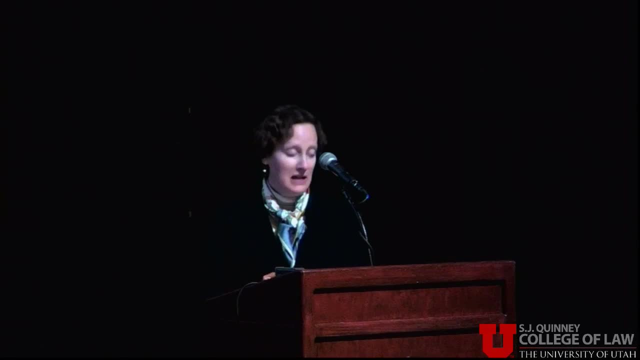 sulfur dioxides, nitrogen oxides, particulates and mercury And, as we know, all of those pollutants have very significant both public health and environmental welfare consequences. So we do have obviously other Clean Air Act programs to address these pollutants. 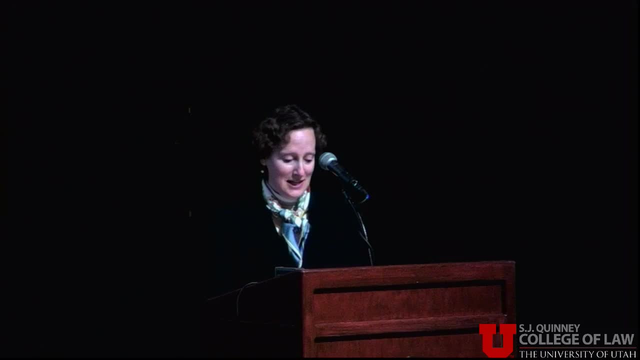 but they're not getting us all the way there, as David suggested, And so a multi-benefits approach that looks at this regulation of the Clean Air Act and the regulation of existing power plants for greenhouse gases but thinks not only about the climate benefits but about the multiple benefits that that regulation could achieve. 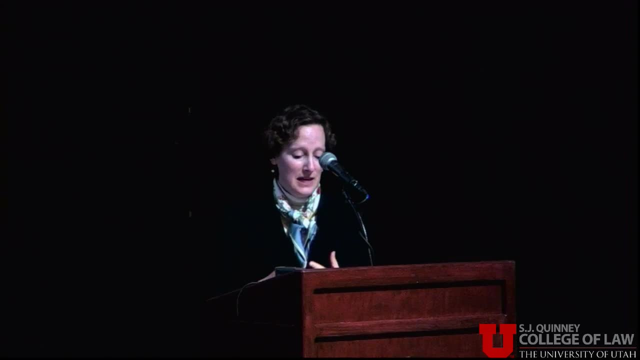 I think can capture important synergies, can give us important opportunities and ultimately provide larger overall benefits. So I want to talk first about aggregate benefits, about overall what we can hope for. Sorry, this is annoying. Who was the one who had the best—I think Bob maybe had the best technique here. 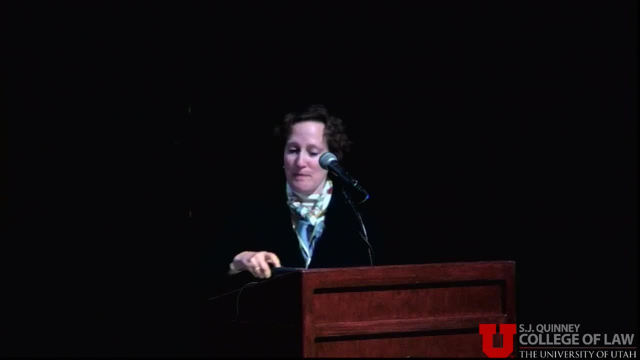 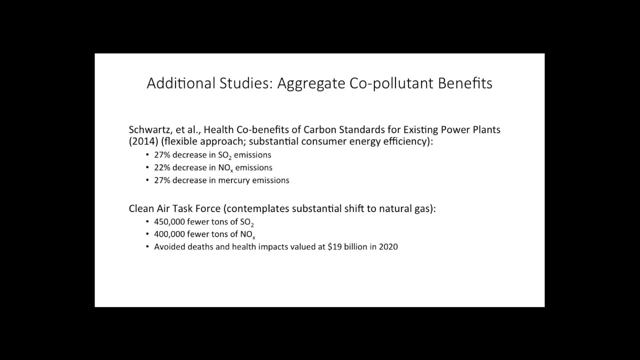 We'll see. I'm going to start with our button. Do I need to point it in a certain direction? That's part of what I'm wondering, Okay, Well, there it is. Okay. So efforts to control greenhouse gases from fossil fuel energy production will, in the 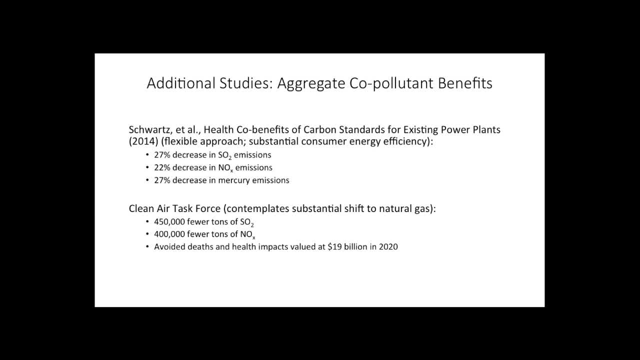 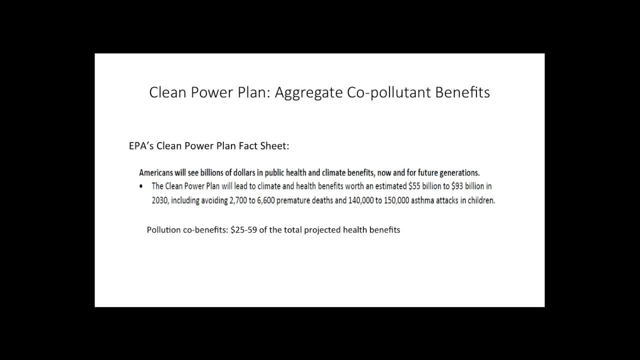 aggregate have significant co-pollutant benefits And EPA highlighted those benefits prominently. This is actually not the right slide. Prominently in its proposal under 111D and its Clean Air Act. It's a clean power plan. Now figuring out the exact benefits is very difficult because, as Anne described, there's 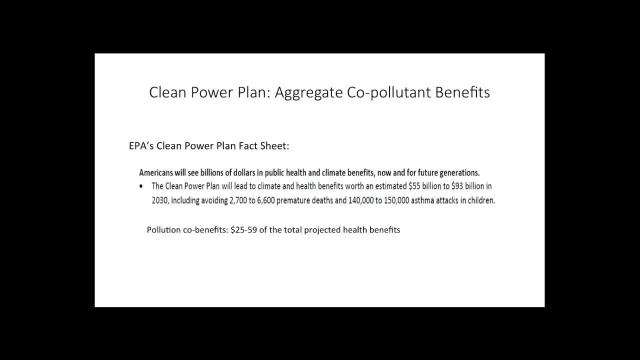 a lot of flexibility here, So we don't know exactly how emissions will be reduced, but whichever way you cut it, we're looking at a very significant potential. EPA projected overall environmental and climate benefits of $55 to $93 billion by 2030.. But the pollution co-benefits, the traditional pollutant co-benefits, are half or more than half of those, And EPA didn't even attempt to quantify, in fact, many of those co-pollutants. That's what EPA analyzed with the Clean Power Plan. 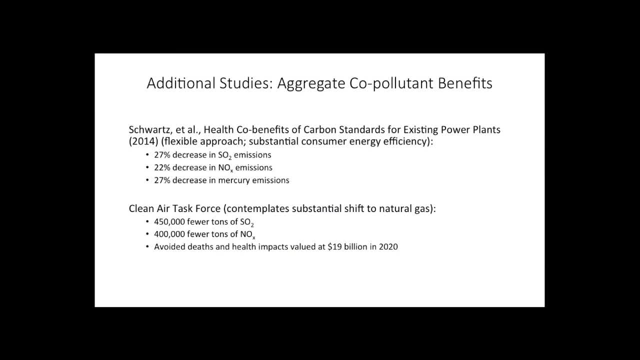 There have been several other studies that have looked at what are the co-pollutant benefits in general that we can get from regulating greenhouse gases. A big study from Harvard, BU and Syracuse done recently analyzed one option fairly close to what EPA came up with in the Clean Power Plan and showed, as you see, very significant. 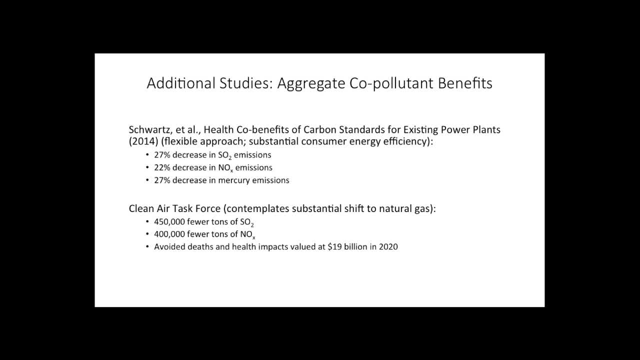 additional reductions in very important pollutants. The Clean Air Task Force with Anne also has done One study looking at an option that looked at a lot of switching from coal to natural gas. also showed very significant reductions. But from an environmental justice perspective, if we're looking at what are co-pollutant, 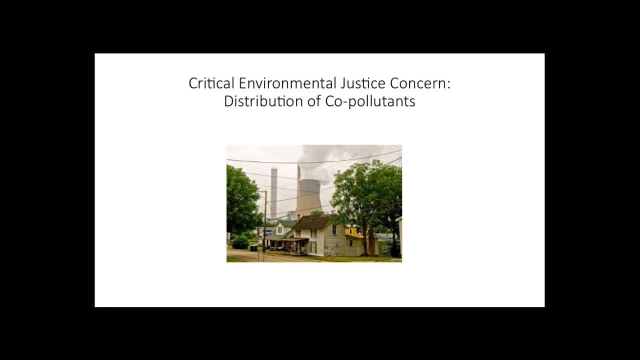 benefits. our concern is not just the aggregate co-pollutant productions, but their distribution. So reducing co-pollutants matters, but it matters most if co-pollutants are being reduced in the areas that experience the most pollution. 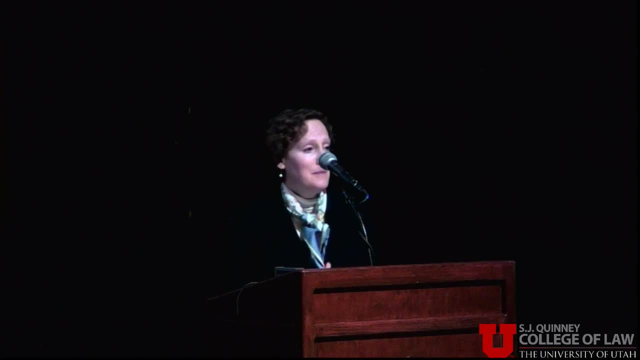 And that are most vulnerable. So, as Anne suggested, when we look at what EPA proposed for the Clean Power Plan for existing power plants, EPA proposed to give states substantial flexibility in how they would go about achieving the targets that EPA has set for them. 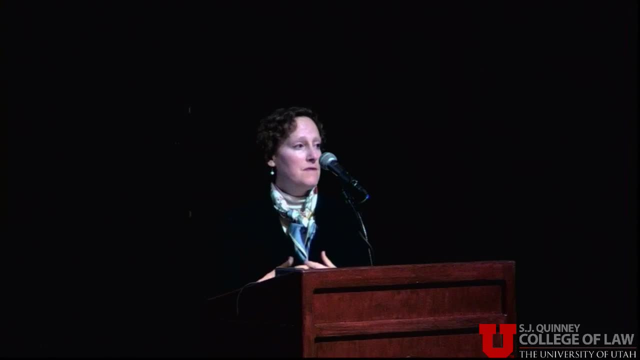 And one of the options- a fairly prominent option that EPA gave the states is to adopt a cap-and-trade approach to do so- And again, Clean Air Task Force is working on that- We'll go into more detail on how cap-and-trade could work here. 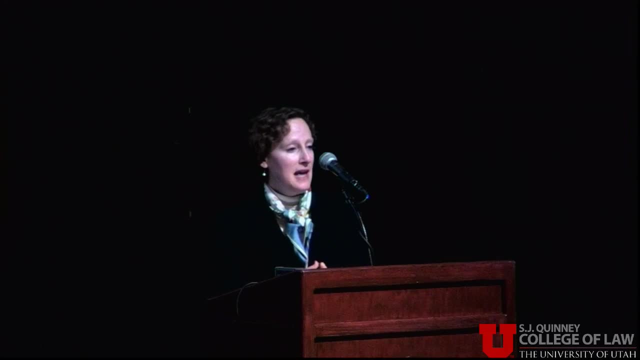 But I note that in the environmental justice world there is a very persistent and deep concern about cap-and-trade programs, particularly with respect to their distributional impacts and also dealing with an offset question. Now, that's not their only issue or concern in the Clean Power Plan, but it's an important 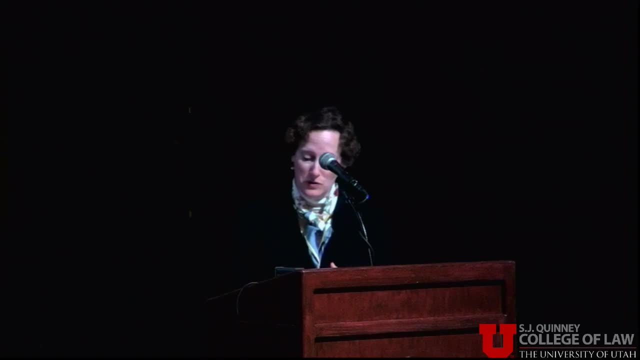 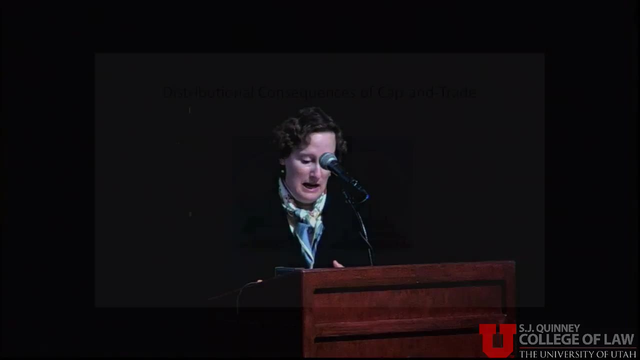 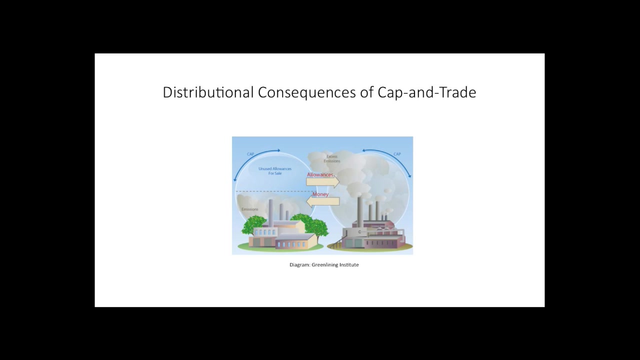 one. I actually want to spend a moment exploring it and also responding to it. So the The first question I'll look at is the issue of distributional impacts. Ultimately, a cap-and-trade program allows certain facilities to potentially buy allowances to cover their emissions right. 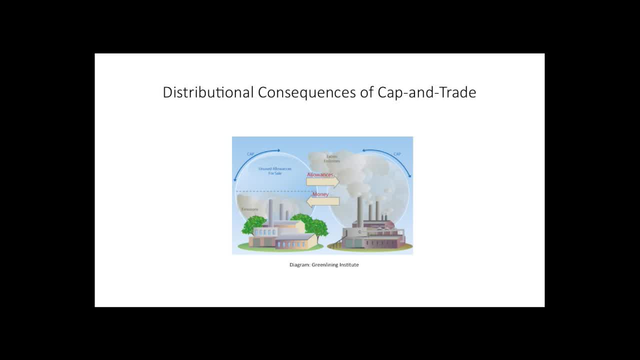 It might be the facility in Kentucky right that can't make the transition just yet. They can actually buy allowance from another facility like the one on the left that's reducing by more and they can cover their emissions. But that's a concern from an environmental justice perspective, because what if that facility 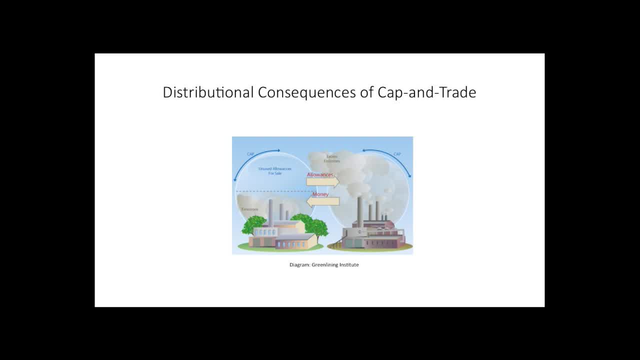 that is buying allowances. it's not going to end up reducing the co-pollutants, right? It's buying allowances to cover its greenhouse gas emissions. It might even be increasing its greenhouse gas emissions and along with that, it will either be maintaining or increasing co-pollutants. 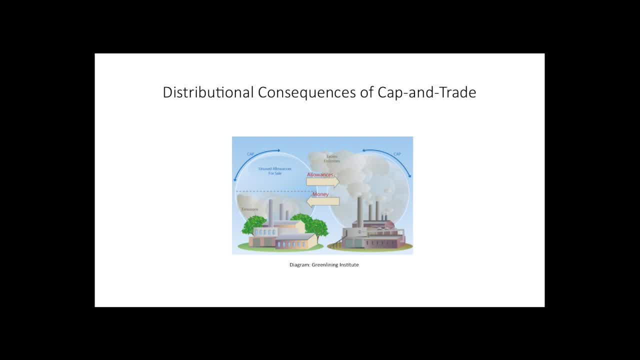 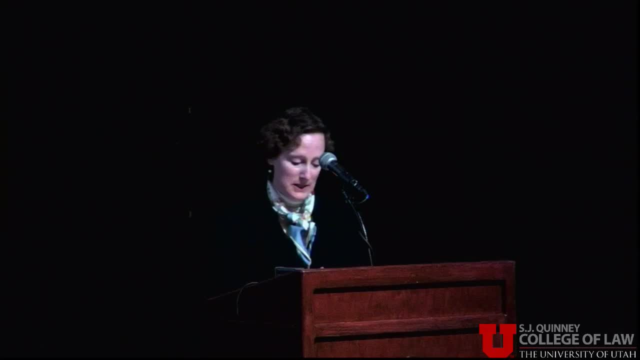 And if that happens in an area that's already heavily polluted and vulnerable, then we're not going to get as much bang for our buck in terms of achieving positive co-pollutant reductions. I have a response. Okay, I have a response to this concern. 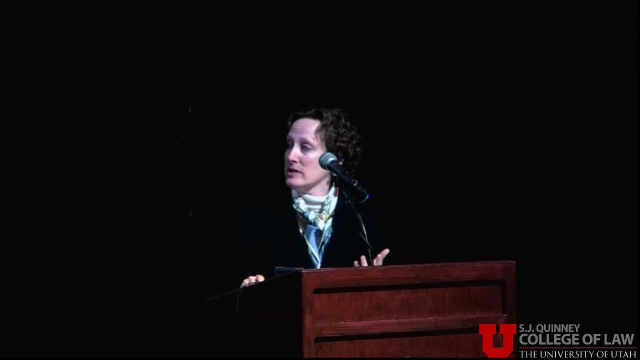 I think it's a real concern. I've written about it. I'm very sympathetic to this concern, But what we need to consider is what the alternatives are right. What are the other ways that are viable for EPA to go about controlling the actual power? 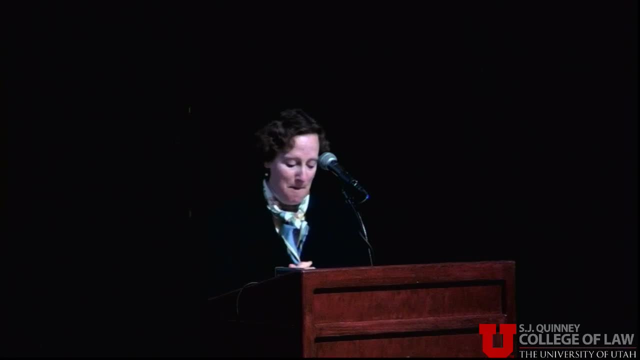 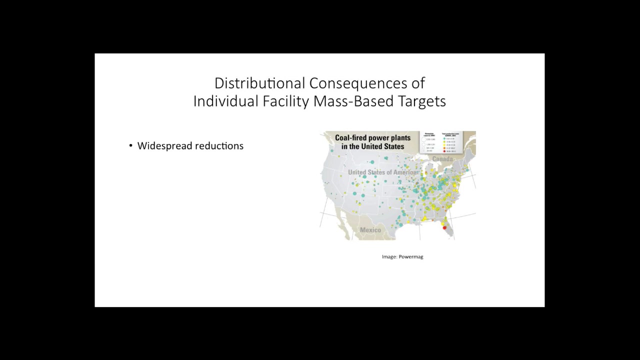 plant pollution. One option that might appear to have positive distributional consequences would be if we actually set individual facility mass-based limits on existing power plants. So I just have a picture I found on Google. isn't that a great instrument of here are? 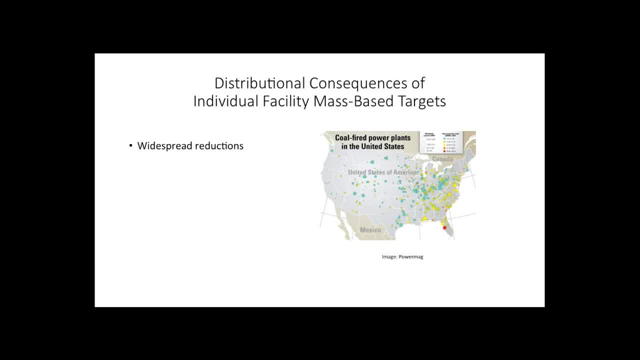 the existing coal-fired power plants. but what if we just required every one of them to reduce the absolute emissions that are coming from them? That would fairly widely distribute reductions and associated co-pollutant benefits. But I think ultimately it's not clear this is going to be anything we would ever see. 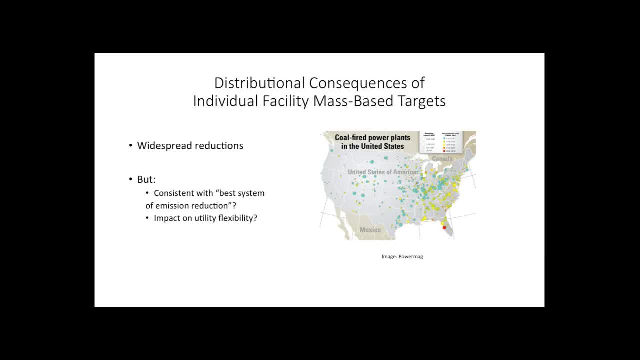 coming out of EPA. Part of the question is whether it's really consistent with what we identify as a best system of emission reduction, the standard Anne referred to, which has historically really always focused on what's the best system, what's the best technology for reducing mechanism. 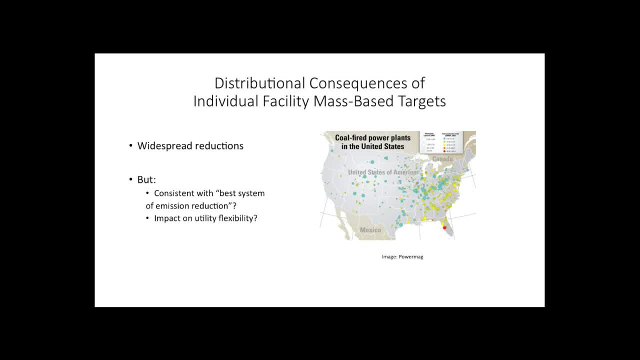 for reducing pollution, not what is the absolute amount of pollution. So to try to set an individual facility mass-based limit on a federal level, I think, is in some tension with that language, Also likely to be extremely controversial, and not that that should stop us, but utilities. 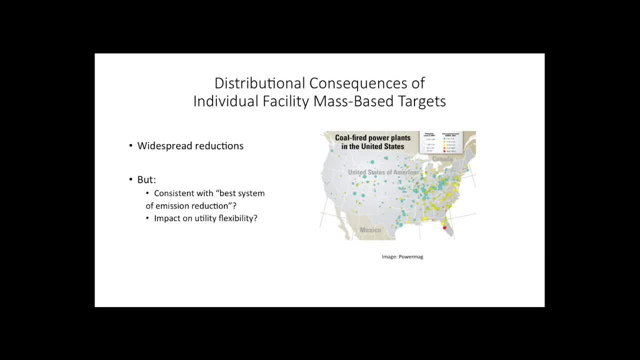 like to have flexibility And to try to set those kinds of limits on everything, Every facility, I think, would not be there. So again, maybe that would have some again widespread distributional benefits here. But I think both legally and for a number of policy reasons it's not one that's likely. 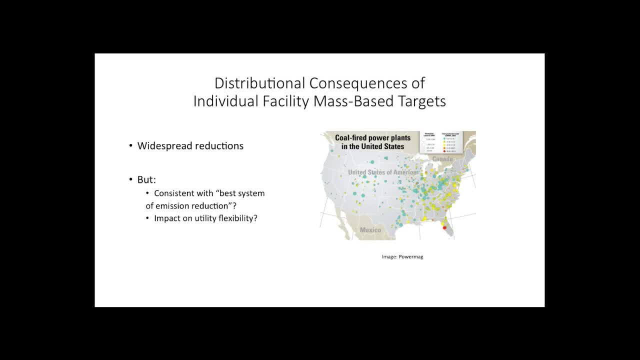 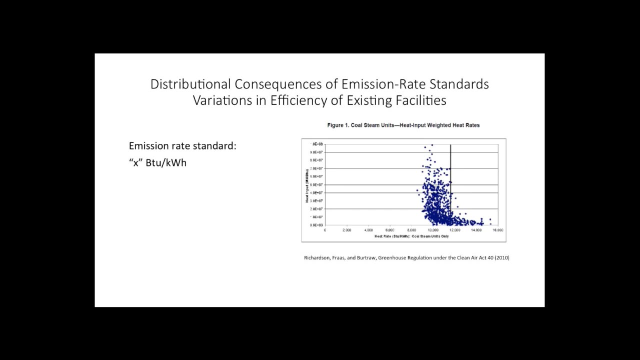 to fly. The other alternative- again if we're looking at the facilities specifically- is going to be setting emission rate standards. all right, So this is different from setting a facility mass-based standard, Where you're limiting the actual amount of pollution. 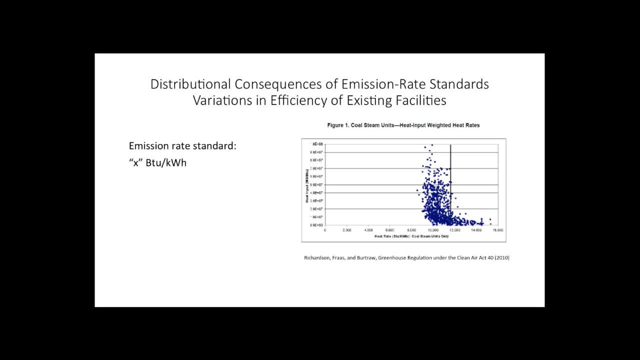 This is setting even or consistent emission rate standards for all coal-fired power plants, And this is more consistent with what we see coming out of typical technology-based performance standards under the Clean Air Act. Here again we'd be looking at setting a limit at, say, X BTU per kilowatt-hours. 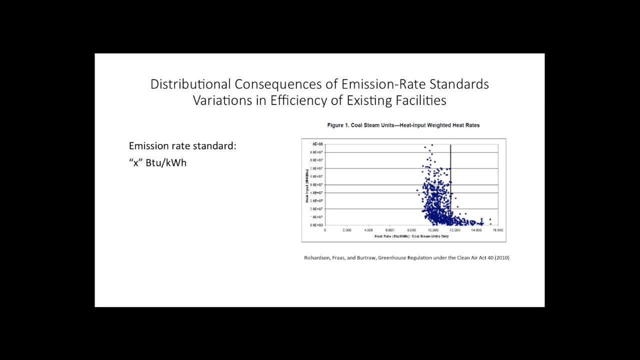 Now that might look again like: well, yeah, that would look like it's setting the same standard for everyone, And so we'd get some good distributional results from that. But here's the thing. Here's where I'm going to push a little. 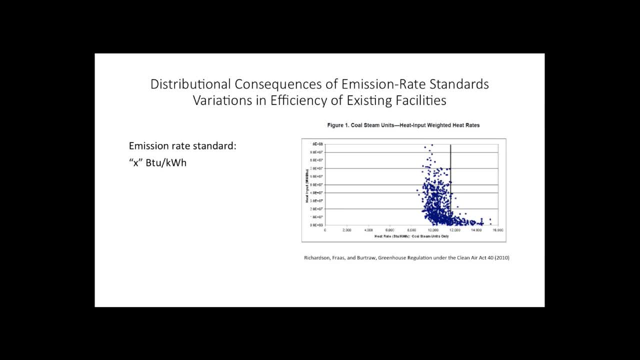 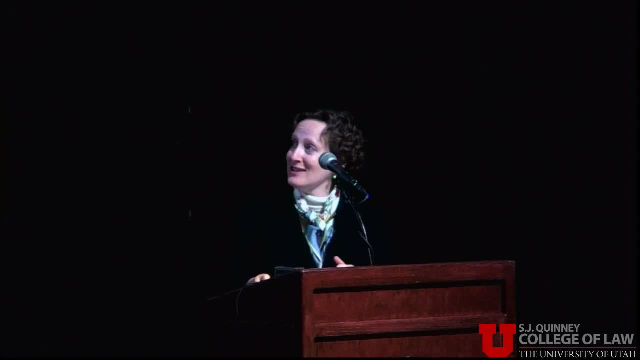 I'm not sure that would lead to positive distributional results. The first issue is that it would not necessarily lead to even reductions at all facilities, because the existing efficiency of coal-fired power plants varies substantially. So this slide shows differences in heat rate, which is an approximation for or a proxy for. efficiency. And you see there's a big range. Some existing power plants have heat rates of 9,000 BTU per kilowatt-hours, Others are almost 16,000.. So if we were to require the same emission rate standard for all facilities, then only. 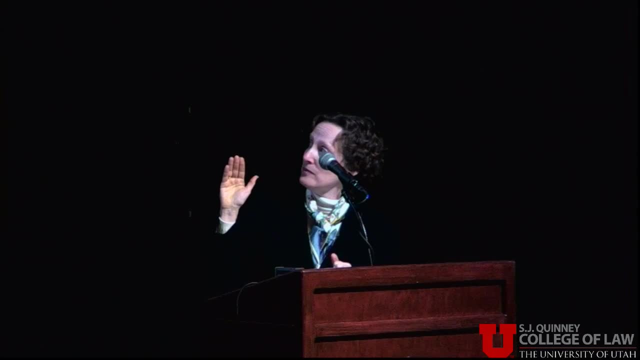 the more efficient facilities only. the more inefficient facilities, the one sort of to the right of the standard, would end up adopting controls, and the ones that were already fairly efficient wouldn't need to do anything. Right, So we would be moving toward a greater evenness in emission rates across the country. but 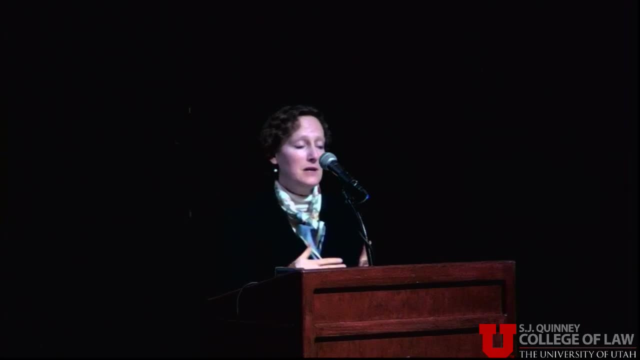 we wouldn't see reductions at all facilities. The facilities that are already fairly efficient would not have to do anything, and so we wouldn't see – and we can't expect distributionally that the clean power plant would lead to reductions everywhere, because it would only happen at the more inefficient facilities. 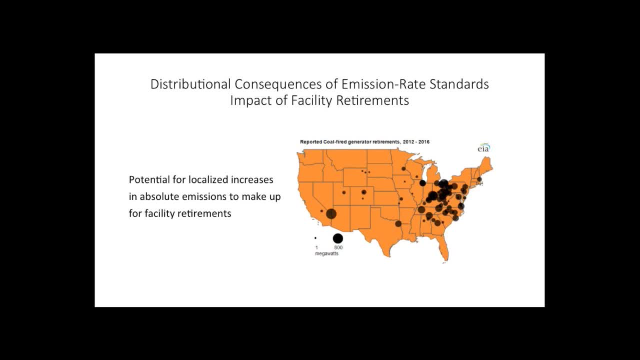 Okay. So the other issue is that we have a – we have an emission rate standard and not an absolute emission standard, Okay. So if you're only controlling emission rates, you're really not controlling the absolute volume of emissions that occur. And in an interconnected energy system, if you have major shifts in production from one 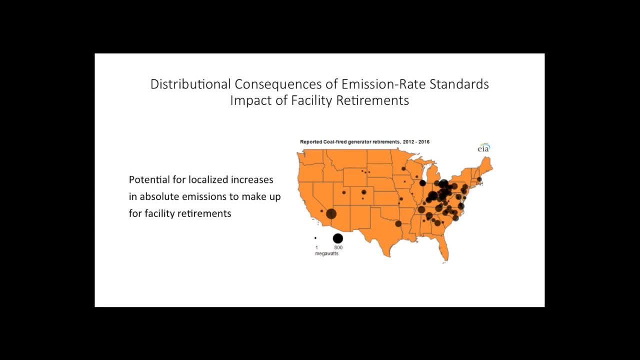 – if you have – you can have major shifts in production from one facility to another, And so you could end up even if you've got an even emission rate standard across the country. if you decrease emissions in one place, you can have them pop up in another. 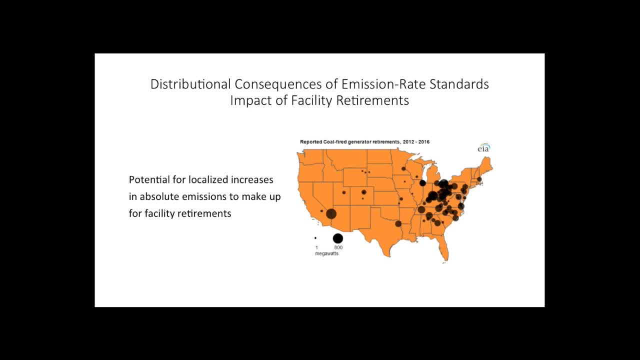 even if everyone has the same emission rate standard. So one way that could happen is if we end up with a lot of retirements of coal-fired power plant, Analysts are expecting that. you know, if we were to impose emission rate standards, or even if we don't impose emission rate standards on facilities, the less efficient. facilities right. the ones on the right of the preceding slide are going to retire rather than improving their emission rates, And that means that other plants are going to start emitting more to make up for the lack of supply. Okay, And that's a really important piece of that. So again, you know from the places that have retired. So facility retirements, then, can lead to substantial increases at power plants, even though they may have become more efficient. The other potential impact is called rebound, and that is a consequence itself of assuming. 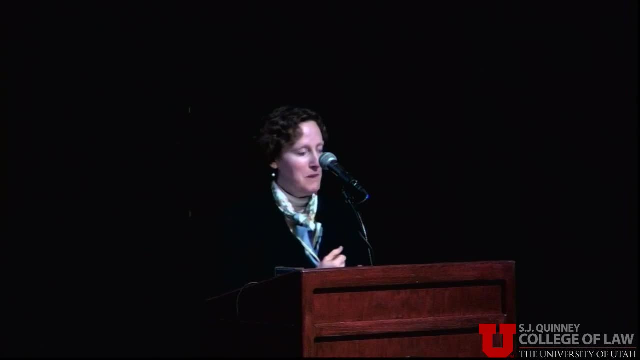 that facilities make efficiency rate improvements. Okay, We're going to invest, We're going to make them more efficient, we're going to become more efficient. But if facilities invest in making their units more efficient, then they may run them more. right, We put the money we used to just run this one a few. 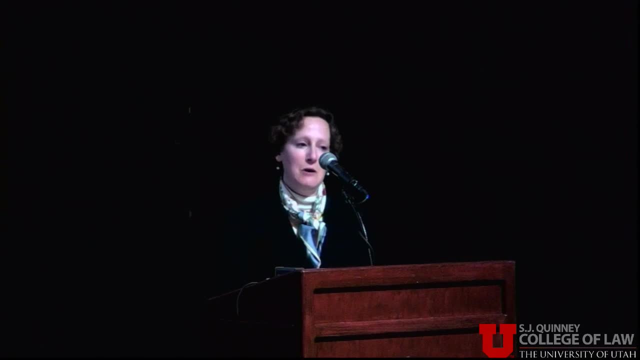 hours a day, but we put the money in. now we're going to run it 18 hours a day, And so you could end up with some coal-fired power plants in fact running more and polluting more than they used to. 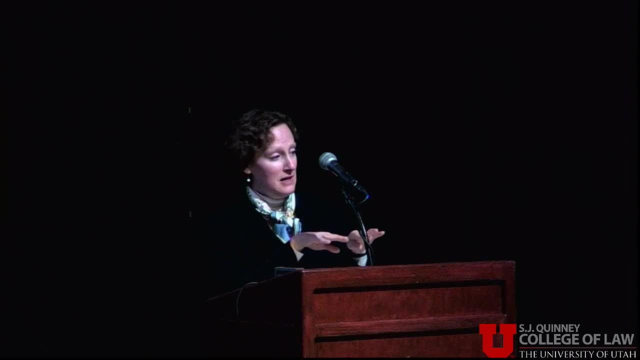 even though they're more efficient, right Lower emissions rate but higher absolute emissions. And this effect could be so strong that one of the studies done on co-pollutant consequences said that if we were to adopt emission rate standards for all facilities, 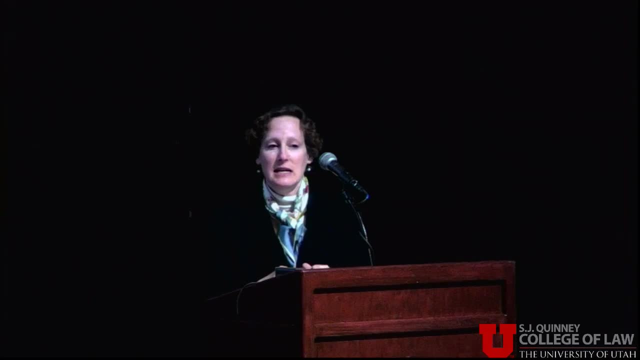 and they ran a model and a projection, we would see an increase in sulfur dioxide emissions because of the rebound effect of choosing to run those coal-fired power plants more. So I think ultimately traditional source-specific emission rate requirements are not, even though they look like they're going to create something fairly even distributionally, won't. 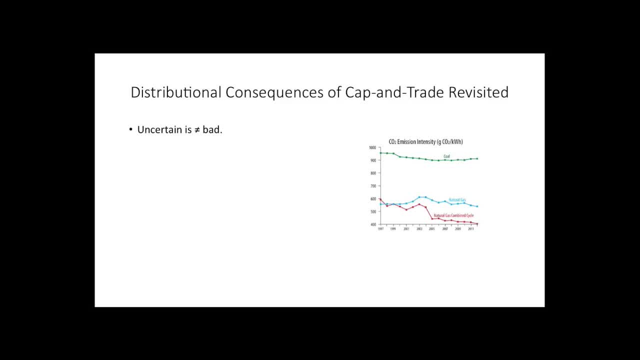 I want to also look at cap and trade again. So again that an early picture showed that we give people the flexibility to buy allowances, we can have increases in emission and that is certainly a real risk, But it creates uncertainty. We're not sure it will be bad, For example, in the 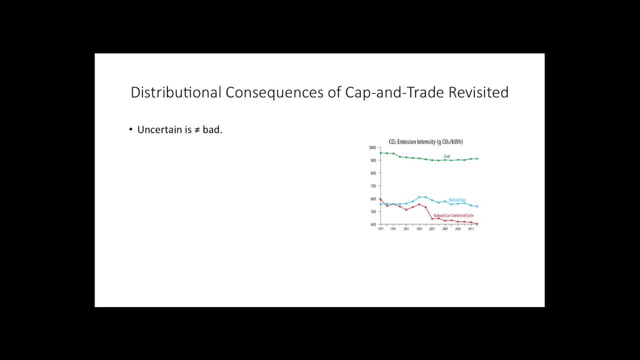 acid rain program. we actually ended up with some fairly positive results, even under that cap and trade program, And also we in fact can make some predictions about the future of carbon dioxide, and we can make some predictions about at least how a good cap, a well-functioning cap and trade 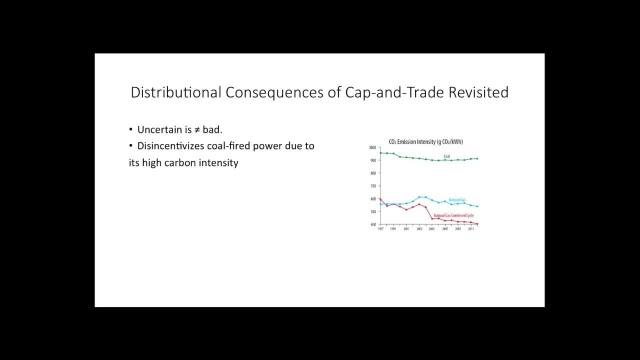 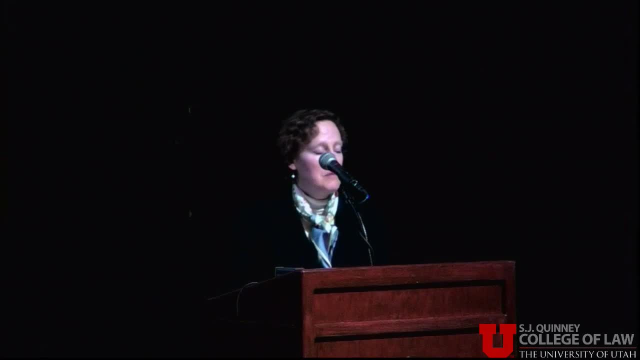 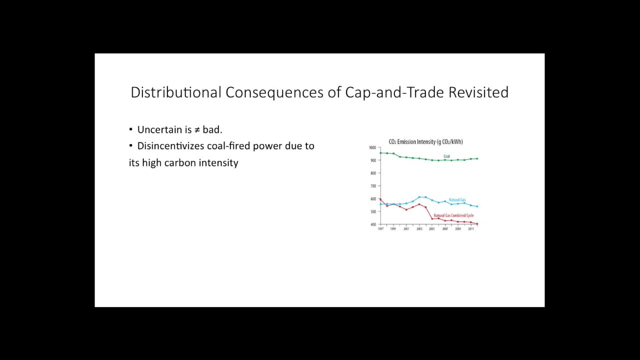 program would work. Sorry, Okay, And that is by observing that coal-fired power is in fact the most intensive greenhouse gas source. I show the emissions in the chart on the right. It's much more greenhouse gases per unit of energy. So if we have a carbon cap and trade program, 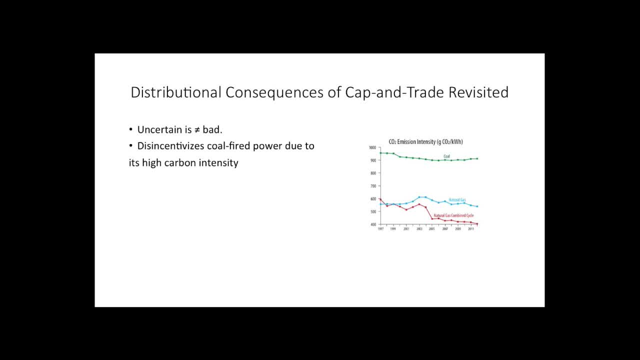 and it has an expensive price for carbon allowances. it's going to discourage generation of coal-fired power because of its high carbon intensity. At the same time, coal-fired power is also the most- excuse me- co-pollutant intensive form of energy. So we're going to be encouraging. 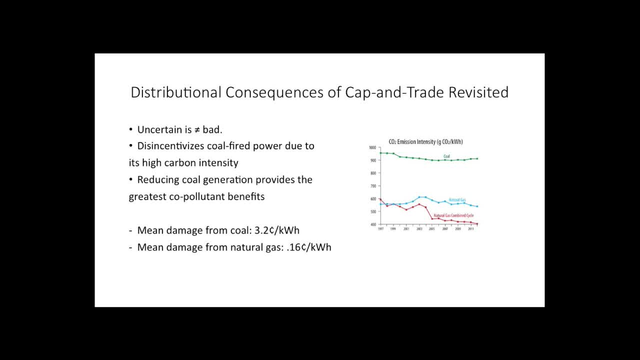 discouraging. if we have a good cap and trade program, we'll be discouraging coal-fired power And the indirect effect of that is we'll actually also be discouraging, discouraging the source that has the most co-pollutants, So distributionally we will be. 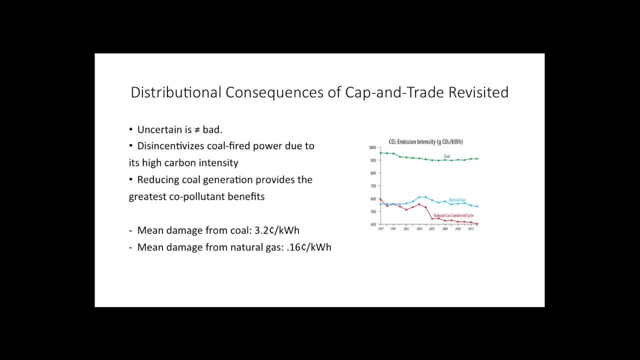 in fact, through a robust cap and trade program encouraging reductions at the sources that have the most co-pollutants, which is at least something of a positive distributional result. Now, the accuracy of that prediction does depend on a couple of things. One is that you have a 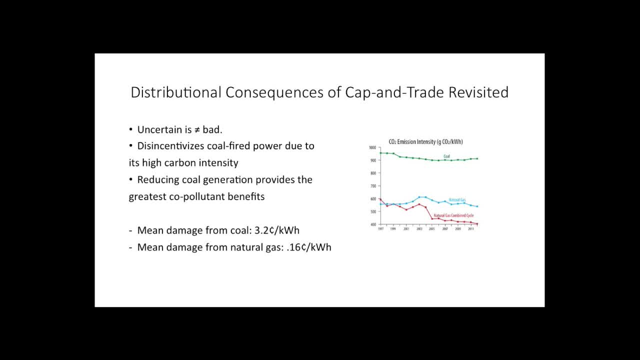 stringent enough cap and trade program that you're really going to create incentives for reductions and not just buying a lot of allowances, And the other thing is that you're going to have a and second- and this is an issue that varies by state- is how sensitive the utility is to price. 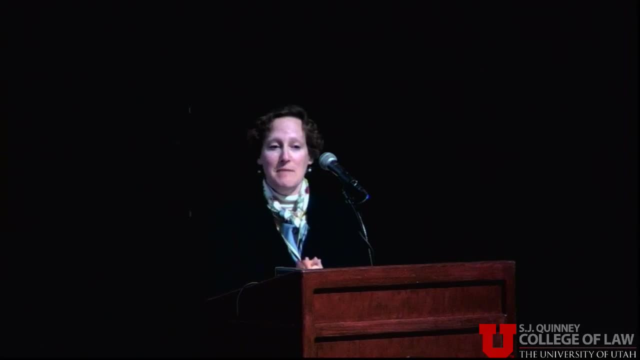 Some utilities are not that sensitive to price because they can pass along all the costs, But at least in some states there is price sensitivity, which will mean that a cap and trade can send the right signals. So ultimately, on the distributional issue, then, I think that 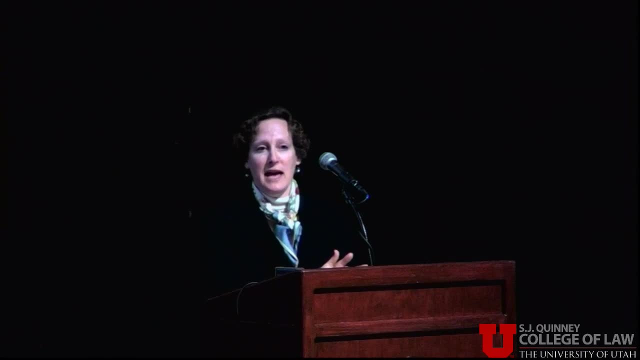 even though there are concerns about the distributional consequences of cap and trade, there's actually when we come to like: what are we going to do about existing facilities? there's no quick fix That's likely to be adopted that will necessarily have dramatically superior distributional results. 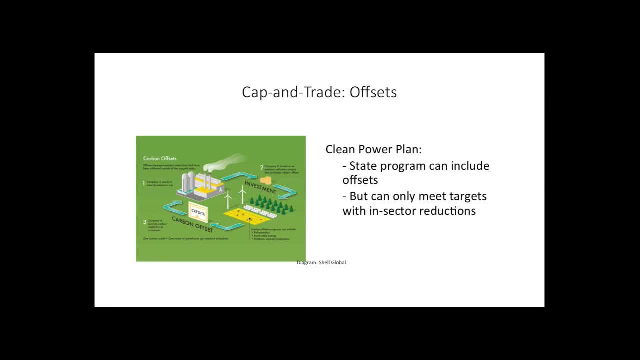 There's another concern that comes up a lot in the cap and trade debate and that is the use of offsets. Offsets allow a facility to avoid making actual emission reductions by purchasing offsets that represent reductions elsewhere. But here the reductions elsewhere are not at another power. 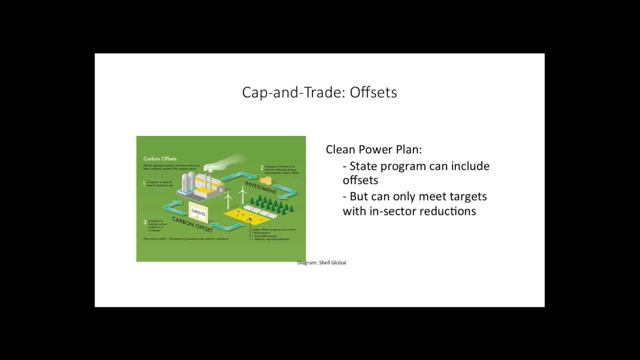 plant. They're some other mechanism for either reducing or capping the emissions. So if you're going to buy a power plant, you're going to be capturing carbon. So it could be a foresty project, right, that is going to sequester carbon, And then a power plant can buy the offset from the. 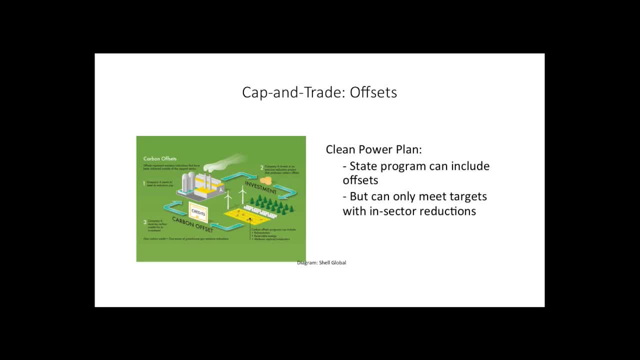 timber company that represents the sequestered carbon, and they can keep generating power and generating both greenhouse gases and co-pollutants. And from an environmental justice perspective, that's a large, a big concern, because it means that even if you've 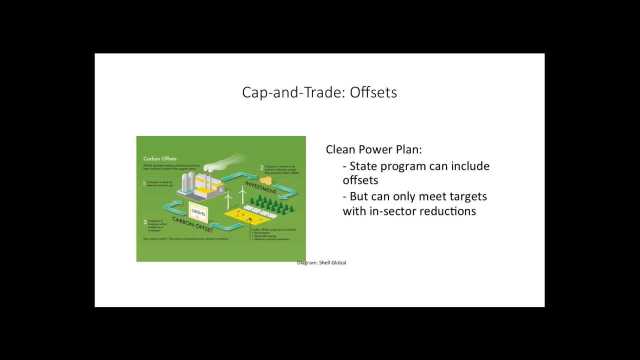 you know, technically reduced carbon, you haven't gotten any co-pollutant benefits. But I think this is not going to be an issue, at least as the current, the Clean Power Plan is currently proposed, because the Clean Power Plan is saying that you're going to have to show. 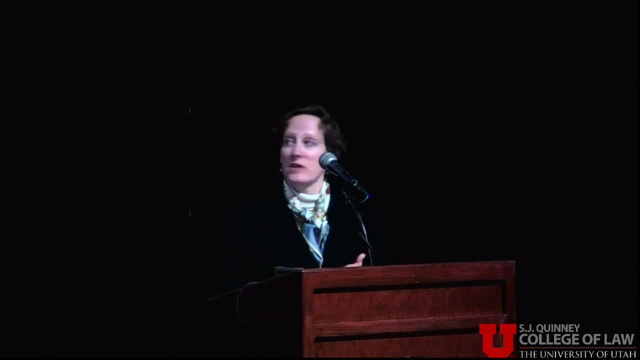 the reductions have come from the electricity sector right. So even if the state program has offsets still at the end of the day, for proof for purposes of the SIPP, the state instrumentation plan, you're going to have to show electricity sector reductions. So this is: 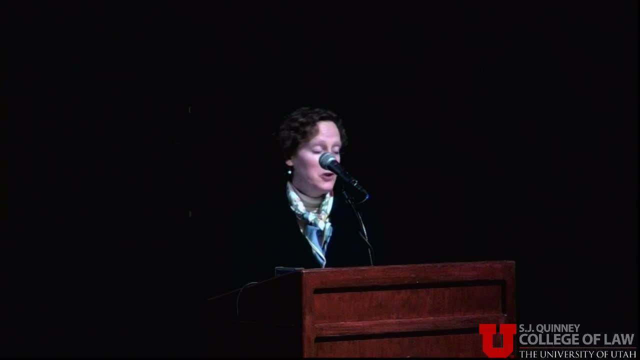 again a very strong concern about cap-and-trade programs in the environmental justice community, and one that I think is not as much of a risk here. in this context, What I do think is fundamentally important in order for there to be good co-pollutant consequences and good distributional 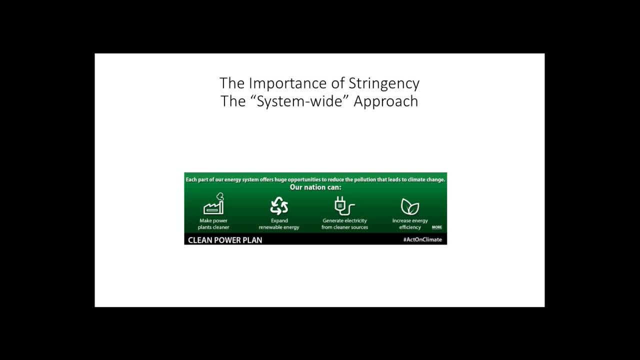 consequences is going to be that the system is stringent enough. So I think the question of form right- is it going to be emission rate standards? Is it going to be cap-and-trade? I think that question is ultimately less important than whether we're going to have a really stringent. 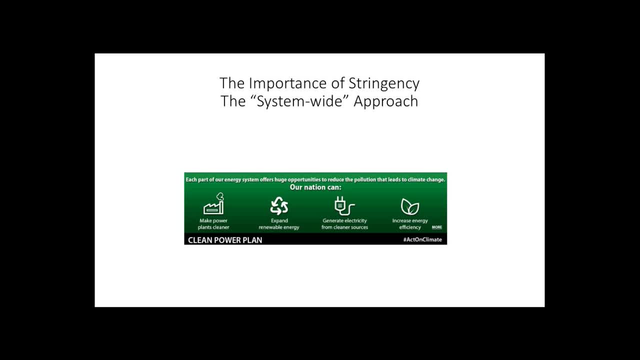 program that is going to maximize greenhouse gas reductions and, as a consequence, also maximize co-pollutant reductions. Stringent targets are going to be essential to have transformative change right. So one of the great things about what EPA has proposed is that it's not just tinkering with coal plant emissions. 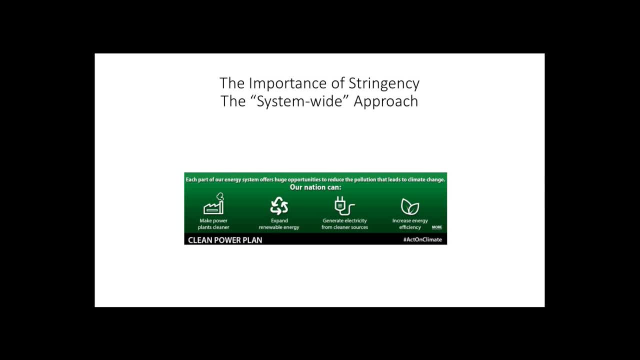 let's increase the efficiency a tiny bit. It's taking the system-wide approach that allows the agency to evaluate all of these different, very useful mechanisms, very important mechanisms for reducing greenhouse gas, mechanisms including ones that have no co-pollutant impacts, like 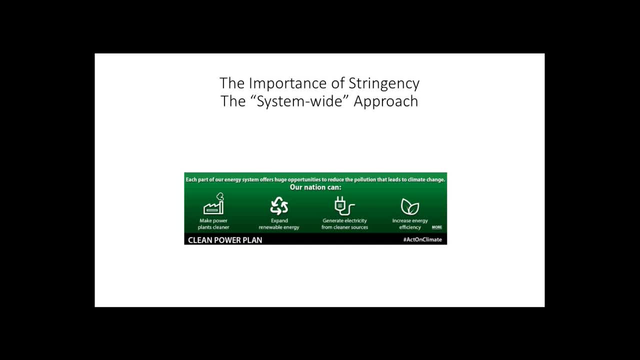 renewable energy and then, of course, reducing greenhouse gas emissions. So I think that's where we want to end up, right, I mean, that's where we want to end up, but we need to have targets that are going to be stringent enough to really push transformative change in order to see both. 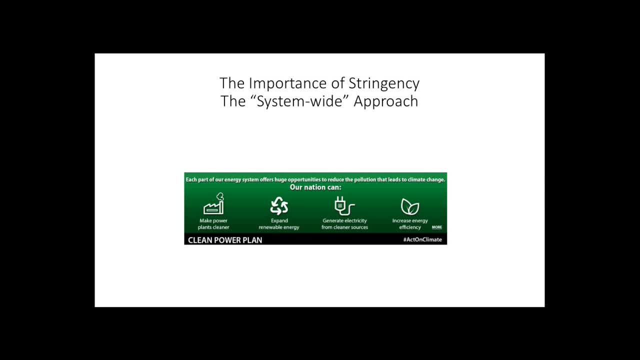 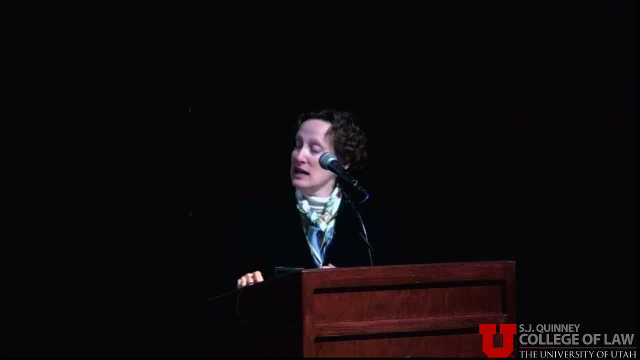 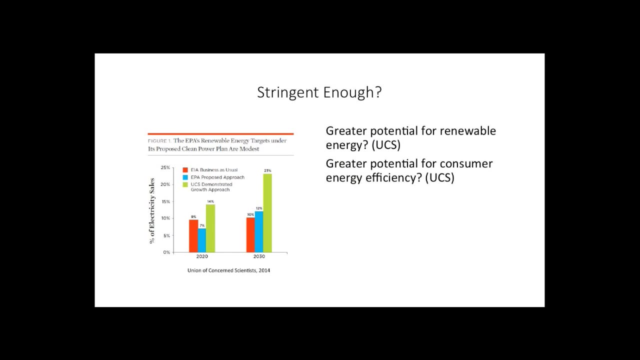 the greenhouse gas reductions and the co-pollutant benefits, And I think the question we have at this point is whether what EPA has done in terms of setting state targets is stringent enough. So there are again targets set for each state, but many have been suggesting- I quote here: 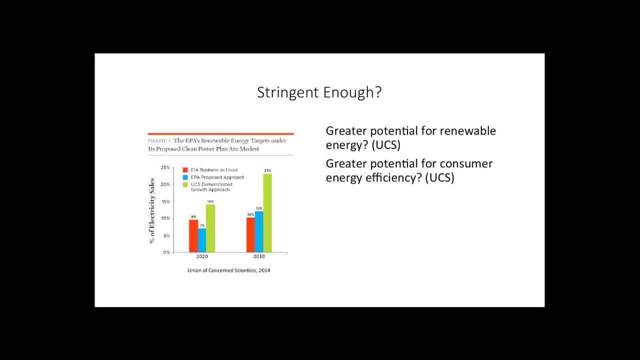 Union for Concerned Sciences. whether EPA significantly underestimated the potential for renewable power or the potential for energy efficiency, EPA was very clear in each of its building blocks that it was not going for the maximum. It was shooting for something less than that. Did they go far enough? Did they include the CG fundamental in the elementary level? Did they include the? lighting in the High low levels I mean either. the healthy living spaces- I'm not looking at the primary buildings- the greatness on the. Did they include the Organization and the development of the aquifer and the action on the gas bomber? Did they include the original Methylатine and the? 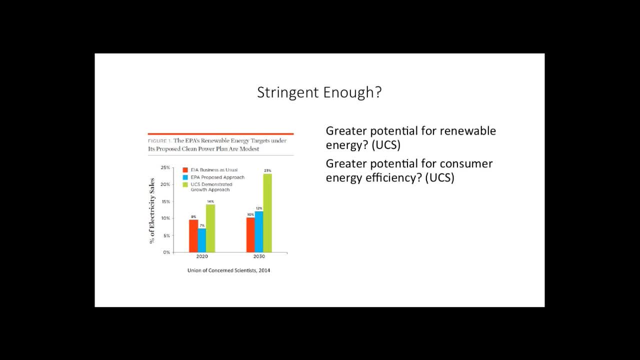 質 contact And even again, building blocks that are kept in Washington surrounding the大概 percent of estado ABGYS population is much less than an abysmal ungefähr of cost off the sagen if Did they include as many of the options as are out there in setting those state targets. 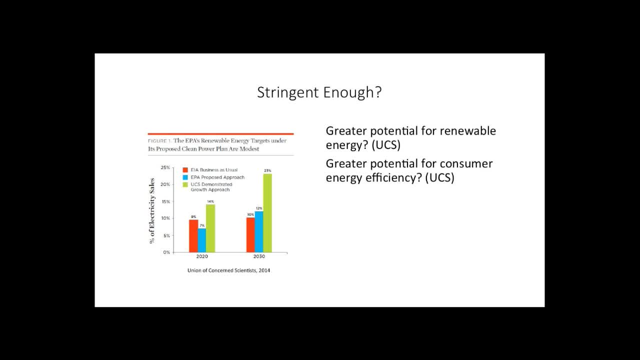 And if they have really underestimated what's possible, then we're not going to get as much. We may just get again facilities buying allowances, for example. We may just get a shift to natural gas right. We may get states recognizing that the easiest, simplest sort of less controversial mechanism here is to do a little less coal-fired power but to keep going with natural gas. And again, lots of less co-pollutants with natural gas and certainly some major benefits over coal, but plenty of its own environmental problems and some real questions about whether it's going to provide the impetus for the kinds of transformative changes to get to the energy efficiency and the renewables that we need. 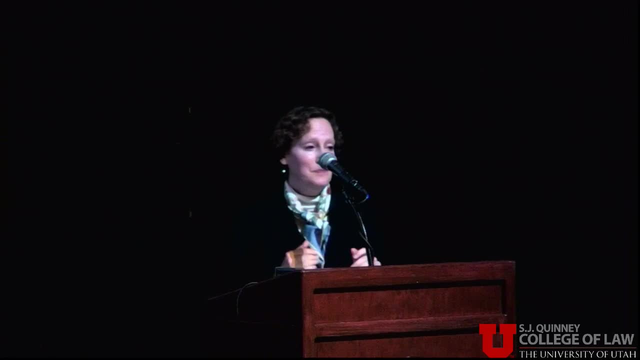 So I think we've got real questions about whether the state targets are stringent enough, And I think if we're worried about co-pollutants and about environmental justice, that's really where a lot of the attention is. I'm not an engineer so I can't provide the definitive answer on those questions, but that's where I'd really like to see a lot of discussion and energy placed. 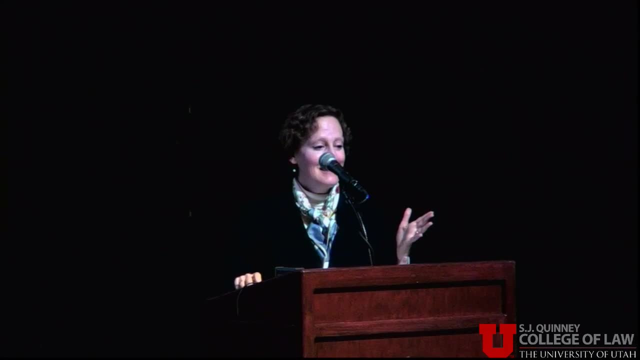 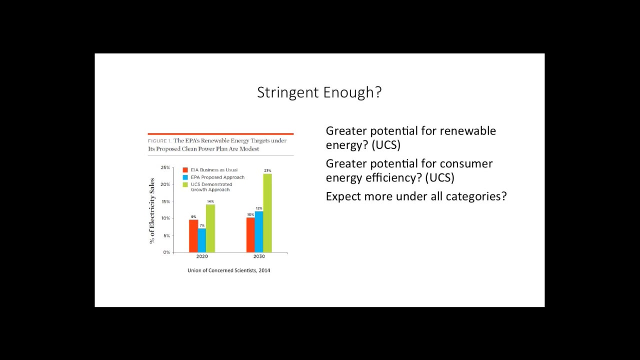 I actually don't know how much time I have left. I'm done, Okay. well, let me just put a sheet over there. I was like, oh, thanks a lot. No, So I don't want to take up time from your important questions, so I'm just going to flash through a lot of other EJ arguments here. 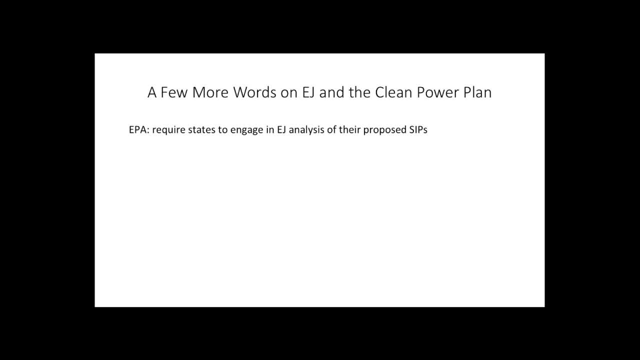 One is: I think environmental groups have suggested that states, in doing their state implementation plan, should have to look at the distributional and environmental justice implications of their implementation plans. I think that is something that would benefit all the states in their analysis. And then I think there's huge room for state advocacy at the state level. 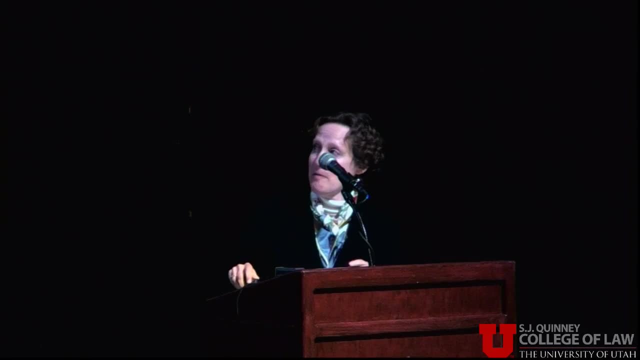 While there are many things I think can't be sort of asked for, of EPA as a federal matter, I think states that advocates can get in there at the state level and say let's retire the really polluting facilities and the really bad, Let's really focus our energy policy on what's here. 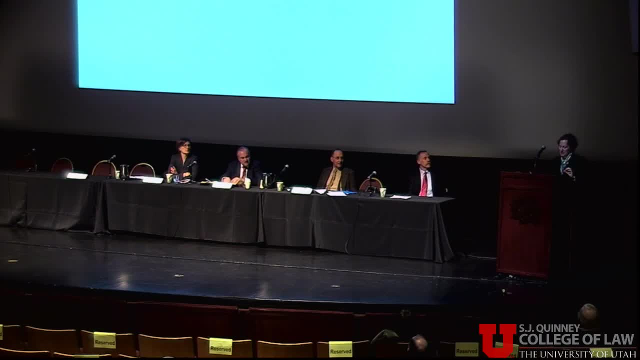 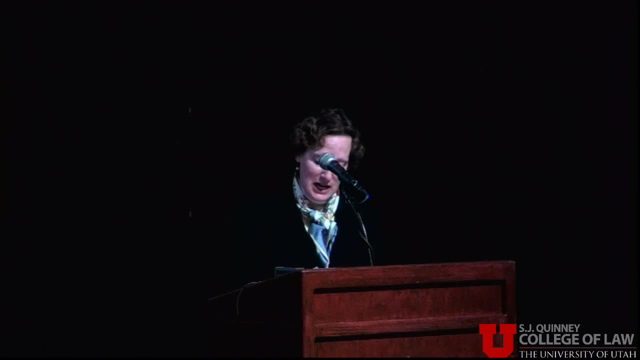 I'm just going to say them. I'm not going to try to do that anymore. So states can really focus on promoting renewable energy and energy efficiency rather than just shifting to natural gas. They can encourage investments in low-income neighborhoods that might not have the resources to do renewable or energy efficiency. 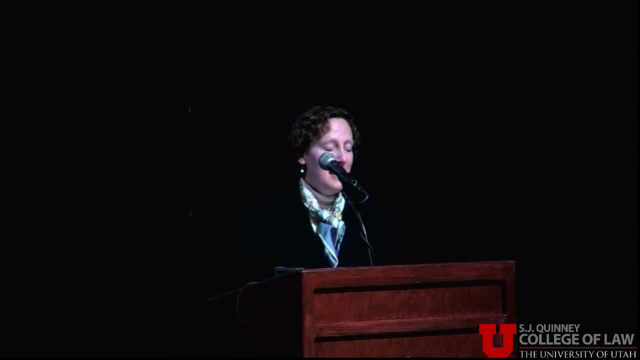 If cap-and-trade programs are adopted at a state level, they can argue for either limitations or they can see whether some of the value that comes of cap-and-trade could be directed to the most vulnerable communities, as is done in California. So, ultimately, I think there are huge opportunities in terms of traditional pollution. 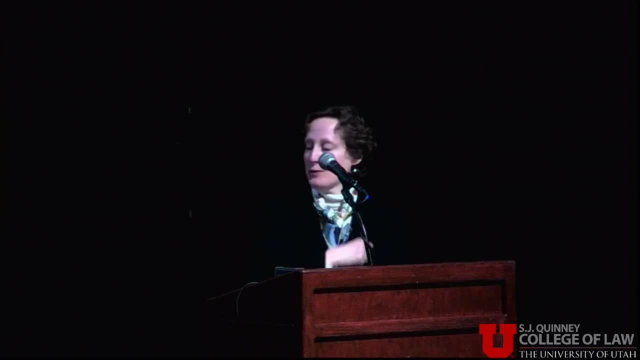 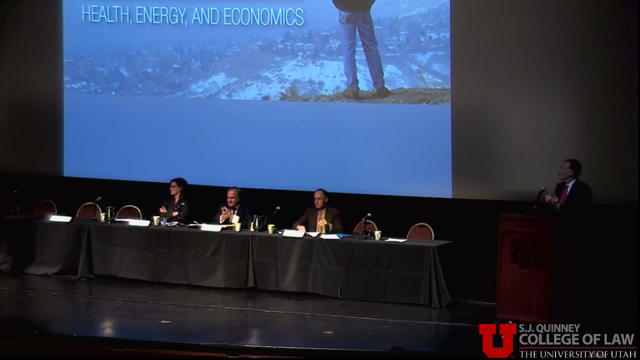 that come out of EPA's new efforts on the climate front and I look forward to your questions. Thank you, Thank you. We're going to take about 10 minutes of questions. I would ask simply that you keep your questions succinct and to the point so we can get to as many as we possibly can. 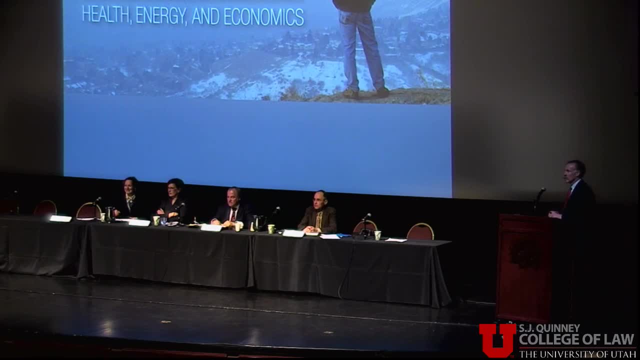 Yes, sir. Could the panel compare cap-and-trade to an offsetting tax program? You mean by offsetting tax, you mean like a tax on pollution, tax on carbon, Carbon tax? Yeah, I mean, I think— I think that carbon tax would be preferable. 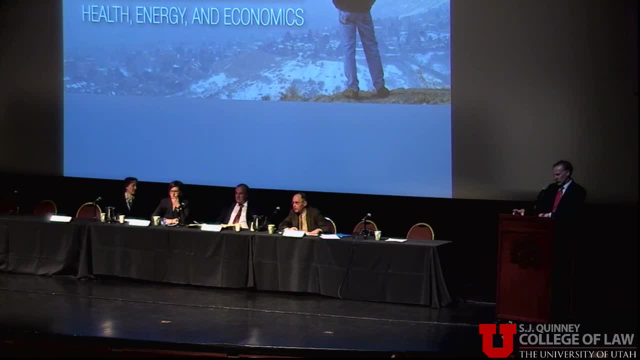 There would be more flexibility in adjusting to changing circumstances. The problem is the word tax, But I mean you hear Republicans talk about it in terms of cap-and-tax, but you know our existing system basically is a tax that's just a bigger tax than cap-and-trade would be. I think that the carbon or the pollution tax would be the best way to go, but that's supposed to be the most difficult. Yeah, I think that—I'm not an expert. I haven't studied a carbon tax per se to see what kind of benefits you would get from that. 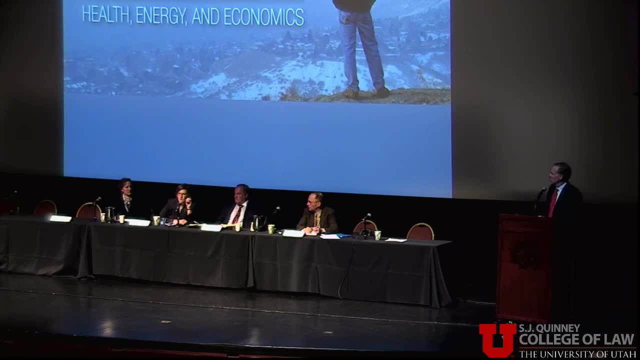 A carbon tax, though would be—you know, I guess you could make it industry-specific. What we see when we're looking at this is that we don't need the Congress to make a choice. Right now. it seems like we're going to have to make a choice. 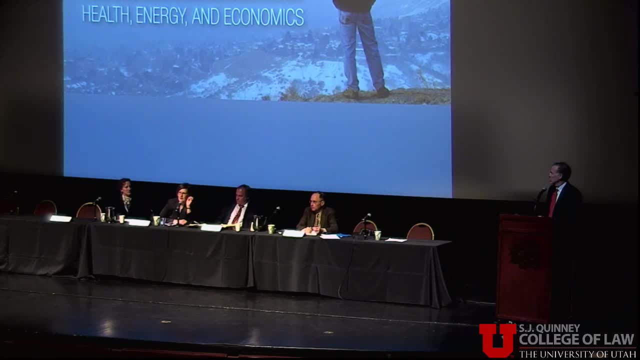 Right now, it seems like we're going to have to make a choice. Right now, it seems like we're going to have to make a choice. It seems like the Congress can't make a choice, can't do what needs to be done. 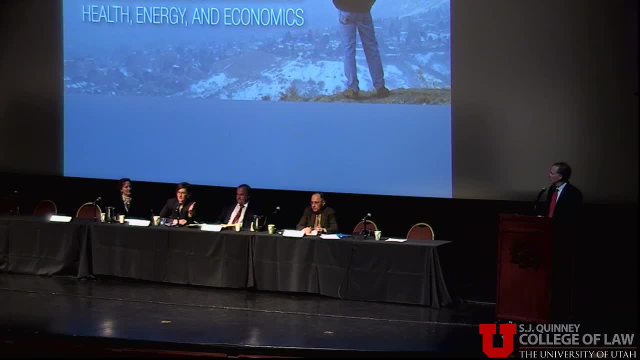 We saw that with the attempt to try to get a national system some 10 or so years ago. It didn't work even then and it's really not going to work now. It's just one woman's perspective on it And I think it's very important that, as we've all said, I think in some way or another, stringency matters. 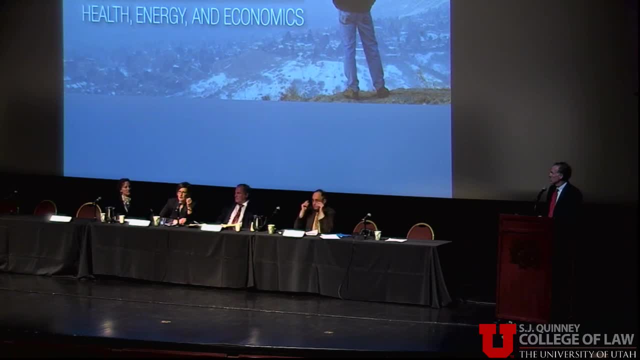 And if you're talking about— If you're talking about- putting a tax on one of the fundamental elements of our economy, you may not get a stringent enough signal, economic signal, Whereas here it's very clear: you can tie the pollution in question to its source and require reductions. 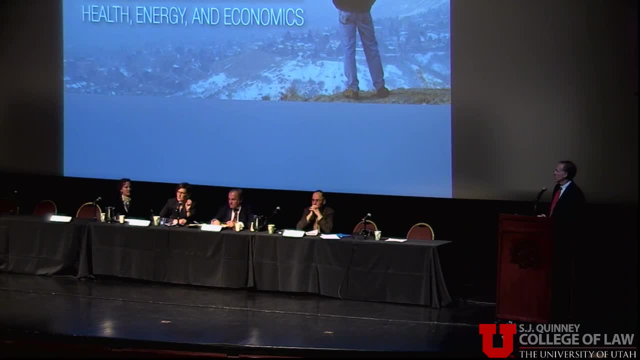 If the agency has the political will to do that, you can actually see some innovations. If the agency has the technology, that may get us even further, which is what we saw with the acid rain program and the other uses of the performance standard sections- gets us actually even further than we expected. 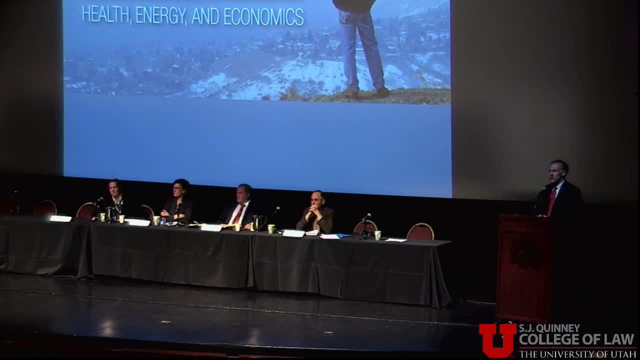 Well, I know there are some who have been arguing that, not even requiring or waiting for Congress to act, that EPA should include, as one of the state options, a carbon tax, not just cap and trade, And I think the issues are very complex. 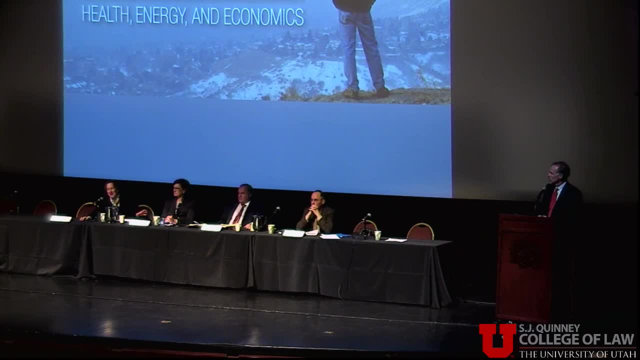 And actually I'm not going to— I'm not going to try to answer them because you know we still have to come back to the statutory language of the best system of emission reduction. EPA has already stretched that a fair amount in doing some very innovative things. 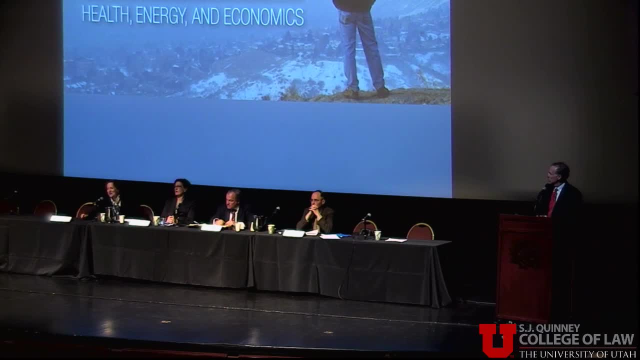 And I think that the stretching just becomes even a little more elastic once we start thinking about a tax. I mean, one of the critical issues with the tax is also that you know it is again linking it to particular mechanisms. I mean, what EPA did in the Clean Power Plan was to say we're going to evaluate actual things. 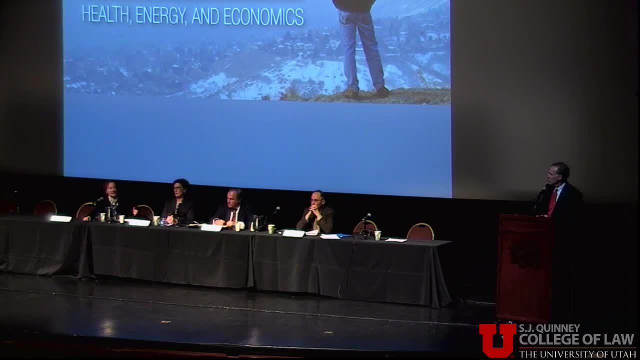 We're going to look at actual things that can be done and then add them up and see what the target looks like, based on actual things being done. That's how you figure out a best system of emission reduction And a tax sort of doesn't have you doing that? 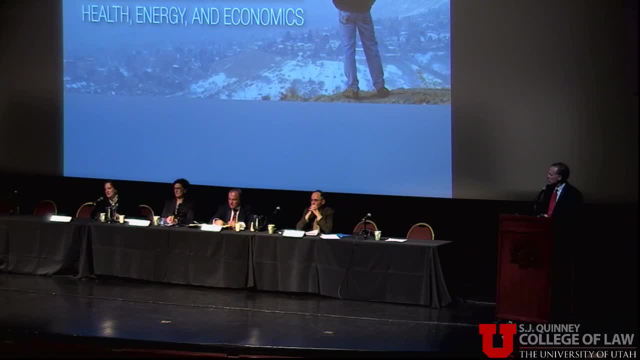 And so it's a very different way of going about setting a standard. that's even more different from the way in which EPA has traditionally set standards than what EPA already did. But again, EPA has been very innovative here, And so I don't want to rule out, and I haven't actually read the analysis. 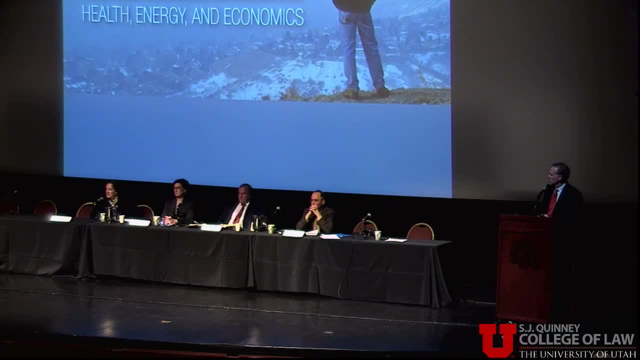 I don't want to rule out the analysis that suggests they should be allowing states to go ahead and do a tax, But somehow it will have to have probably be a cap in tax, not just a flat-out tax, Because I think somewhere in there you're going to have to show you're actually, you know, getting a certain degree of reduction. 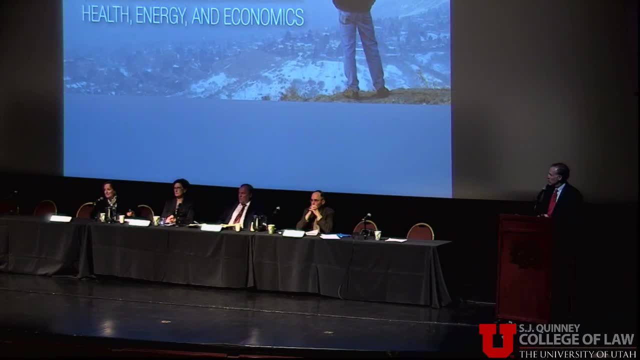 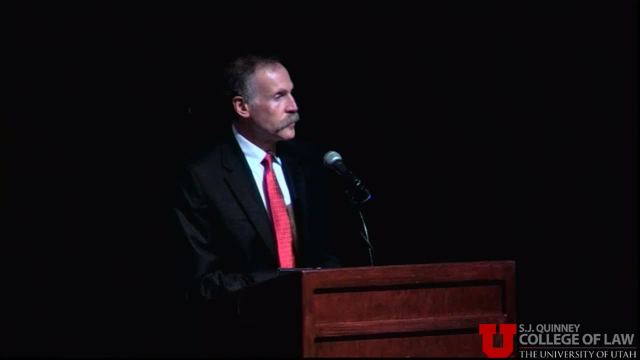 The problem with the tax is you may end up just getting people paying it and not actually getting the reduction, Hans. So I don't want to go into the details, But what I can do is I can see just what we're saying, what that looks like and what's going to go in the future. 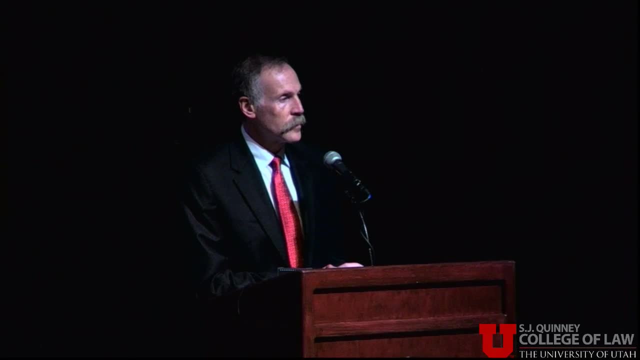 But what I can do is I know what it's going to look like when the tax rate goes up. That's not what I need to do, And that's what I'm trying to do, And what I don't need to do is I'm just trying to say that we're going to go ahead and start weighting the long haul if it's going to go up. 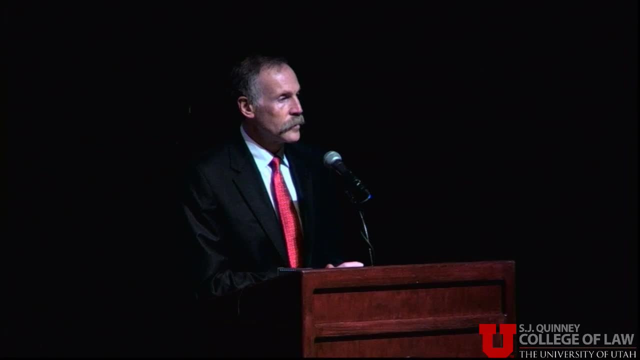 And maybe that's the other thing- that costs a lot of money, just the cost of the tax. I know what it costs. I'm going to have to make that up Like it's not something that's going to go up. It's going to go up. 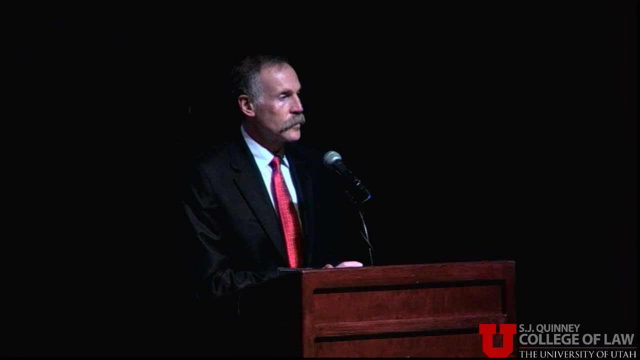 So I'm just trying to make that up. So the question was: some people object to using the Clean Air Act as a misapplication of a pollution statute for climate change. Is there a more direct approach, such as a constitutional amendment or other form of? 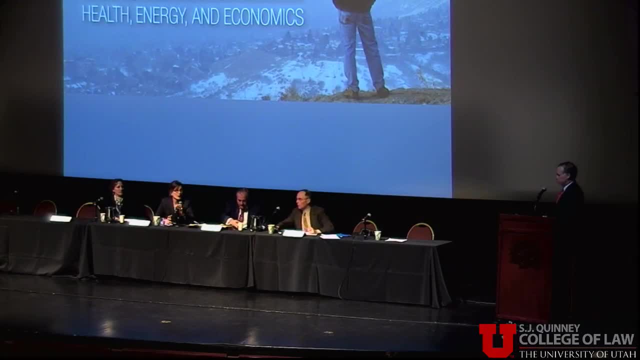 national energy policy. Well, I mean, it seems to me that the train has left the station. in terms of whether the Clean Air Act could be applied to climate change, because the Supreme Court has decided, Is it not close enough? Might not be on. 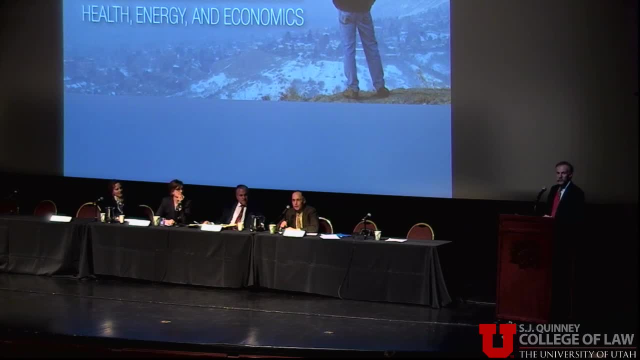 Is this on? Yes, it is Okay. So the Supreme Court has already decided. Now there may still be a question of legitimacy that some people would argue, But anyway, it seems to me we've probably gone beyond that. But if we're going to, if we think that something else besides the Clean Air Act is needed and 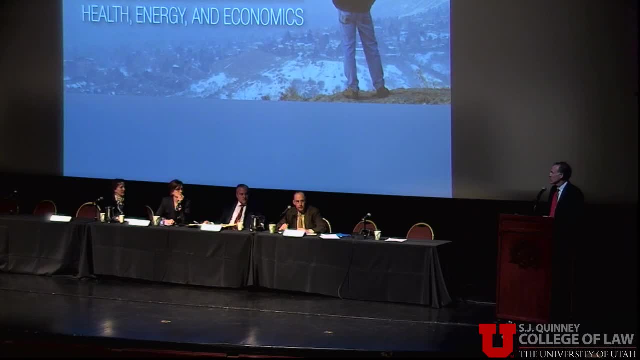 I do think that we'd be better off with something else. I think the logical approach would be a statute. It would be even harder to get a constitutional amendment through, obviously, than a statute. So I think- And our report here suggests the statutory design- 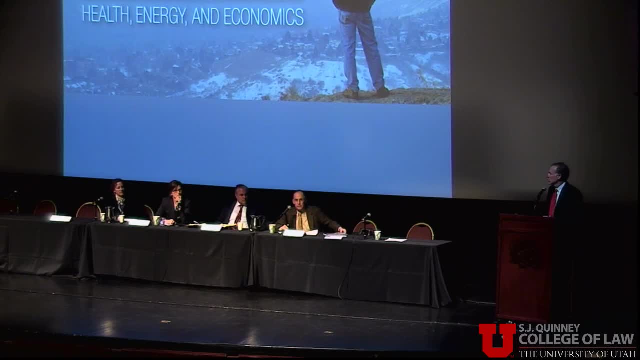 Now one may well say that Congress is not going to act. I mean this Congress, I mean what do you expect it to do? But who expected? Nobody in 1968 expected Congress to pass the Clean Air Act in 1970.. 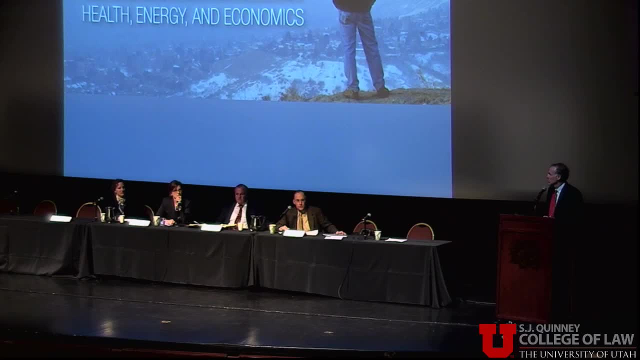 People have to start expressing anger at a system which is not terribly functional. As I've said in my talk and I'll say now, I think EPA has been very clever in trying to use the Clean Air Act, but it really is not terribly well adapted to the job. 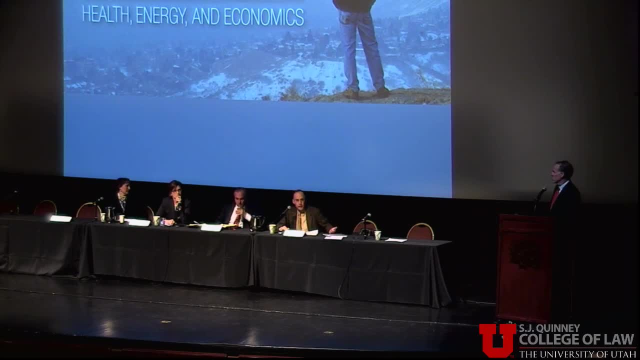 For this reason that we talk about cap and trade or trading emission allowances to take advantage of that latitude to trade and the ability that that gives us to reduce the carbon emissions more economically, forgets the fact that the Clean Air Act throws lots of wrenches. 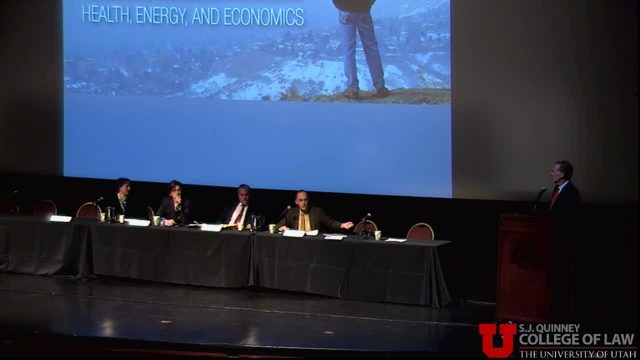 in the machinery that denies us the latitude. So it would be much better if we could get Congress to actually address this thing from scratch. It's not about to do it today, but we've got to get angry for it to happen. I think where we all agree is that it would be useful to have a national energy. 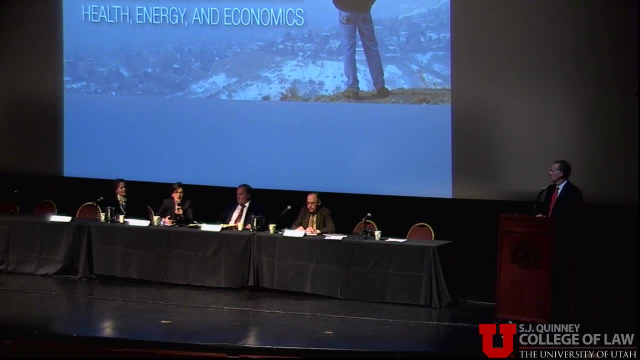 policy that emphasizes carbon and carbon reduction. I think that we tried to get a comprehensive economy-wide Thank you bill passed and it failed. I think that if we sit around and wait, we're losing even more time than you're concerned. we're losing by using the statute. 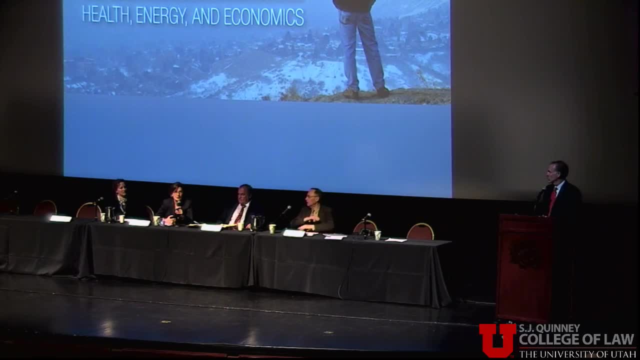 In fact, right now a new source has to have a carbon limit on its emissions, So the act is actually working. Car emissions have to be reduced over time, So we are getting benefits by using the tools we have. My granny used to say a bird in the hand is worth two in the bush. 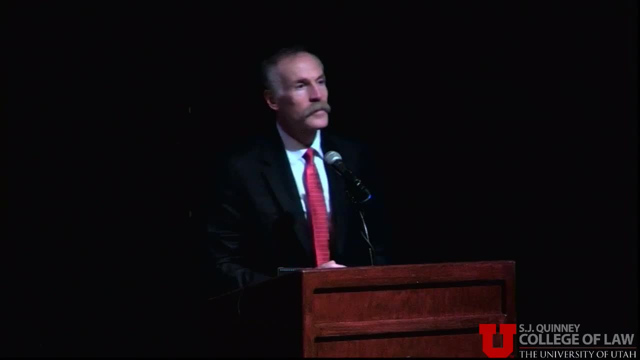 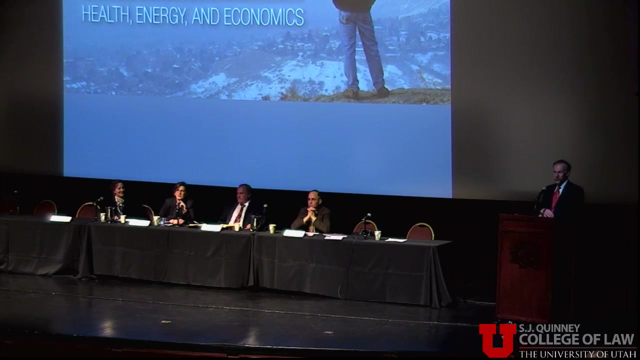 Yes, Thank you. One of the first cases I worked on as a young practicing lawyer was a case under Section 126 of the Clean Air Act, which says that an upwind state is responsible for controlling its emissions, so that a downwind state doesn't go out of attainment or isn't in violation of the air quality standard. 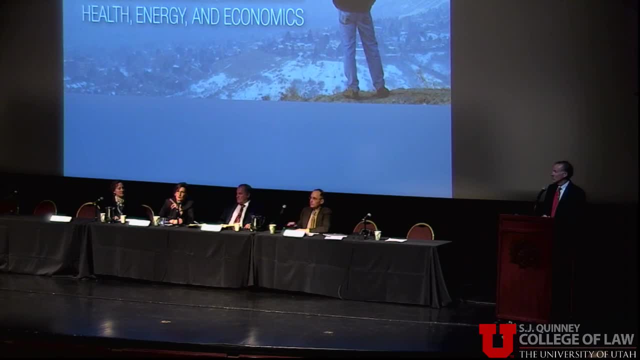 And there are two approaches. One is the federal government can pull state implementation plans and say these are not adequate, and here's what you'd have to do to make it better. Or a state can sue an upwind state under 126.. 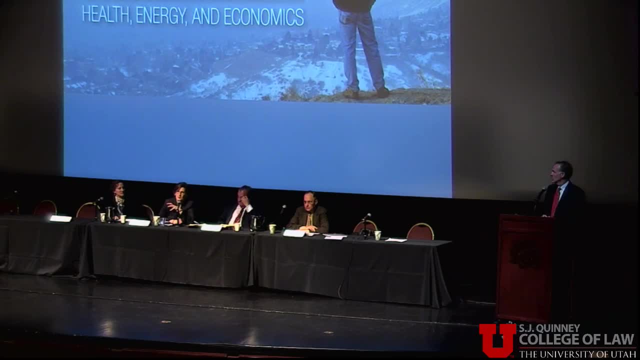 The first one is under a different section- has to do with the adequacy of state plans. EPA has been doing this in the eastern half of the United States with respect to ozone And in fact the Supreme Court last year had it. It got the case evaluating. its most recent attempt called the cross-state air pollution rule to quantify and to direct states on what they needed to do, what the upwind states needed to do to control the downwind states' pollution. 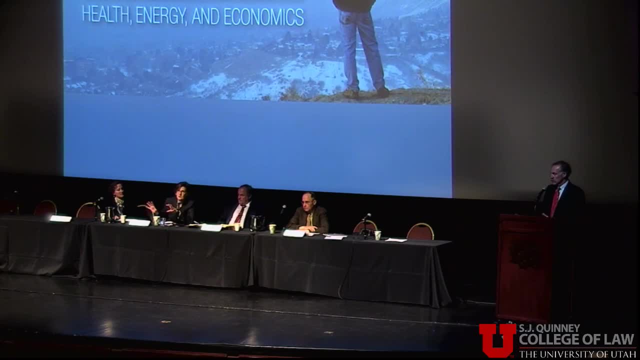 That is the eastern half and it has to do with smog. But those tools are certainly available elsewhere. if there are demonstrated mechanisms whereby states State A downwind- is being harmed by upwind state A's air pollution, I would add that, yes, I would agree that the mechanisms do exist in the act, but they are fraught with delay and awkward to use, so we don't get as much good out of them as we need.